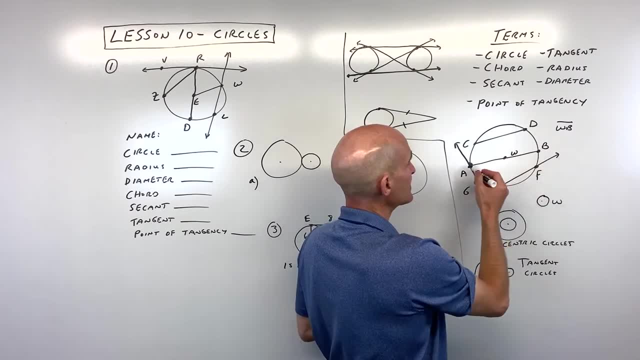 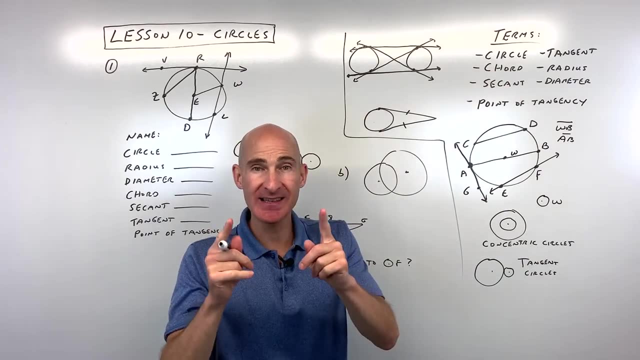 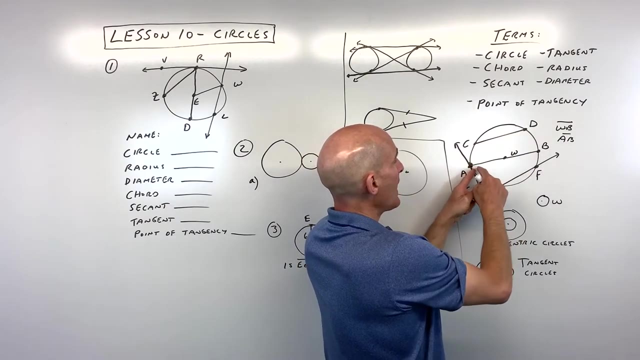 that segment lie on the circle, and in this case the diameter here would be segment ab. Okay, now let's go over here to a chord. so when we talk about a chord it's a line segment, such that the end points of the line segment lie on the circle. So for example, cd is a chord ab we. 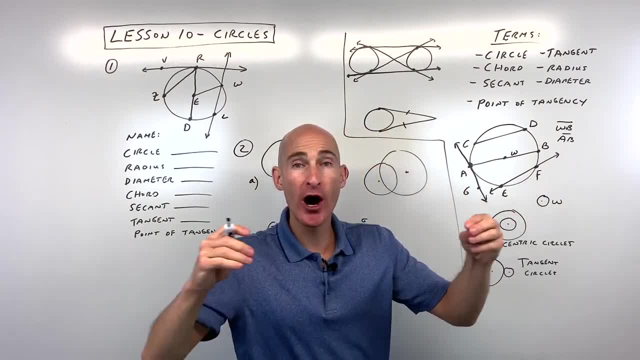 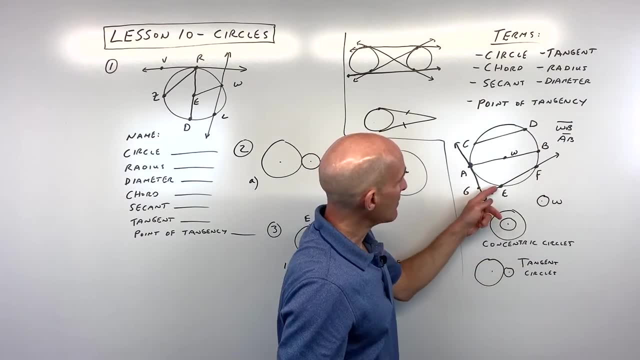 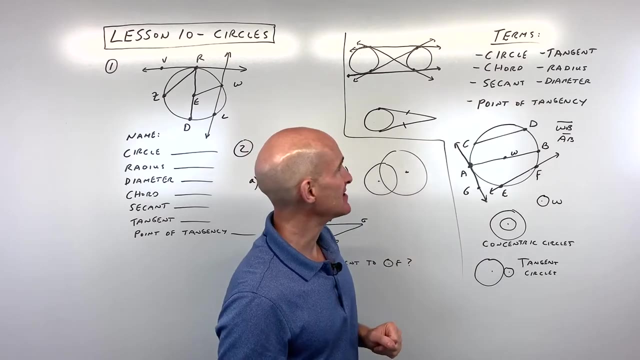 said is a diameter, but it's also a chord. it just happens to be the longest chord in the circle. So also here you could say segment ef is a chord. Now, if you talk about line ef, see how it keeps going. it cuts through the circle at two points. that's what we refer to as a secant okay s-e-c-a-n-t. and. 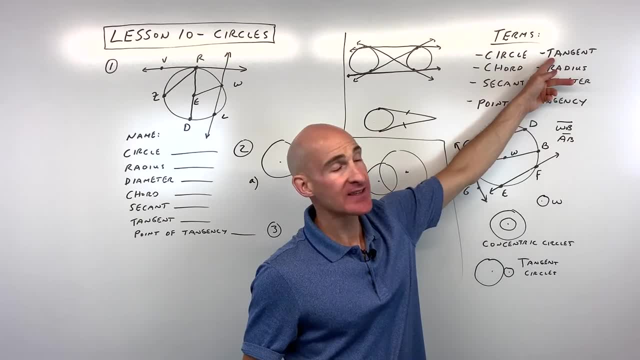 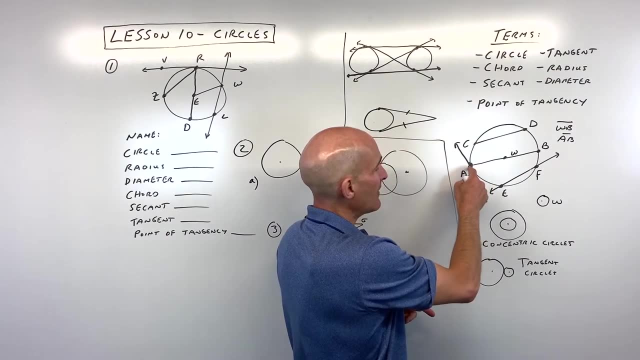 then a tangent is a line or a line segment such that it touches the circle just at one point. So it just barely touches the circle, just kind of barely scrapes it, and this point where it touches that circle we call the point of tangency. So in this case the point of tangency would be a. 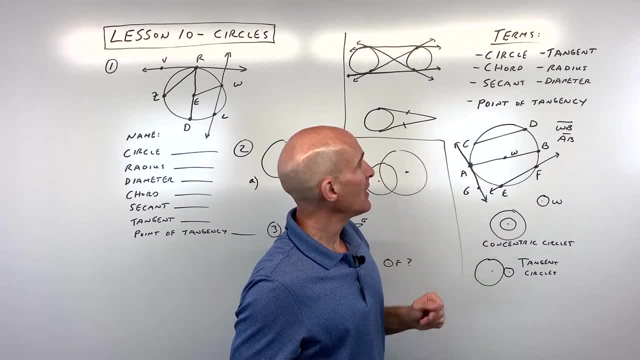 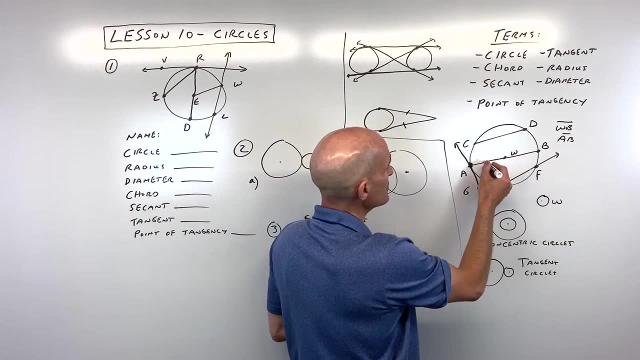 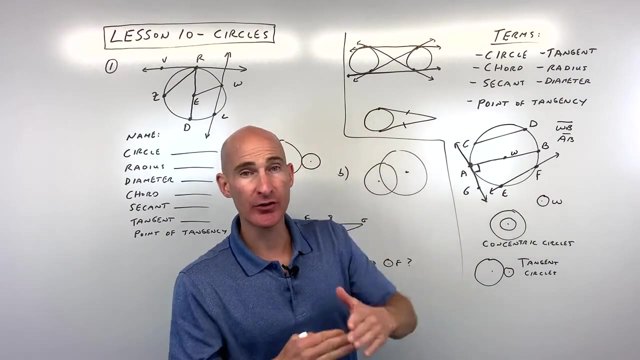 the tangent line would be line ag. And the other thing we want to talk about is when you have a circle and you draw a radius, okay, to a line that's tangent to the circle, like this, it's always going to form a right angle, a 90 degree angle. it's going to be perpendicular, It's. 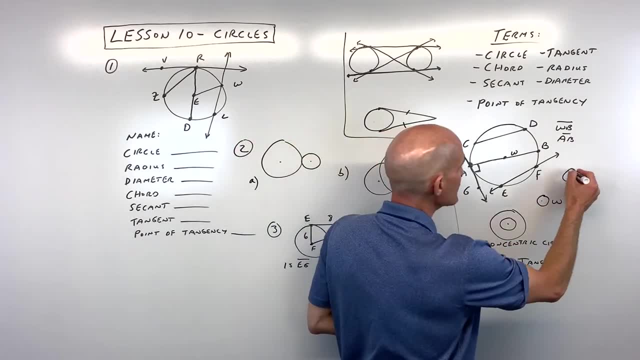 kind of like if you're riding a bicycle, kind of visualize: here's your bike right and this is the ground right, one of those spokes. okay, if you go perpendicular, or I should say if you go right to the point where it touches the ground here with the edge of the tire, that's going to form a right. 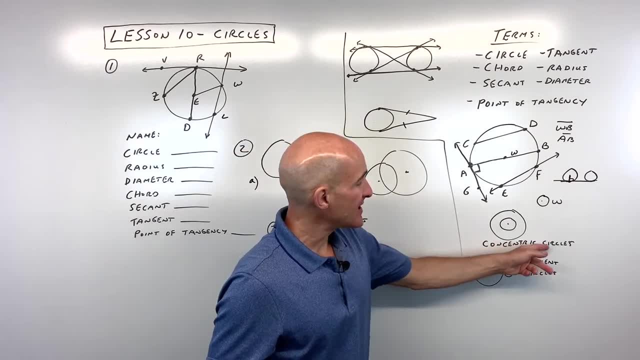 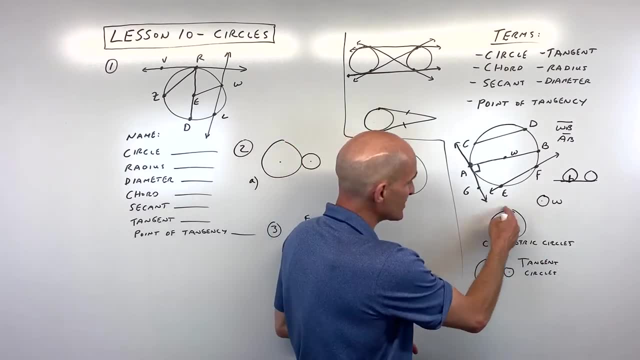 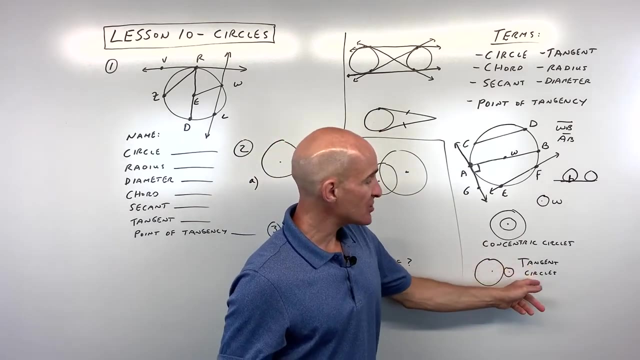 angle, a 90 degree angle, So you can have two circles. C-o-n means like width, the same center. so here you can see, you have like a circle inside of a larger circle, but they both have that same circle. it's kind of like a bullseye. so that's an important term. concentric circles, Tangent circles we talked about when, like 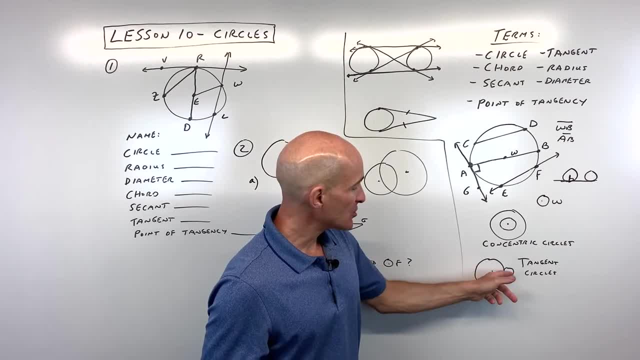 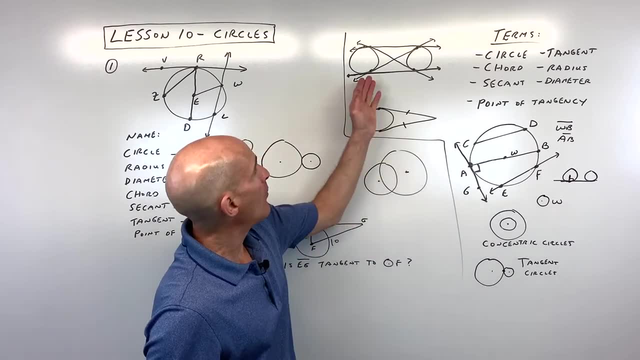 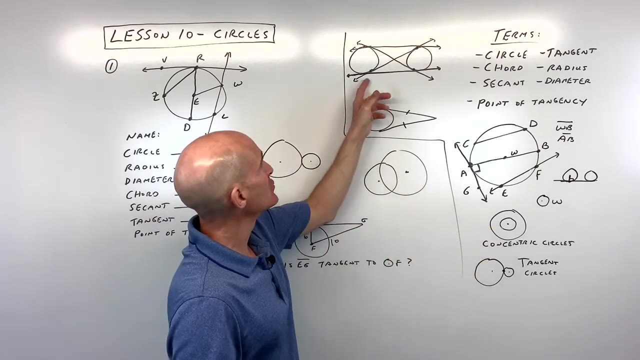 a line is tangent to the circle, it just touches it at that one point. but you can have circles that are tangent to one another, where the circles are just barely touching at one point, like that. Now, when you have two circles, you have a tangent that's in common to both circles. so, for example, if we look at this line, 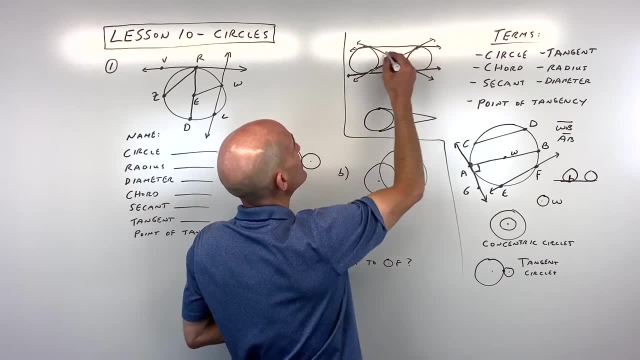 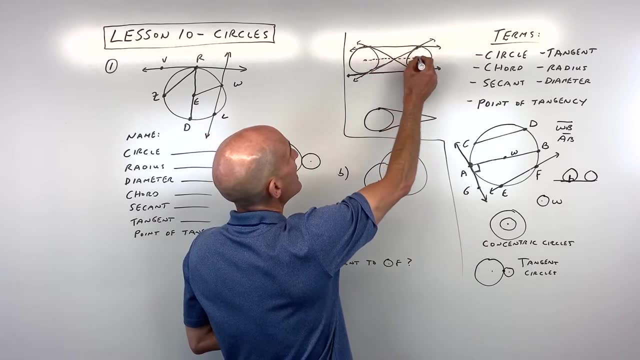 right here. this is what we call a common internal tangent, and you can see it's going in between the two circles. Another way to look at it is if you were to draw like a dashed or dotted line between the two center points of the circles. if it's an internal tangent, it's going to cross that. 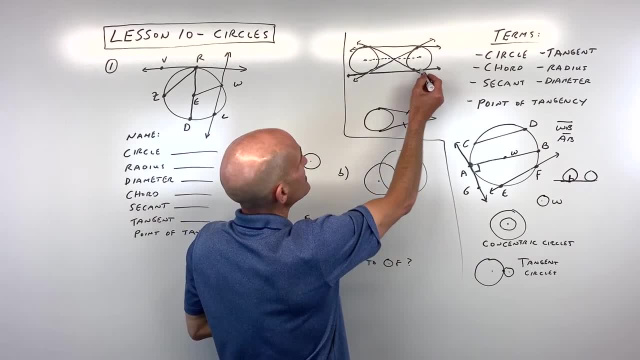 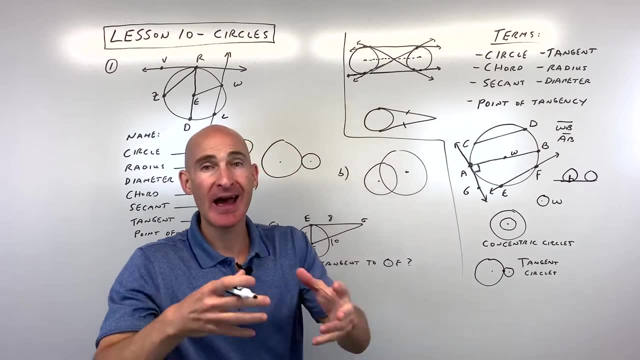 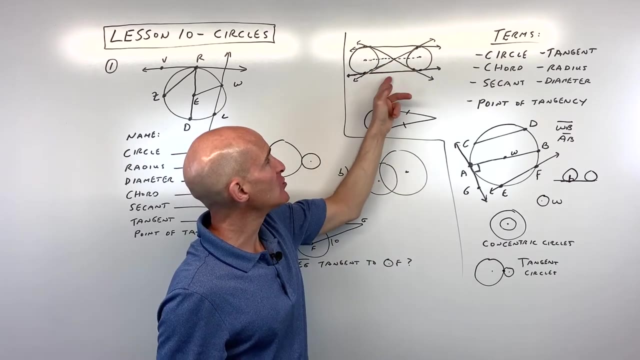 center line, whereas if it's a common external tangent, see how it's just barely touching both these circles at these two points, but it doesn't cross that center line. this is what we call a common external tangent. so it's common to both circles. it's just that it's external. so in this case we had two internal and we had two external. 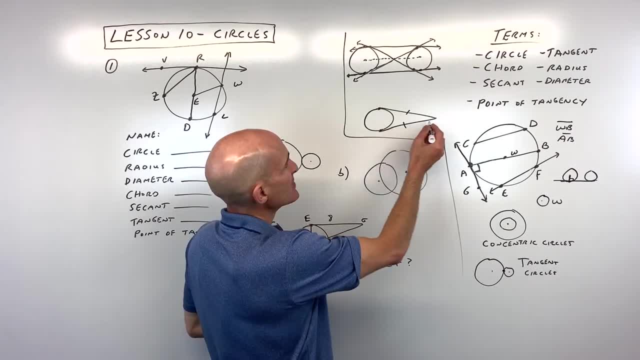 tangents. and then the last thing I want to show you here, before we dive into some examples, is: say, you have a point outside a circle. you could draw a tangent such that it goes just barely above the circle, just barely below the circle. but these two tangent segment lengths are going to be 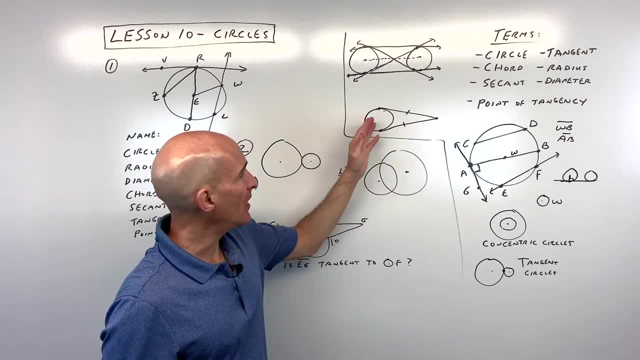 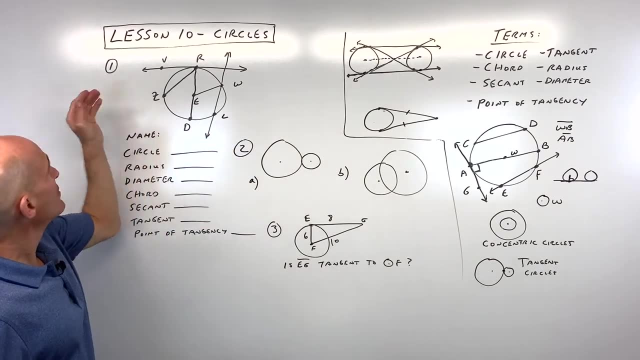 congruent, okay, and you can prove that usually using the congruent triangle theorem we talked about earlier in the course. but let's try some examples so you can see how this works. so let's look at number one. so what we want to do for number one is we want to name the circle, the radius, the diameter of the chord, the secant, the tangent and 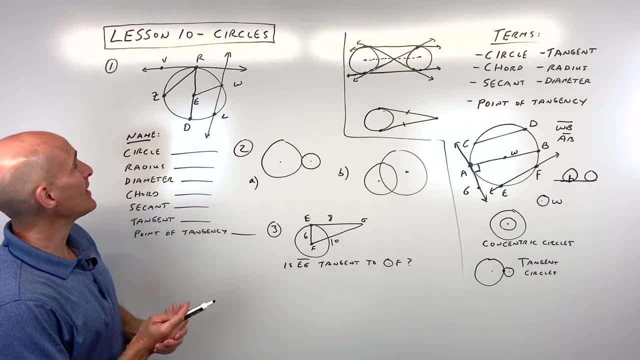 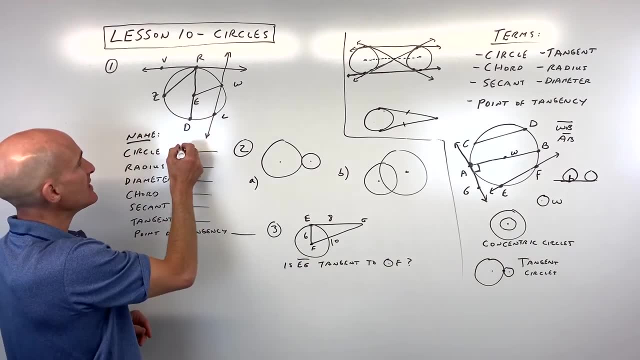 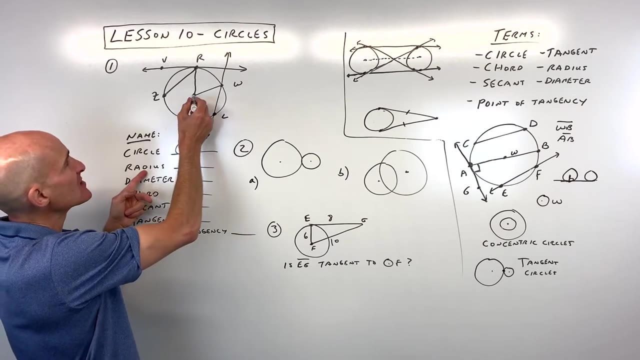 the point of tangency in this diagram. so how would you name this circle right here? well, the important thing is the center of the circle. you can see, the center is e, so we're going to label it circle e. how about a radius? well, remember, the radius is the distance from the center of the circle to a point on the circle. so 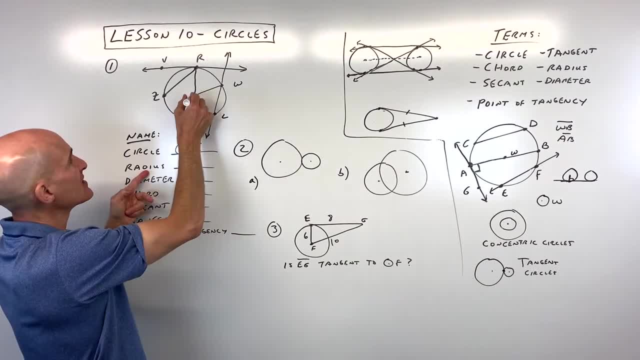 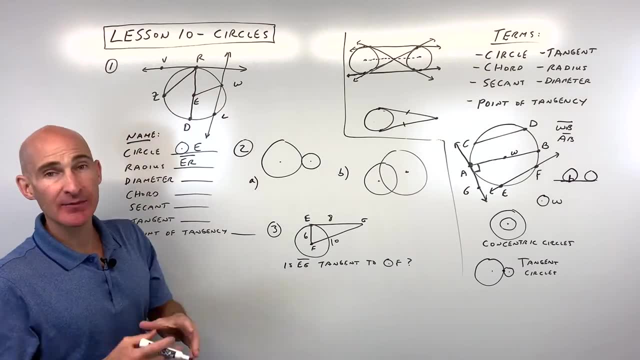 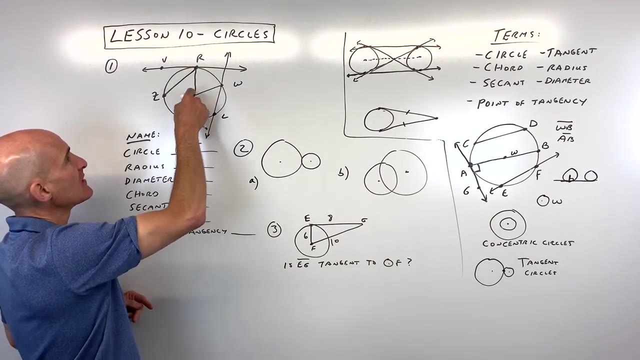 we could say segment er. that's one option. we could say segment ed, segment ew. there's more than one radius here, but all these radii will have the same length. how about a diameter? diameter, remember, it's a segment, such that the end points lie on the circle and it goes through the center of the 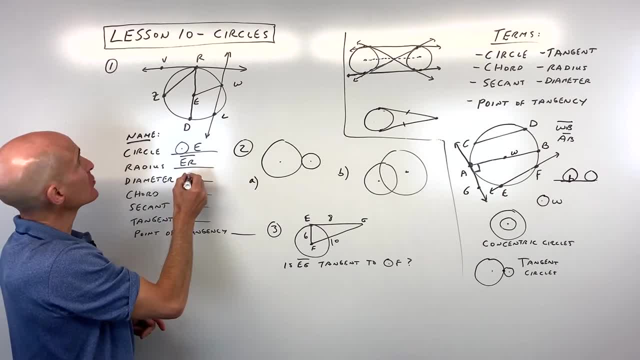 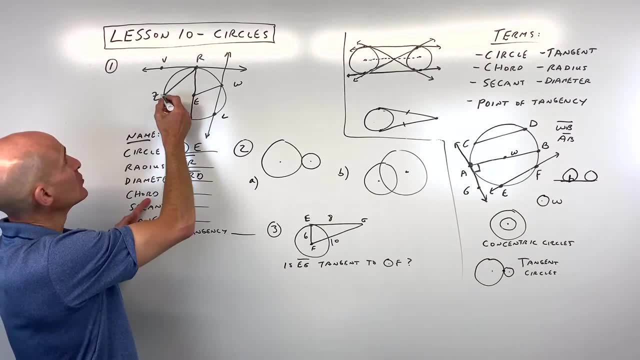 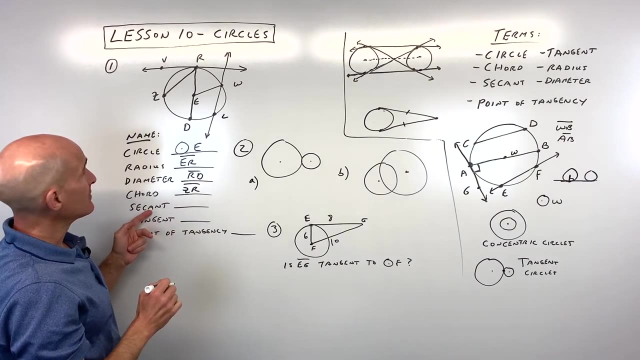 circle. it's a chord. it's the longest chord in the circle. in this case it's going to be segment rd or you could say dr. either order and let's see a chord. we could do like zr, remember, a chord is a segment with the end points on the circle. let's see a secant. secant is actually a line. it keeps. 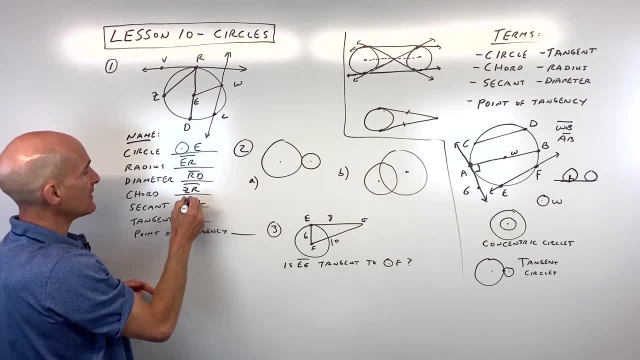 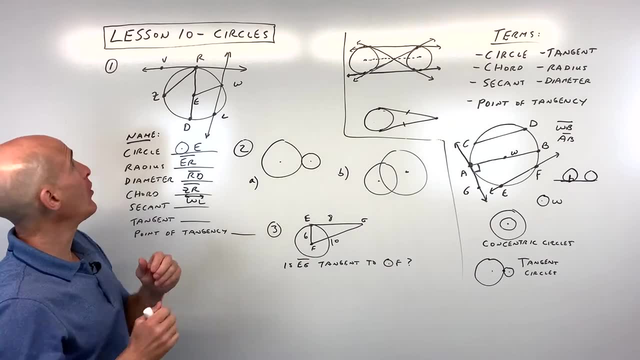 going and it cuts through the circle at two points. so here I would say line w or lw and a tangent: okay, a tangent, we know. it just barely touches a circle at one point. so here we can say like line vr: okay, And then the point of tangency. 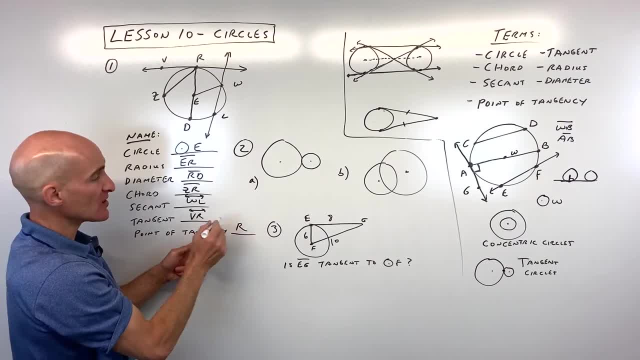 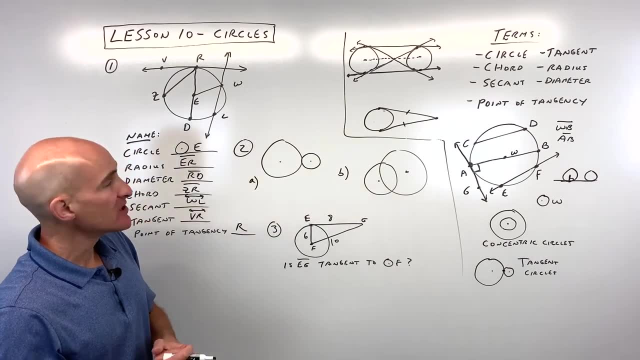 where does it touch the circle? at just one point. That's gonna be point R, So we use a capital letter for points. Okay, for number two, we've got two parts, A and B. What I want you to do here is: 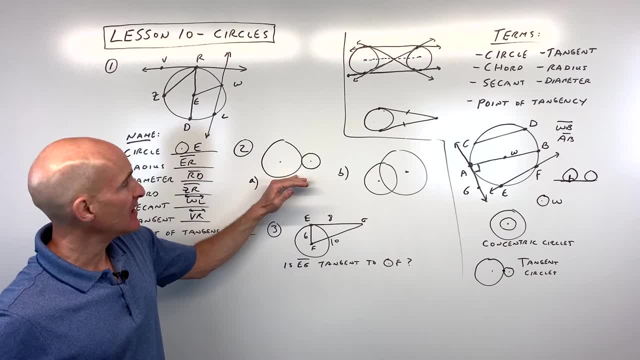 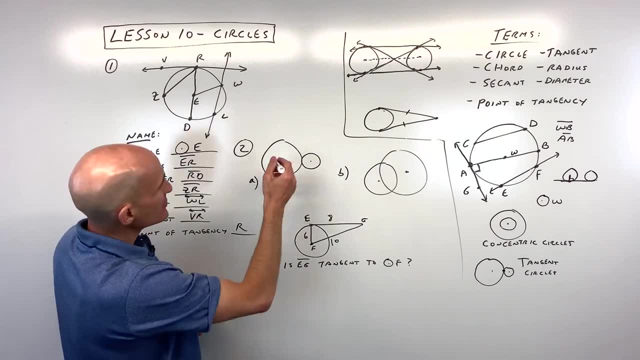 how many common tangents do you see in this diagram, And are they internal tangents or are they external tangents? Well, let's see Here. it looks like we could draw a common external tangent like that. Okay, so that's one. 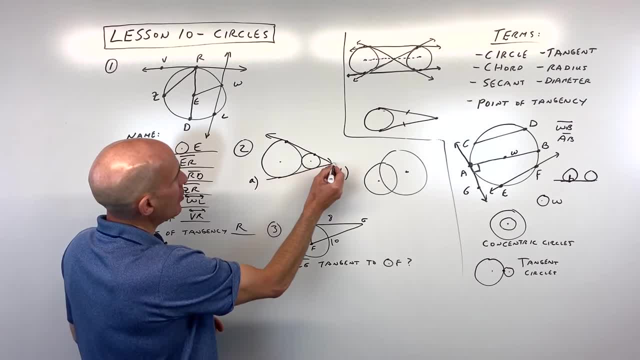 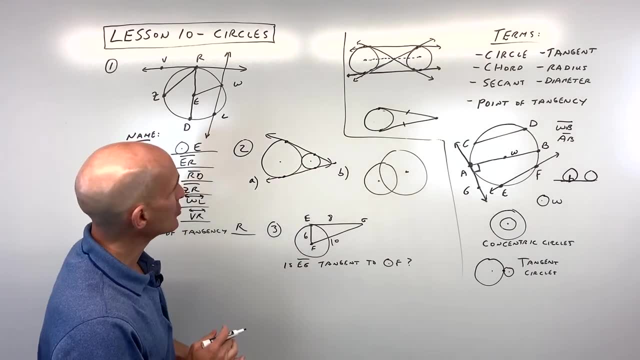 Any others We could draw, maybe like this right below: Okay, so it touches just at these two points. So we've got two common external tangents. How about internal? like in between, It has to cross this imaginary line that connects the two centers. 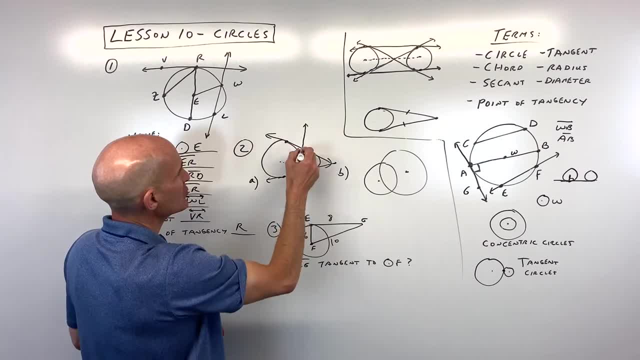 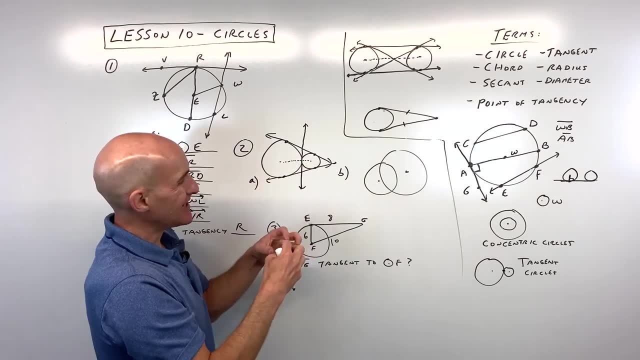 Well, in this case we could go like this, where it just goes right between the two circles. That would be one common internal tangent. And you can see that the circles are tangent to one another. They just touch at one point, right there. 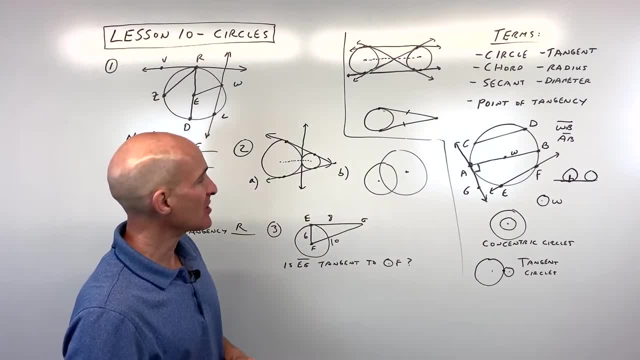 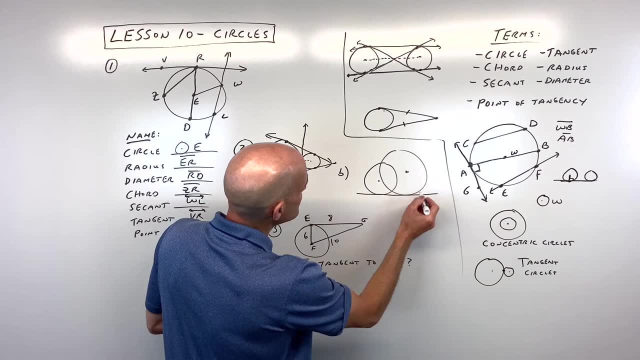 Okay, how about for letter B? What do you think? How many common tangents are there, And are they internal or are they external? Well, let's see. In this case, we could draw one like this: Just barely touches here. 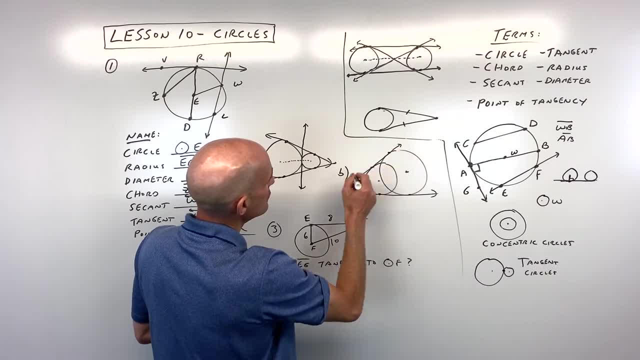 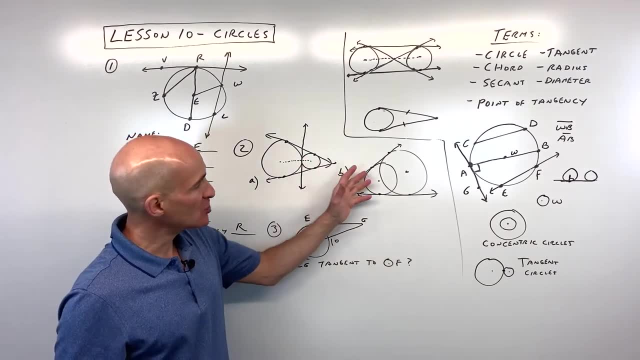 We could draw one like. this Just barely touches at these two points. Can we do any internal ones in between? Doesn't look like it because of the way the circles are overlapping, So it just looks like two common external tangents. Okay, how about for number three? 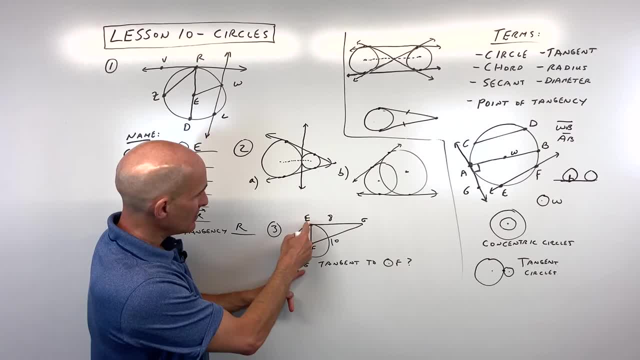 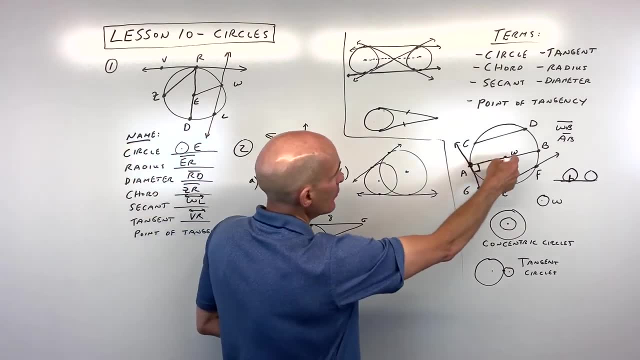 Now number three. this is a little bit different. It says is segment EG, right here, tangent to circle F. Well, remember when we talked about when you have a tangent and you draw like a radius from the center to that point of tangency. 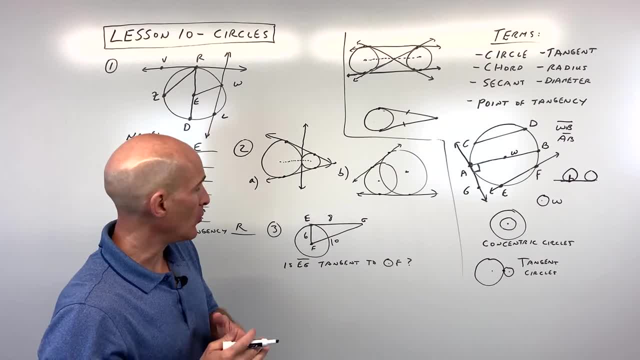 it's always gonna form a perpendicular. you know a 90 degree angle, a right angle. So the only way that this would be tangent is if this is a right angle. Well, how do we know if this is a right angle? 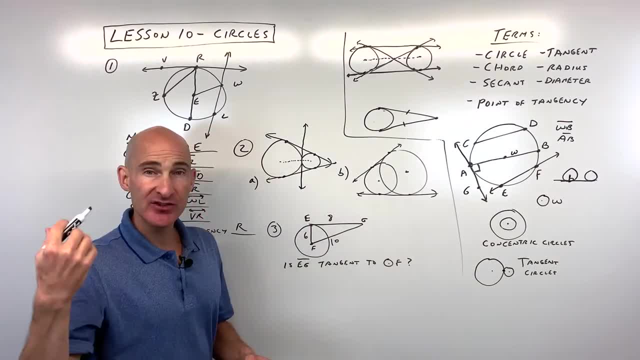 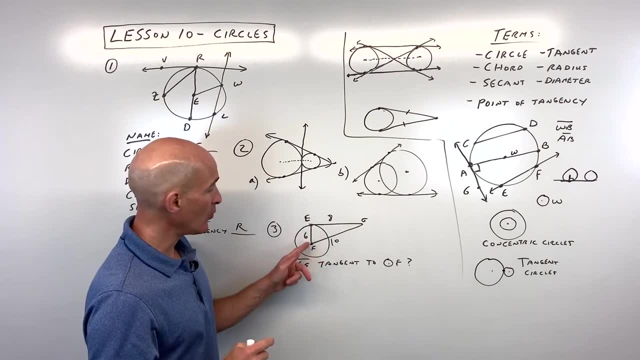 Well, we talked about this in a previous lesson about the converse of the Pythagorean theorem. If A squared plus B squared equals C squared, then we know this is a right triangle. This is a 90 degree angle, which means then that EG would be perpendicular to FE. 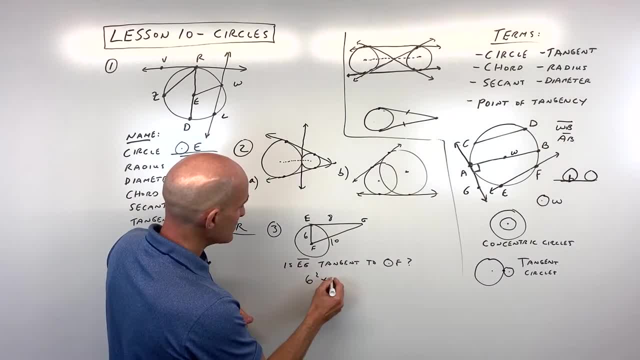 So let's test that out. Is A squared plus B squared equal to C squared? Six squared is 36.. Eight squared is 64.. 10 squared is 100.. So it looks like: yes, this adds up to 100.. 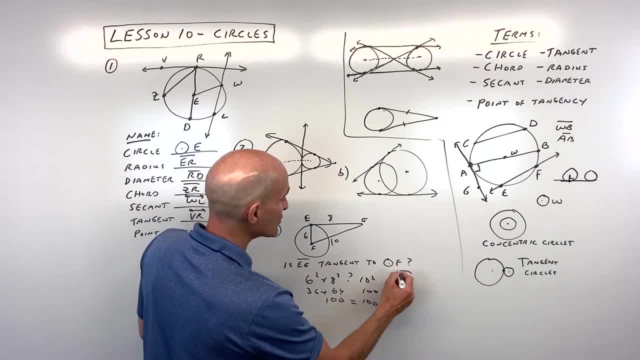 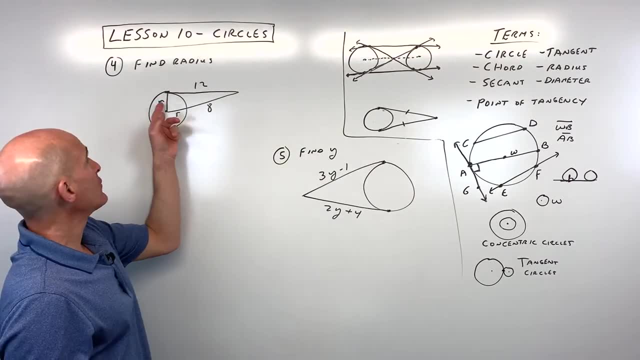 100 is equal to 100. So, yes, this is actually tangent to the circle, So it's touching just at that one point, at that right angle. Okay, for number four. we wanna find the radius of this circle. Now, remember, in this particular example, 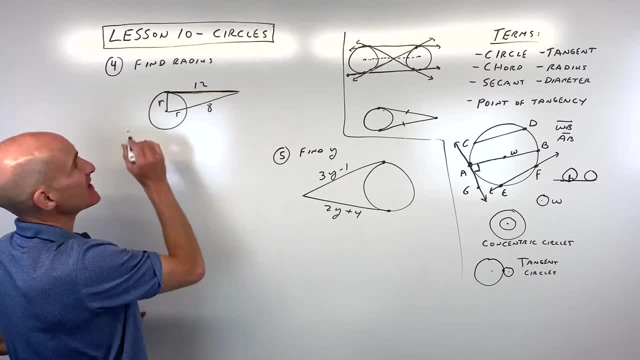 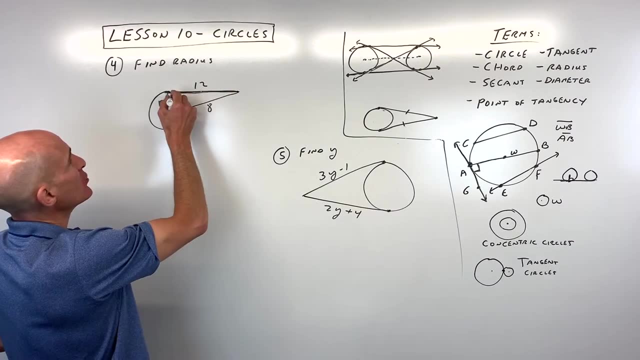 we're gonna assume they're gonna tell us. I'll just tell you that this is actually a tangent to the circle, this 12 length here in this segment. So if we know it's tangent, then we know that this is a right angle. 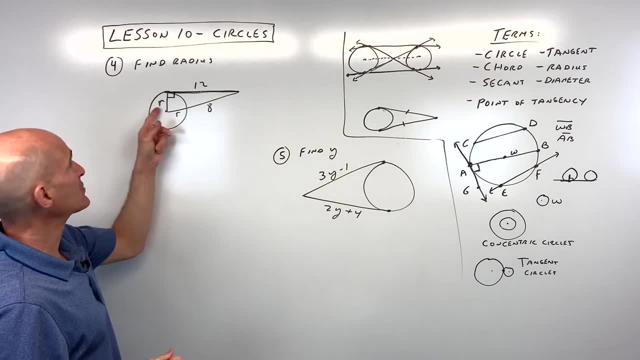 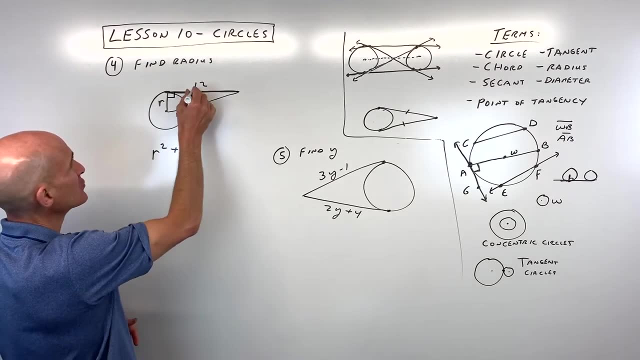 and we know, if we have a right triangle, that the Pythagorean theorem holds: A squared plus B squared equals C squared. So let's go ahead and do that. So we have R squared plus 12 squared equals this whole quantity, R plus eight. 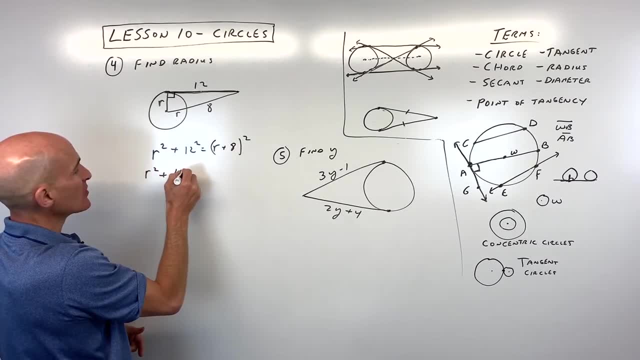 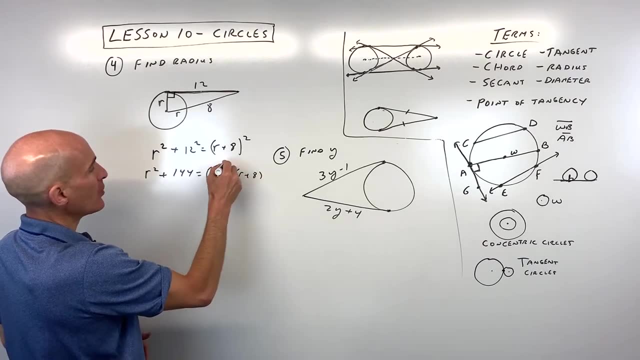 the quantity squared right. So this is R squared 12. squared is 12 times 12.. R plus eight squared is really like R plus eight times another R plus eight and you can FOIL or you can do the distributive property twice. 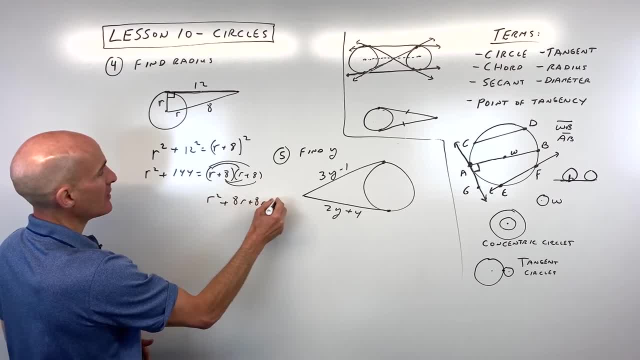 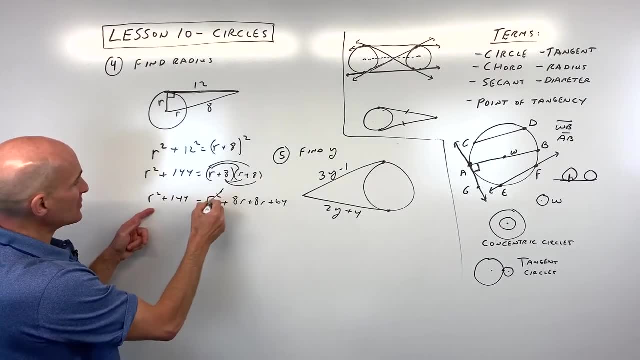 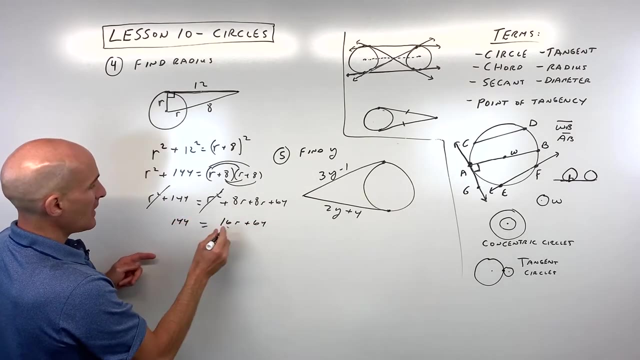 So that gives us R squared plus eight, R plus eight, R plus 64. And if we subtract R squared from both sides, these are gonna cancel And let's see, this comes out to 16 R plus 64.. If we subtract 64 from both sides, 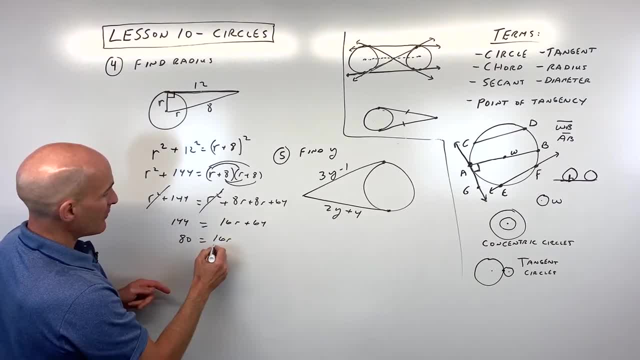 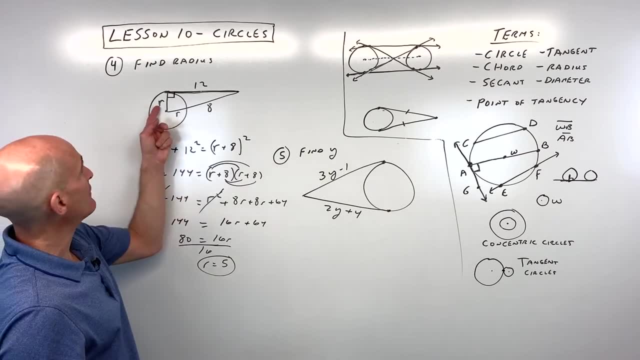 this comes out to 80. And if we divide both sides by 16,, R is equal to five, And you can check your work. if you put it back in, this would be five, this would be 13, and this would be 12, and that you can see. 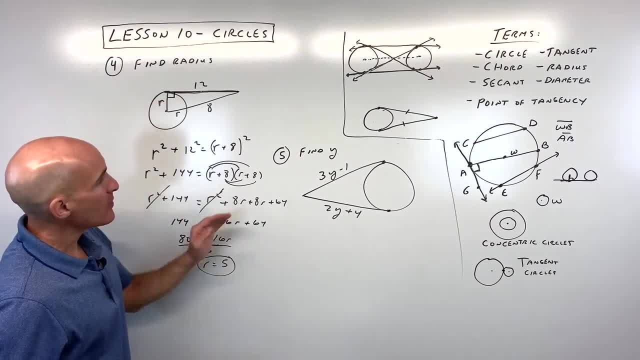 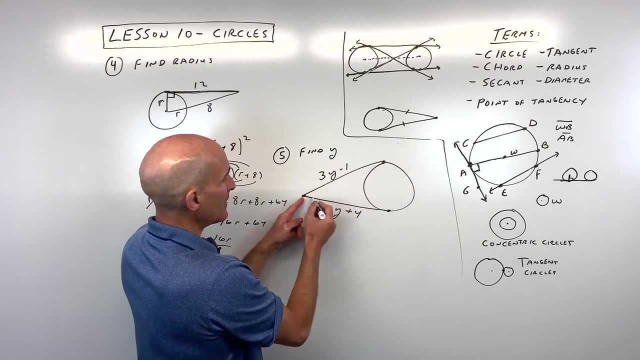 that's a Pythagorean triple five: 12, 13.. Okay for number five. now it says find Y. Okay, so you can see, here we have a point outside the circle and we're drawing a tangent above and below the circle. 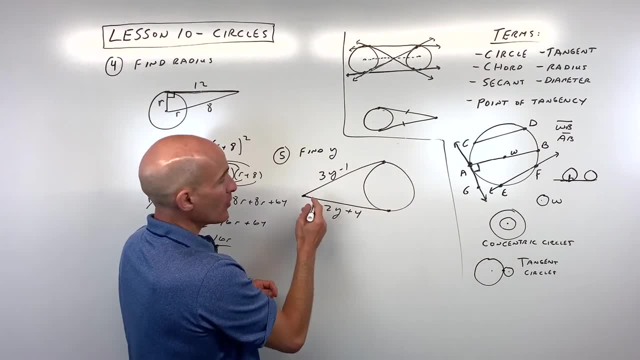 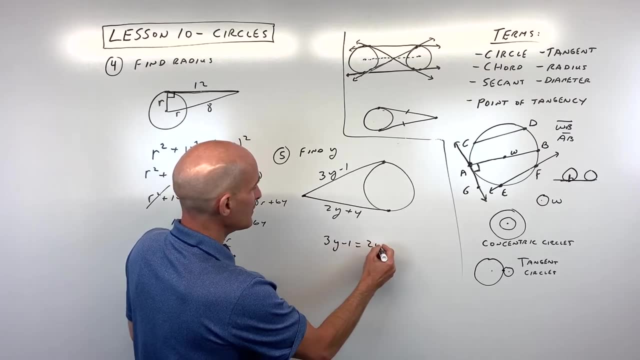 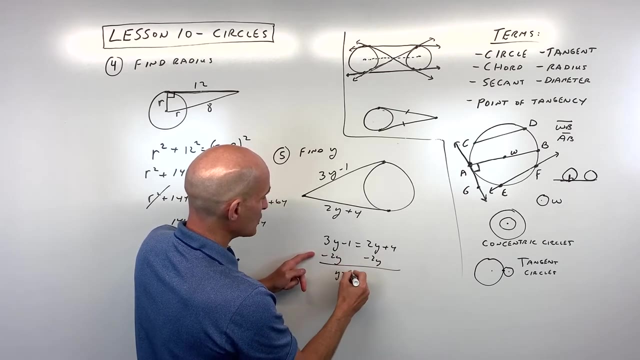 It just barely touches that one point. Well, we know that these two tangent lengths are gonna be equal to one another, So this is gonna be three Y minus one equals two Y plus four. If we subtract two Y from both sides, we get Y minus one equals four. 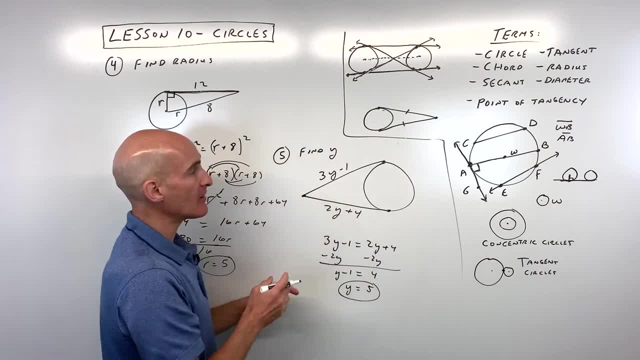 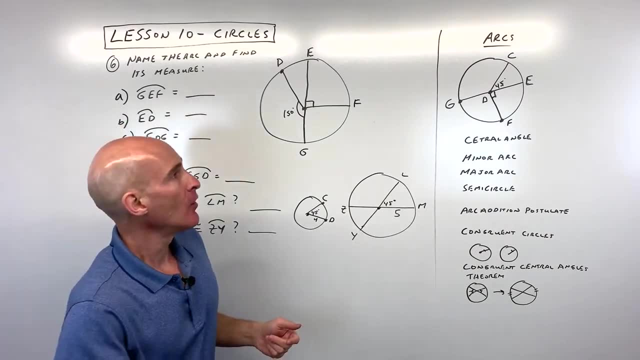 And if we add one to both sides, you can see that Y is equal to five, And you can double check your work by putting it back in. Okay, now let's switch gears and talk about arcs. So what exactly is an arc? 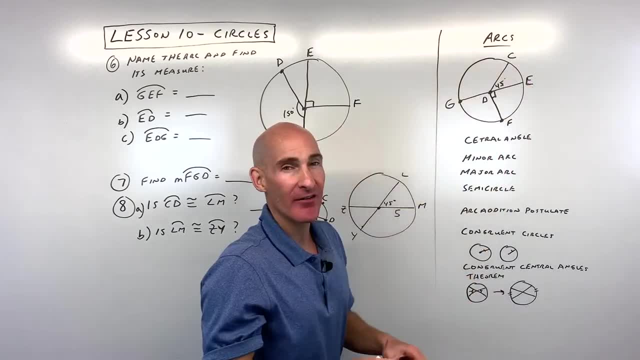 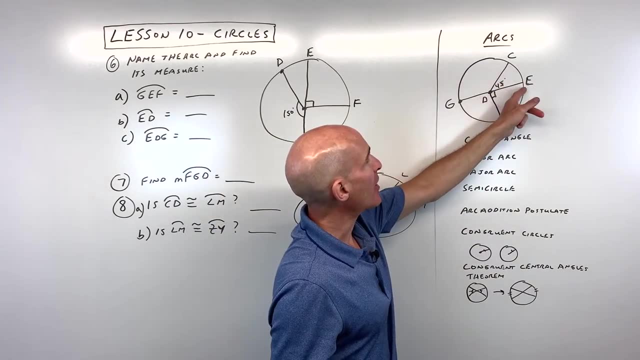 Well, an arc is like a curved portion of the circle, So it's kind of like a line segment, but it's been, you know, been bent right. So the two end points of the arc lie on the circle and they connect that portion of the circle. 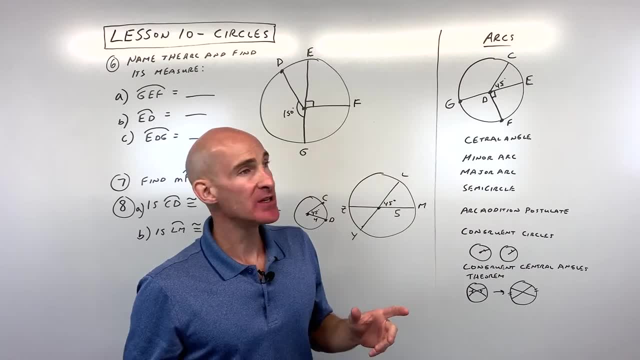 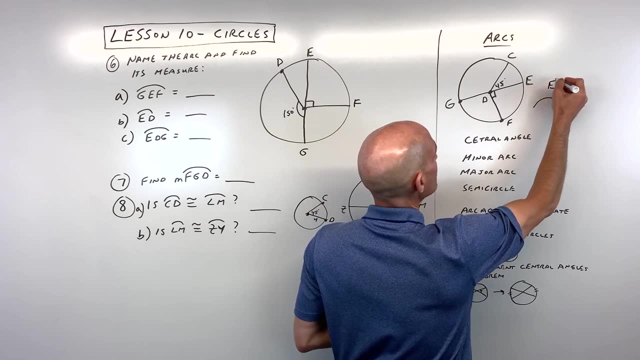 Now, when you label an arc, what you wanna do is you want to use this arc symbol. okay, remember when we labeled segments like, say, if I had segment EL, for example, if I put a line above it like that, like a bar above it. 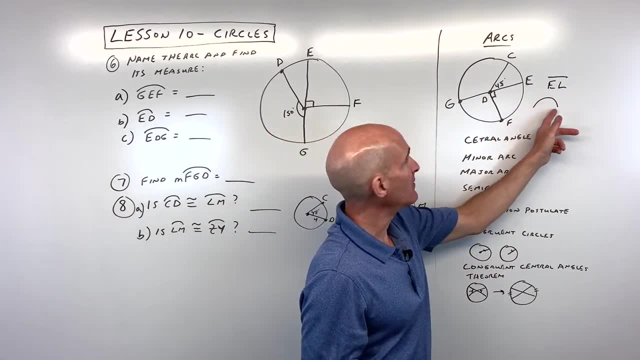 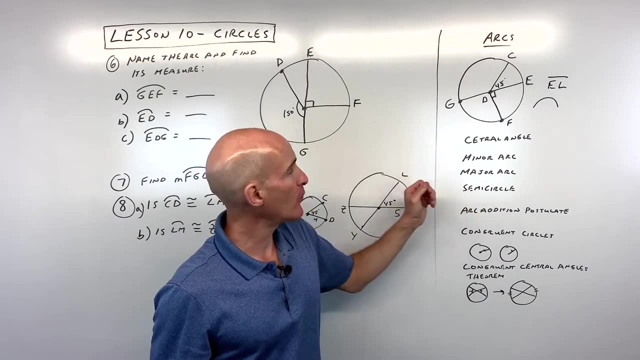 that tells me it's a segment. If I put like this arc above it, then I know it's an arc. But what we wanna talk about first is the minor arcs: major arcs and semi circles. But before we do that let's talk about central angles. 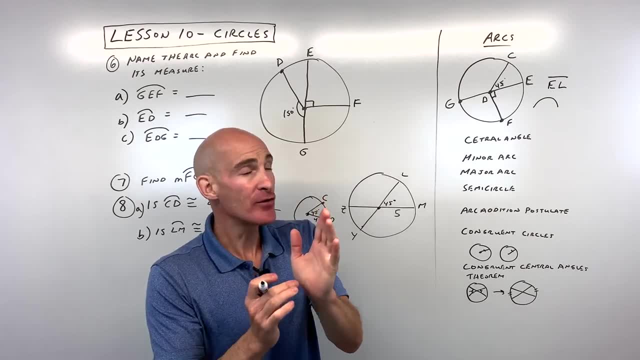 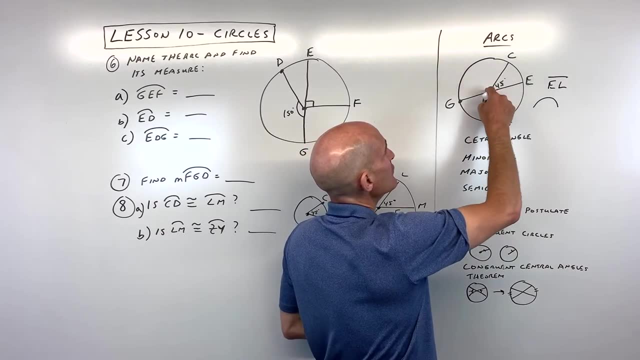 What a central angle is? it's an angle right Where the vertex is. it's gonna be at the center of the circle. So, for example, here we've got the center of the circle. here is at D And if you look at this angle, CDE. that's a central angle. 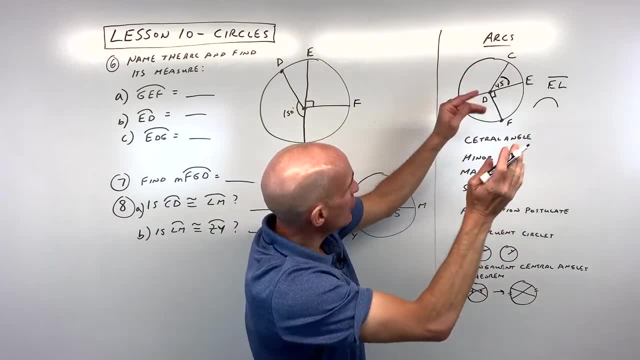 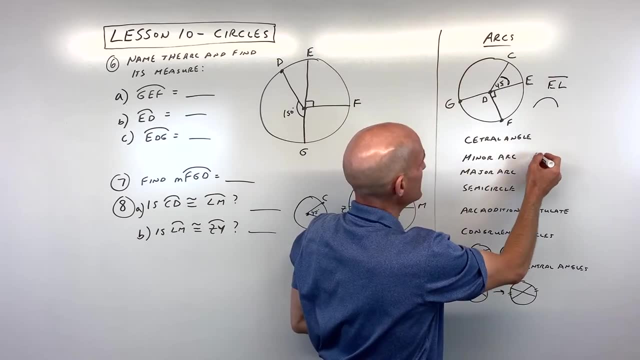 In this case it's 45 degrees. The part of the circle that it intercepts or cuts off, you know the angle, cuts off this part of the circle. that's arc CE, like that, And we call this a minor arc. 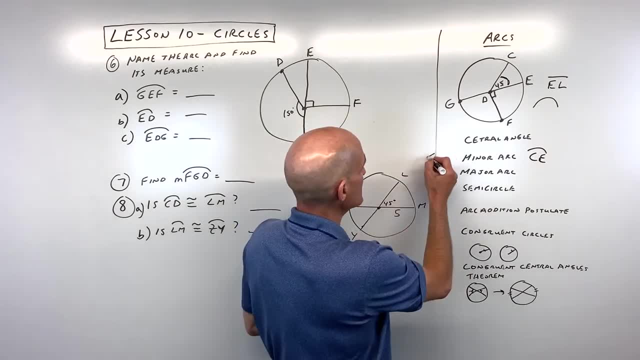 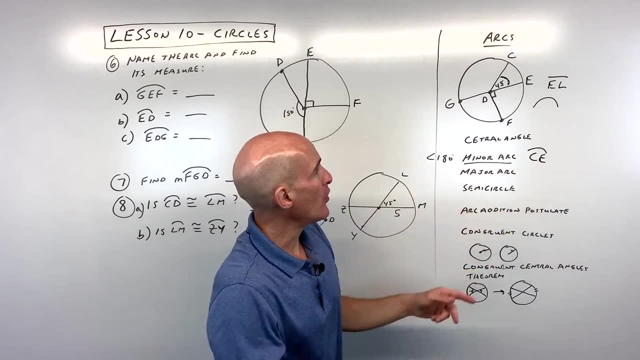 Minor is whenever it's less than 180 degrees. So less than 180 is minor, And if it's a minor you just use two letters, It's just two end points. So this way, if I say CE, you know to go this distance here. 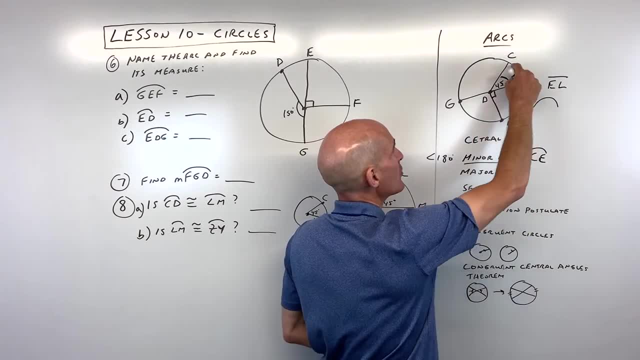 You don't go all the way around like that and say, oh, this is my arc, No, it's the shorter distance from C to E. When it's a major arc, though, you're gonna need to use three points, okay. 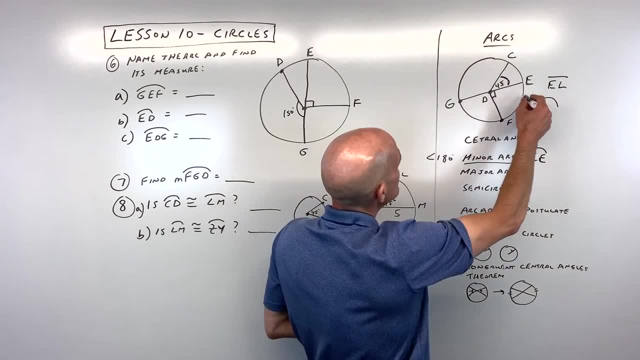 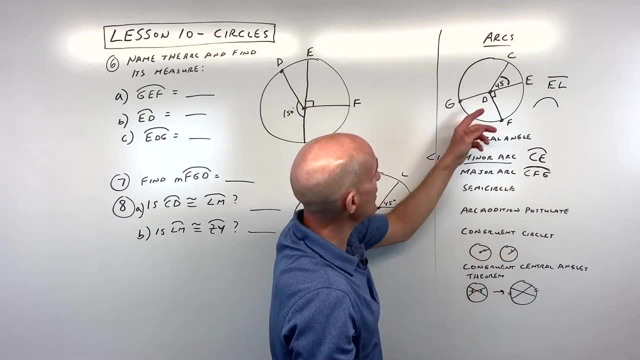 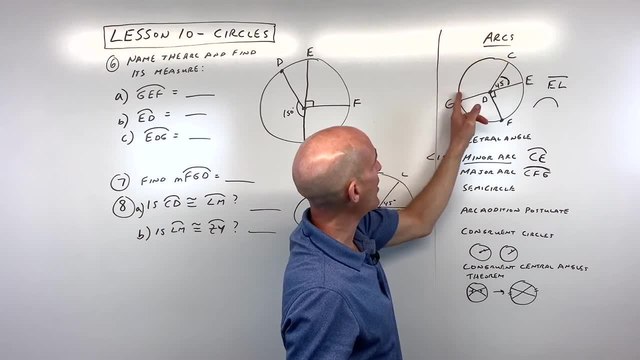 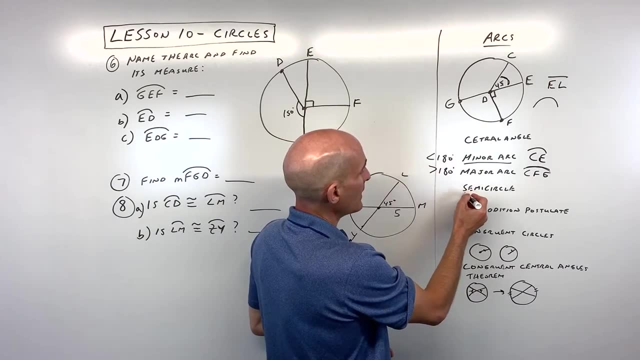 And you can't just say like CG, Somebody would think I'm talking about this arc, not this arc. So that's why we use three points when it's more than 180.. And then when it's exactly 180, that's called a semicircle, like half a circle. 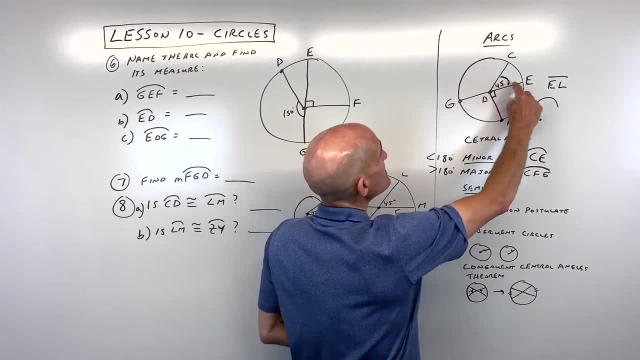 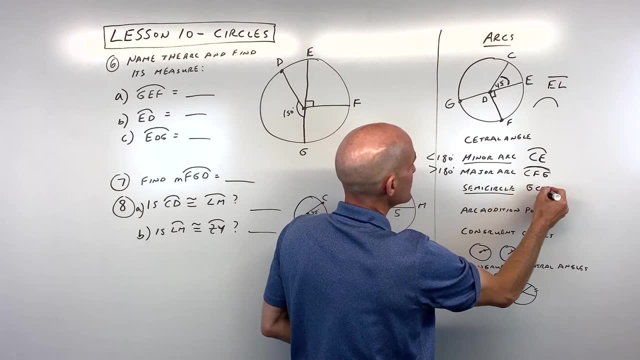 Again, you want to use three points Like here. you can see this goes: This is a diameter here, GE. So I could either do semicircle GCE- let's talk about that one- or I could do a semicircle GFE. 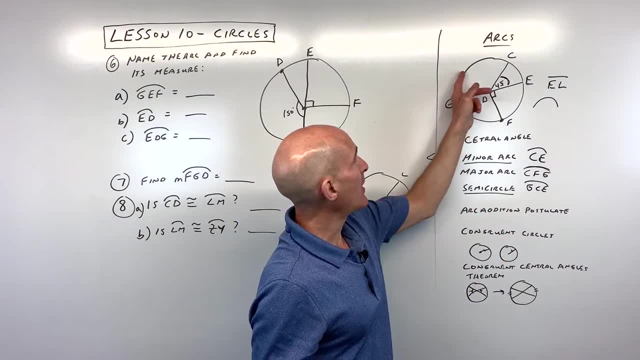 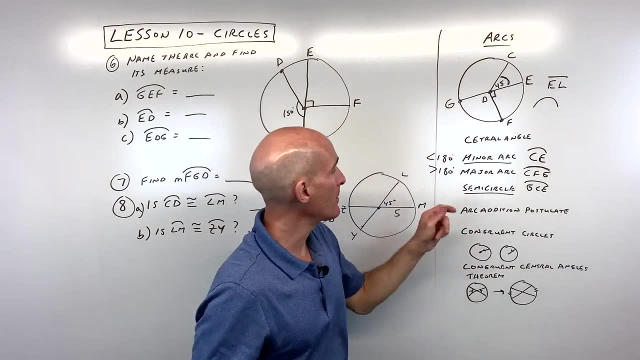 But if I was just to say GE, it would be unclear. am I going this direction or am I going this direction? I'm starting at G, I'm ending at E, but along what part of the circle am I going? So just remember, if it's equal to 180, it's a semicircle. 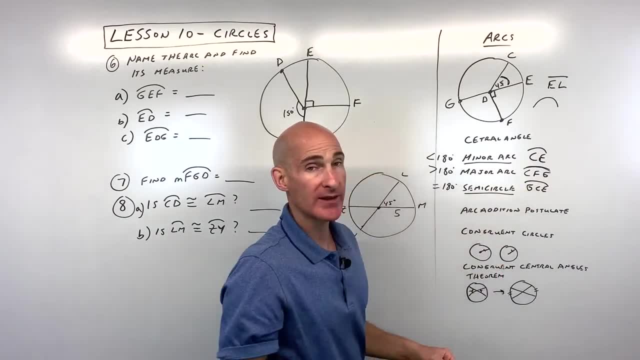 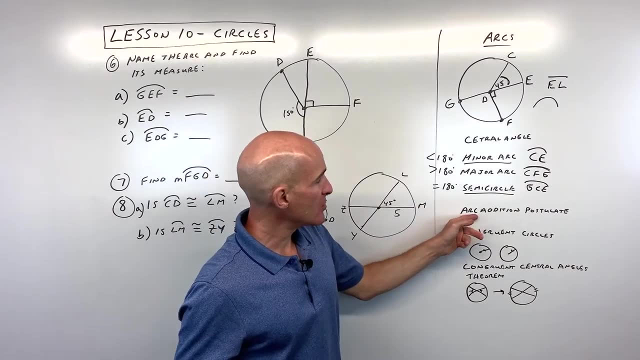 If it's greater than 180, it's a major arc. These ones we have to use three points along the circle. Less than 180, we can just get away with using two points and that's a minor arc. Now what about this here? the arc addition postulate. 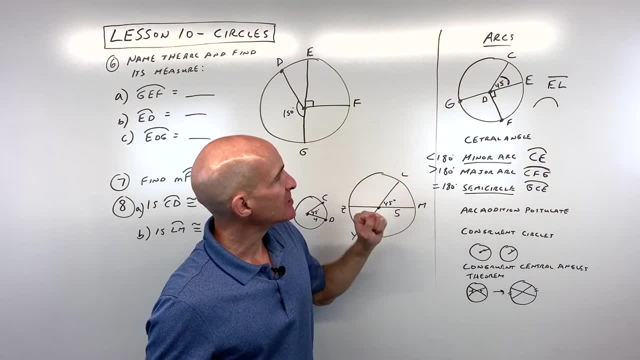 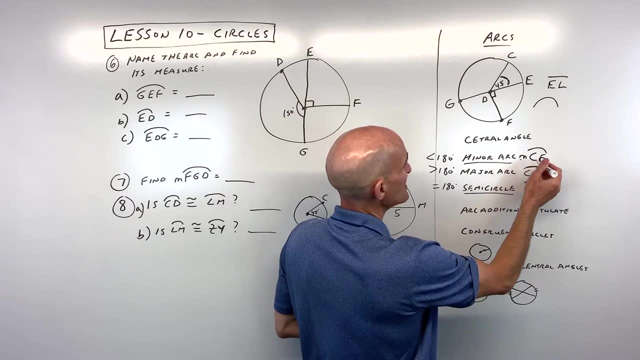 Well, before we talk about the arc addition postulate, I want to talk more about: how do you find the measurement of an angle? So when we talk about the measurement, let's say the measurement, see that M in front, the measurement of CE. that means, like, how many degrees is the arc? 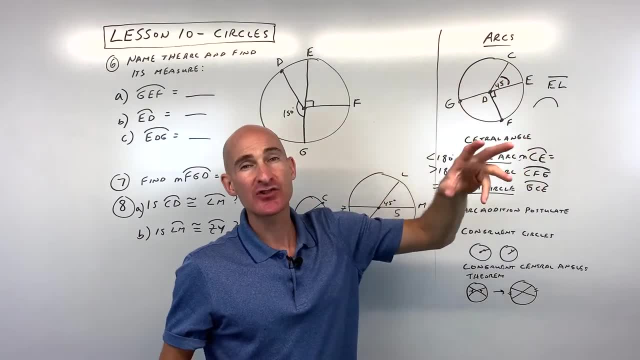 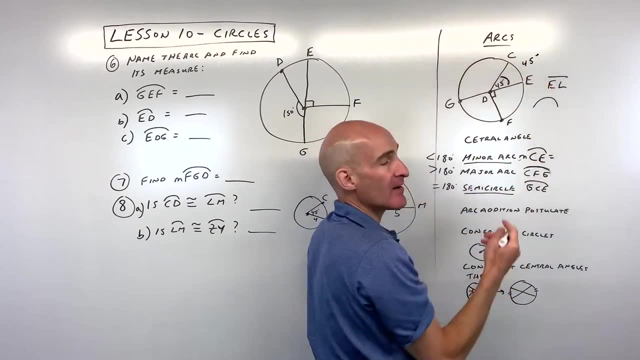 Now the measure of the arc is going to be the same as the measure of the central angle. So if this is a 45 degree angle, then the measure of this arc, we say, is also 45,. okay, so they match. 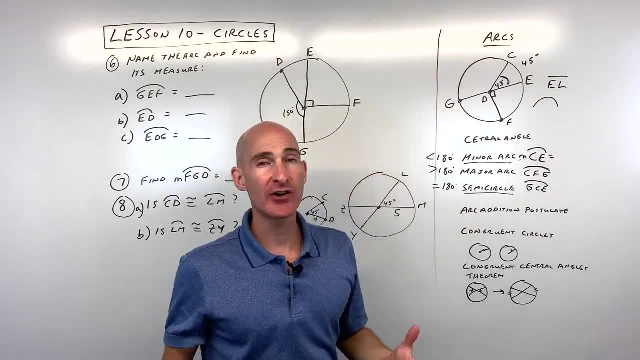 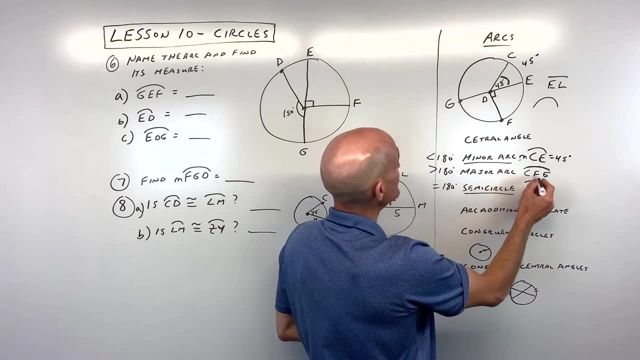 And in a circle, all the arcs would add up to a total of 300.. Okay, So that's going to be 160 degrees, That's the measure. So let's write that down here. 45. Let's say, if we want to do, let's say CFG, so C to F to G. well, you can see that this. 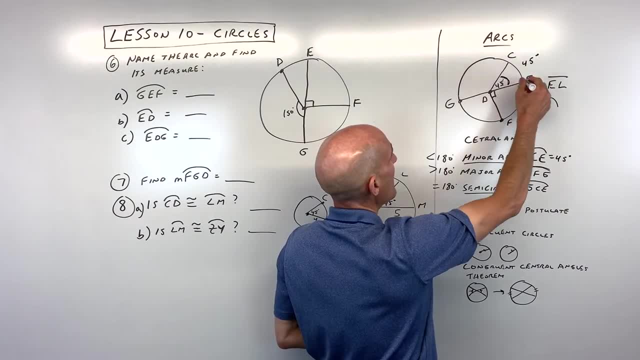 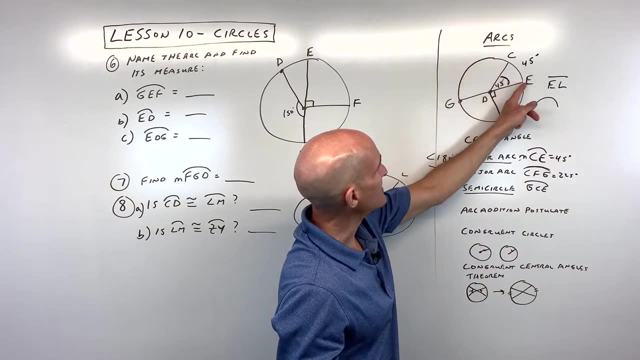 is 180, because this is a diameter, plus this 45, so that's actually going to be 225 degrees And if we do GCE, that's a semicircle, that's halfway around- that's going to be 180 degrees. 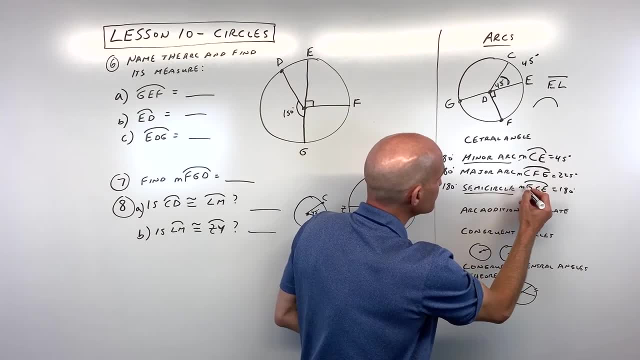 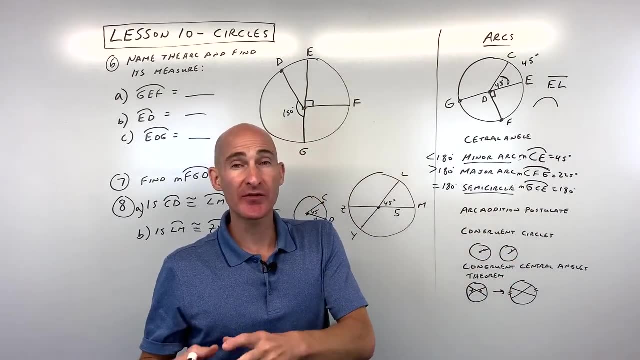 So if you want to find the measure, they'll write it like this, with a little M in front. that's the measure of the arc. like how many degrees? But the arc addition postulate we learned earlier in the course about the segment addition. 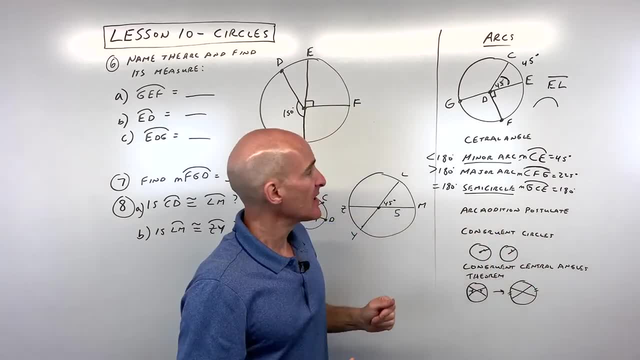 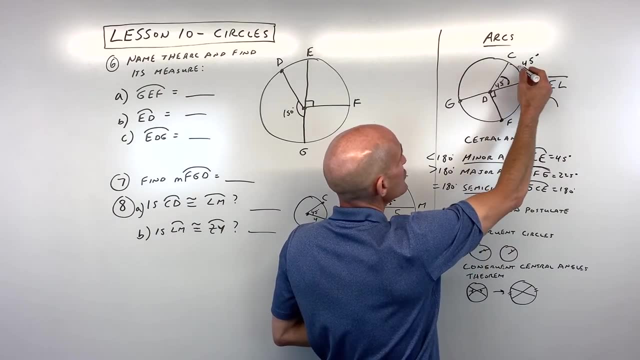 postulate like two segments add up to the whole length. It's the same thing here with the arc addition. If I say the measure of CE plus the measure of EF is going to equal the measure of CF, it's like those two added together give you that whole length. 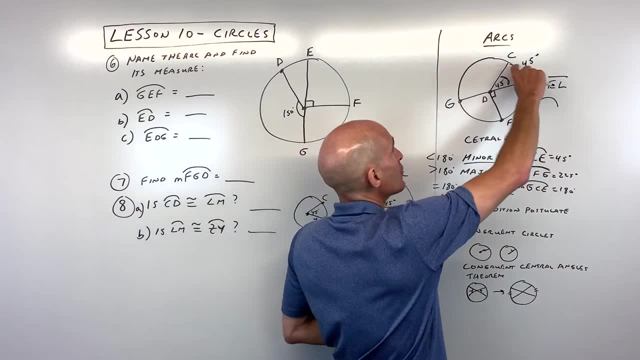 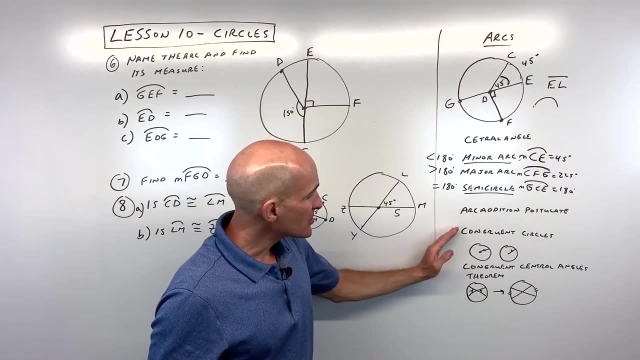 And that's assuming that they're not overlapping, they're adjacent to one another, they share the same endpoint here. That's the arc addition postulate Now: congruent circles. we know. congruent basically means if we, you know, cut the figure out. 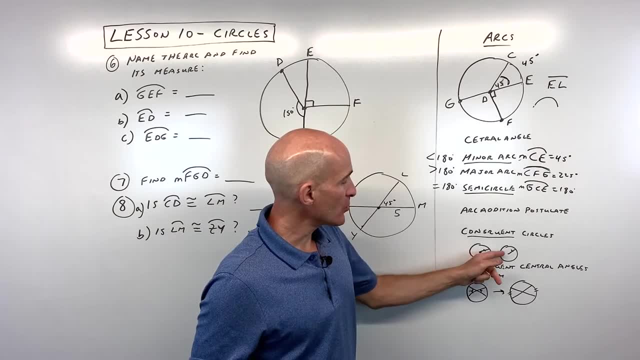 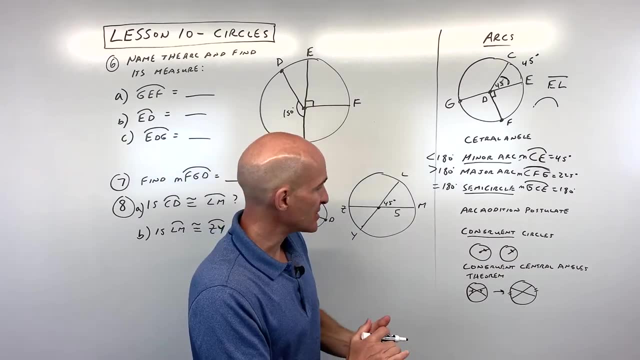 place it on the other figure. it's an exact match right, But with congruent circles. you know they're congruent because the radius is the same length in both circles. So that's how you know. if you cut one out, match it up with the other one. it's going. 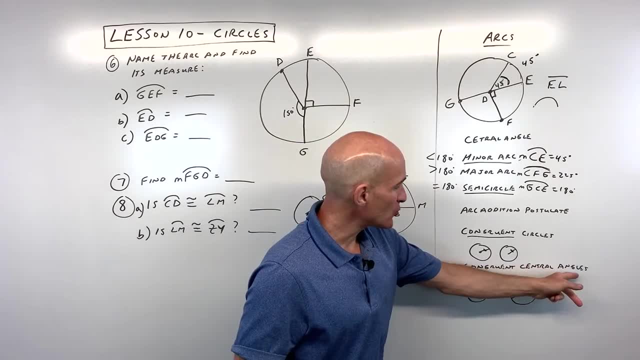 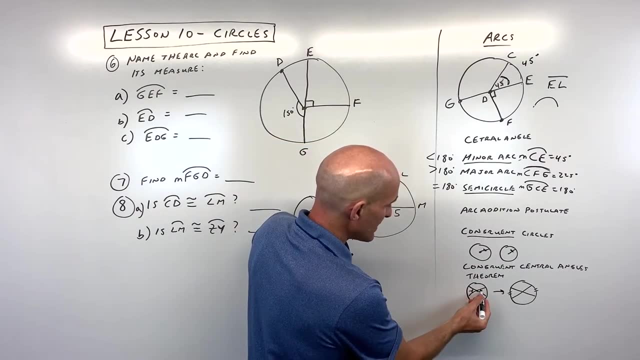 to be an exact match. And then here the congruent central angles theorem. What does that mean? It's kind of a long phrase there. Well, if the central angles- Okay, For example, these two angles here- are the same, they're congruent- then the arcs that 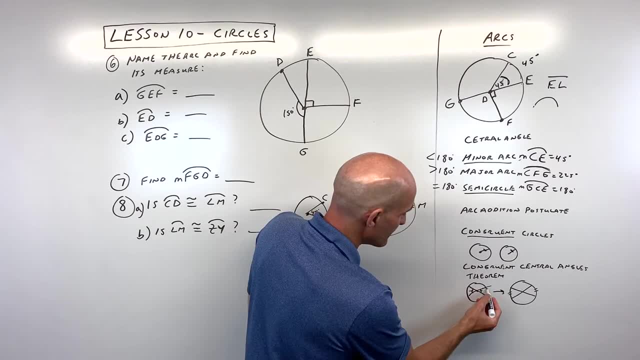 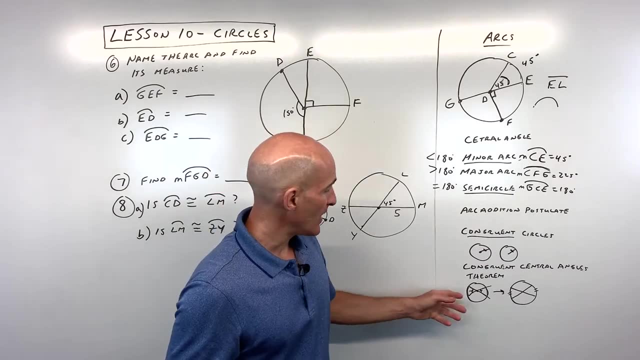 they intercept, like if you were to continue these angles, see how they cut off these two arcs here and here those arcs will be congruent. Okay, So that's the idea. Now, these are two. these are basically in the same circle. 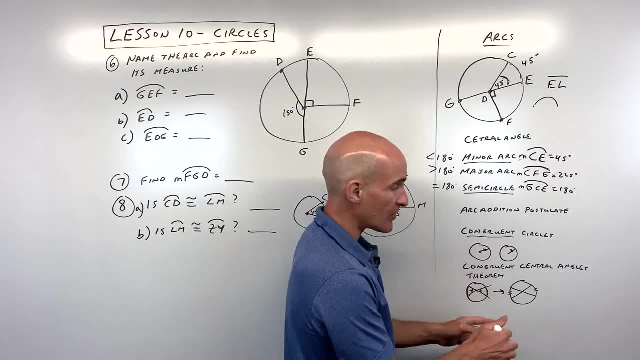 You have. they have the same center, they have the same central angle, So the arcs that they intercept are going to be congruent. But it also works if you have congruent circles. So, for example, if I had like another circle here. 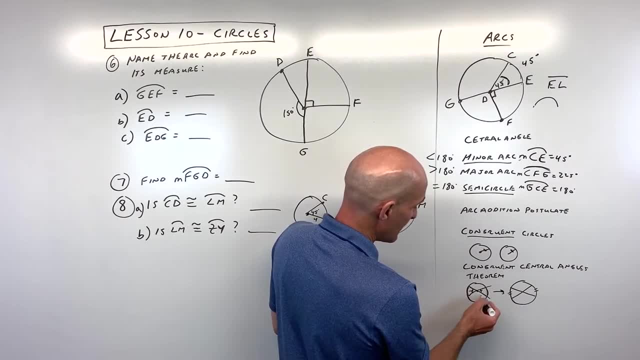 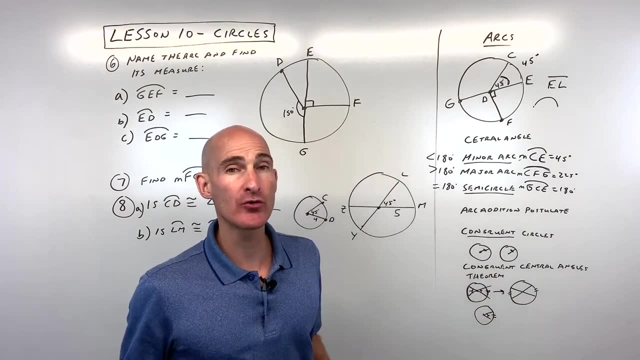 And if I knew that these angles were the same and the circles were congruent, then I know that these arcs here will also be congruent. So it works within the same circle, or congruent circles. if they have the same central angle, the arcs will be congruent. 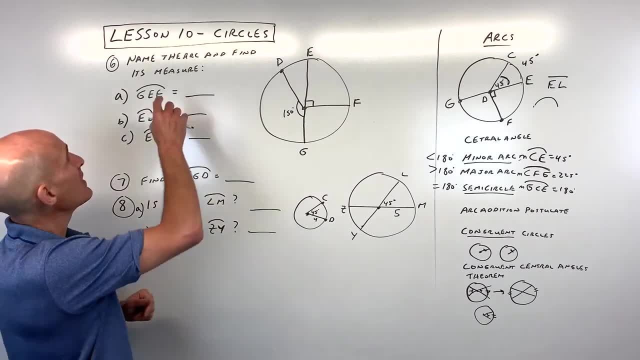 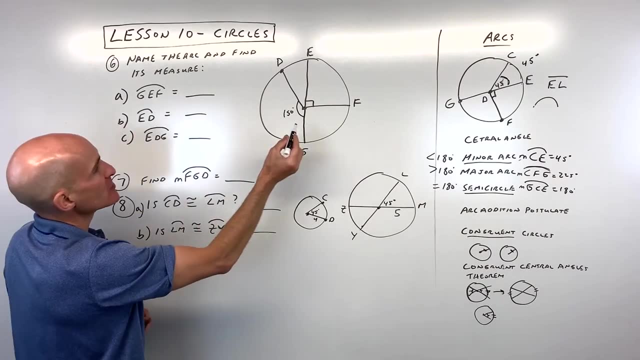 Okay, So let's practice a little bit here. So let's go to number six. It says: name the arc and find its measure. Okay, So here we have arc G E F. So let's look over here: G E F. 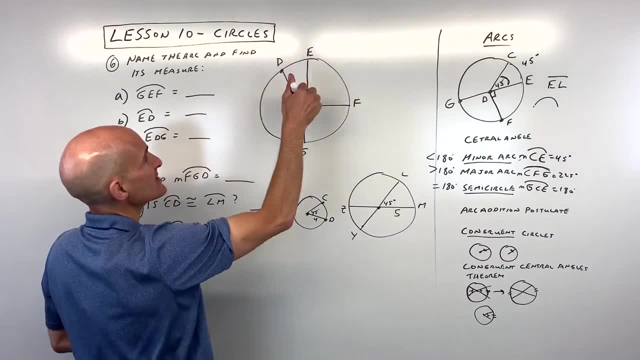 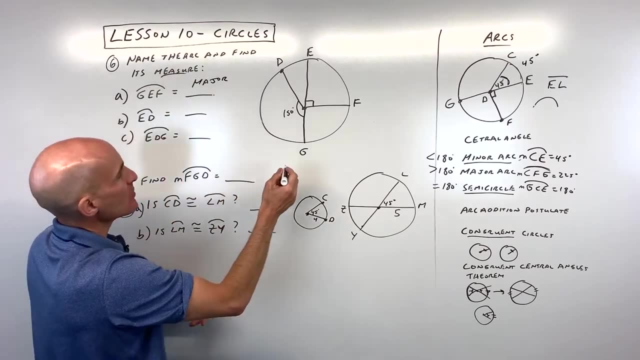 Okay, So this is definitely more than 180, because you can see that G, E is a diameter. So this is going to be a major arc. I'll just write major And the measure: how many degrees. Well, let's see. 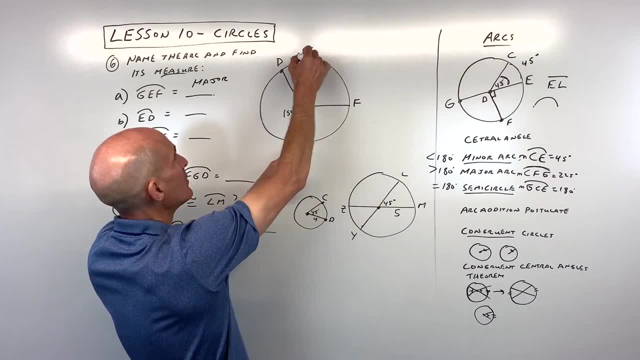 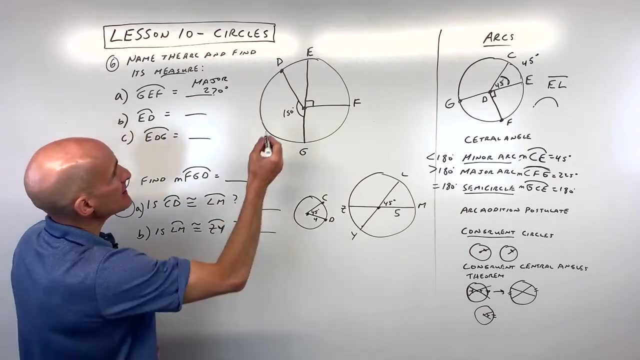 So G to E, that's 180, because this is a diameter, that's a semicircle, plus another 90, see that right angle, So that looks like it's 270 degrees. Okay, How about arc E, D? 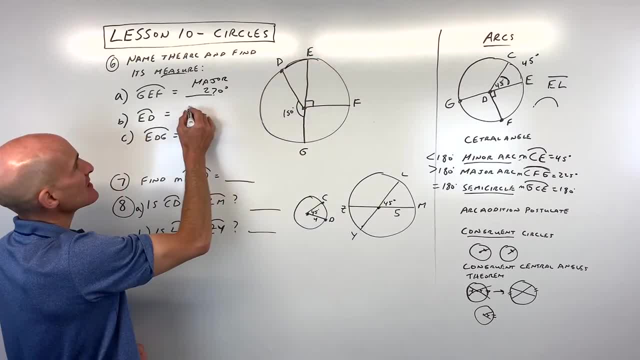 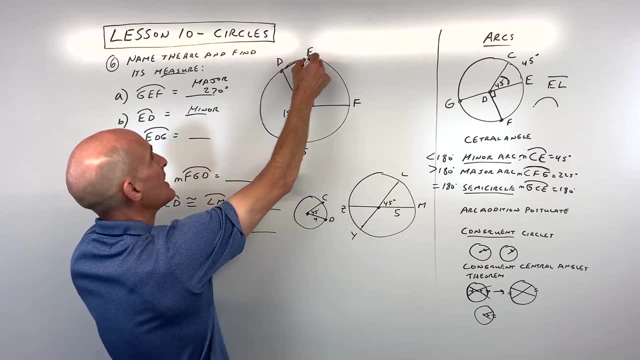 So E D is right here. You can definitely see that's less than 180, so we would say that's minor. But how many degrees? Well, you can see that this is a diameter that's going to be 180.. This is 150, so it takes 30 more. 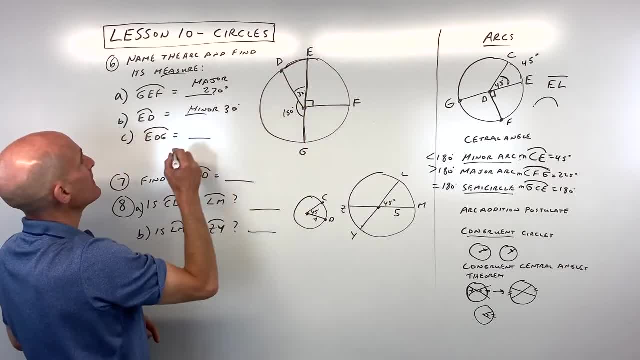 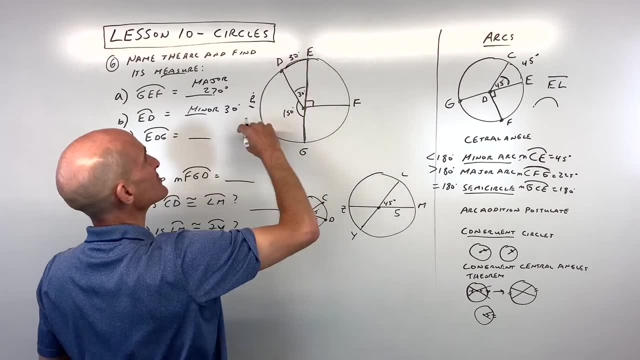 Okay, So this would be 30 degrees. Notice the central angle and the arc measure. they're the same. If this is 150,, this is 150.. If this is 30,, this is 30,. right, This is 90,, this is 90. 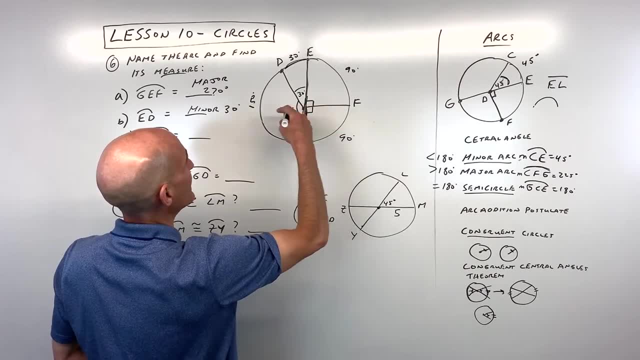 This is 90. here this has to be 90, because that's a linear pair, which means this is 90. And if you add all those up, they're going to add up to 360.. Okay, Now, how about for E D, G? 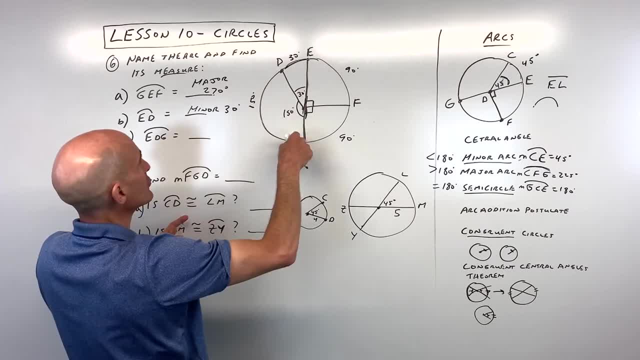 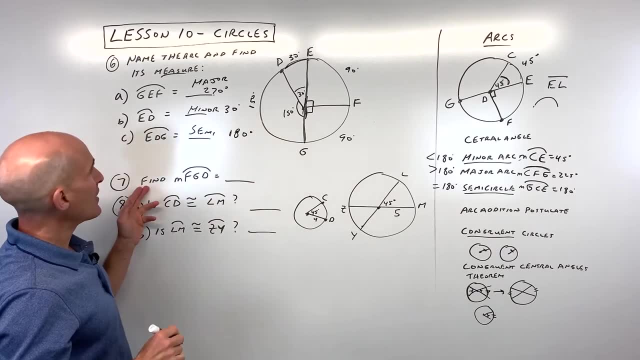 Let's see where is E, D, G, E D G. oh, that's a semicircle, so I'm just going to write semi and we know that's going to be 180 degrees. Okay, Let's go down to number seven here now. 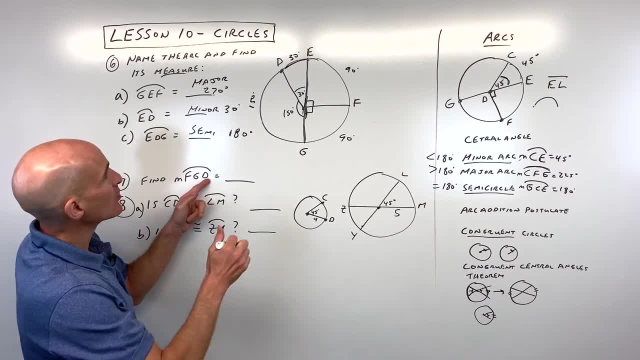 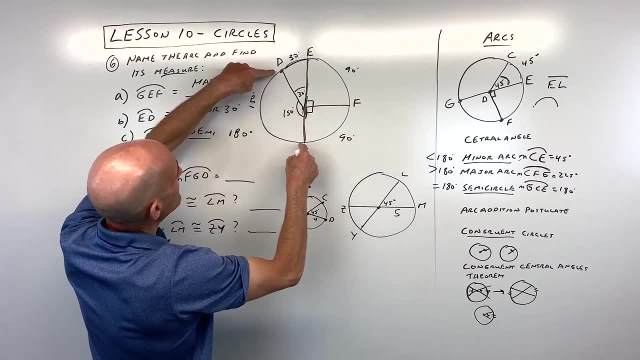 It says: find the measure of arc F G D. So where is F G D? So F to G to D? So we're basically let's do this: we're going 90 plus another 150, we're using that arc addition postulate. 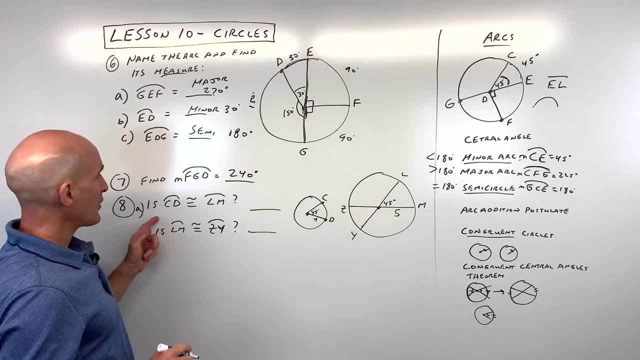 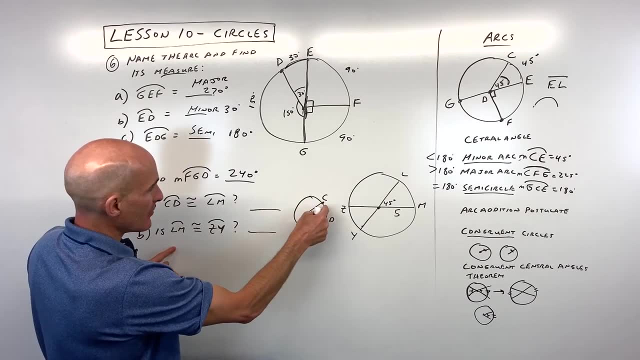 That's going to be 250.. That's going to be 240 degrees. Okay, For number eight. it refers to this diagram, parts A and B. It says is arc C, D- that's this guy right here- congruent to arc L, M. 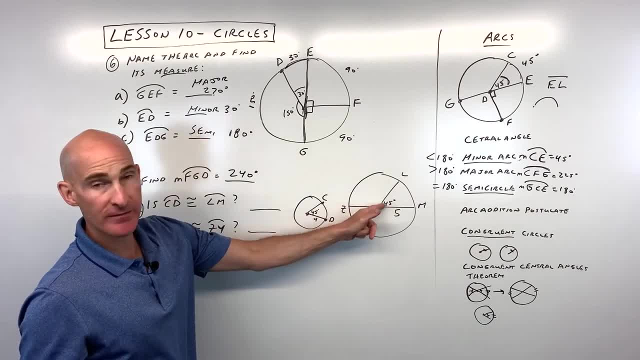 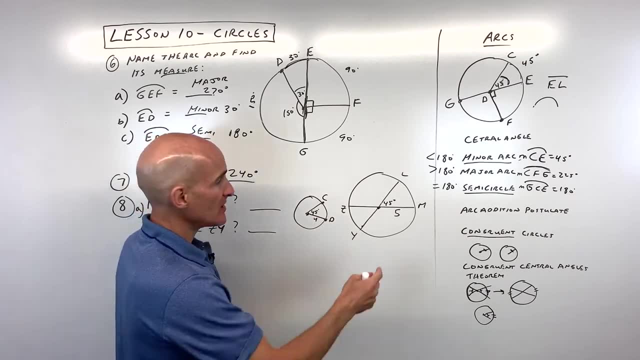 That's this guy right here. What do you think? This is 45,. this is 45. It looks like the. now, this is where you don't want to get confused. The measure of arc C, D is 45 degrees. The measure of arc L, M is 45 degrees because see the central angle and the measure of the. 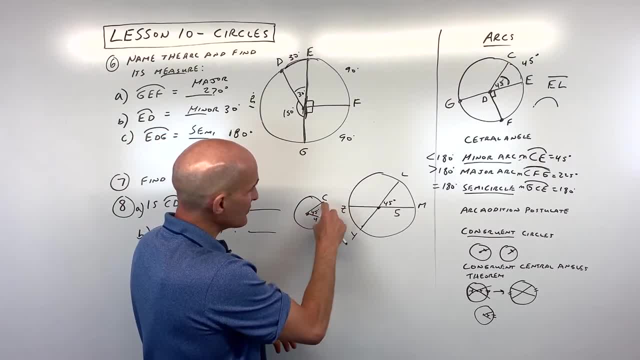 arc. they're going to be the same. But if I cut this little piece right here, this arc, and I place it on here, is it going to be an exact match? Are they going to match up? perfectly Well, no. 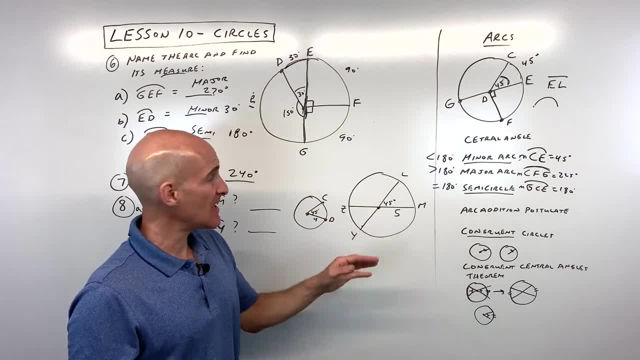 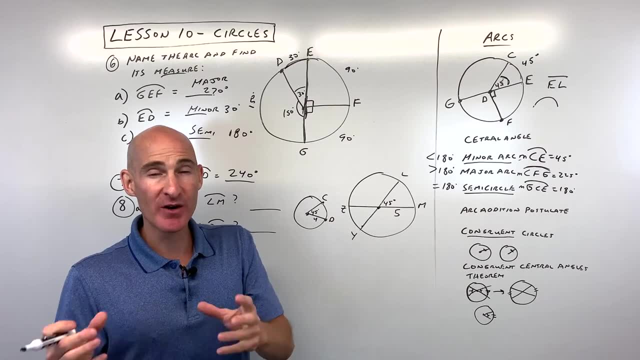 And why not? Because these circles are not the same size. This circle is obviously bigger. So don't get confused measurements, you know, like the angle measurements or the arc measurements with the length. Okay, That's different, So they're not congruent. 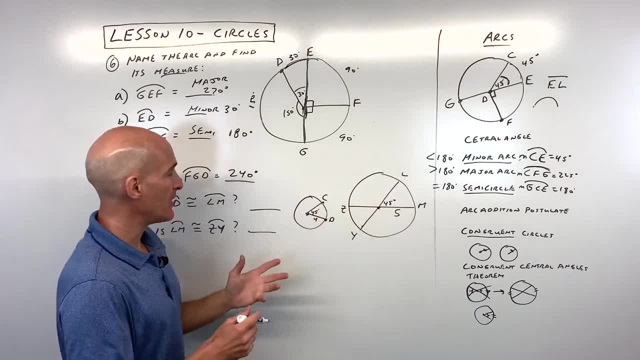 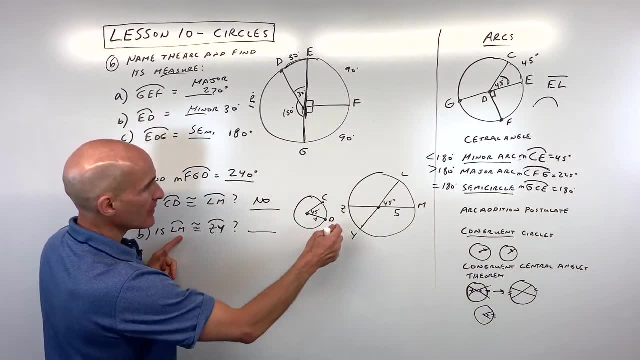 They have the same measure, meaning like the same number of degrees but not the same length. So we're going to say no, Okay. So we're going to say no because the circles are not congruent. And then, for part B, is arc L, M, this arc right here, congruent to arc Z, Y. 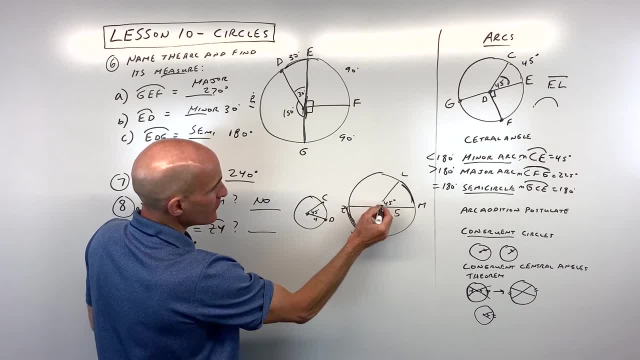 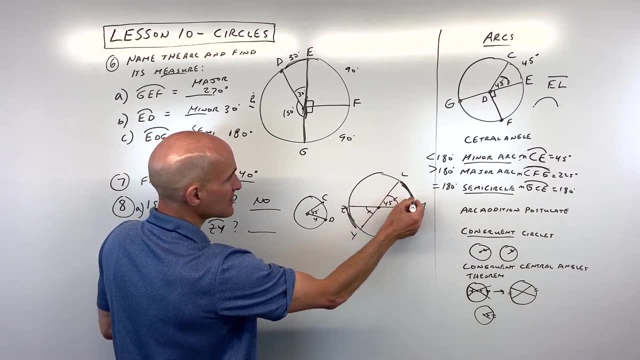 Well, see, if this is 45,, this is 45, because these are vertical angles, right, And if the central angles are congruent and within a given circle, then the arcs that they intercept will also be congruent. So this is going to be yes. 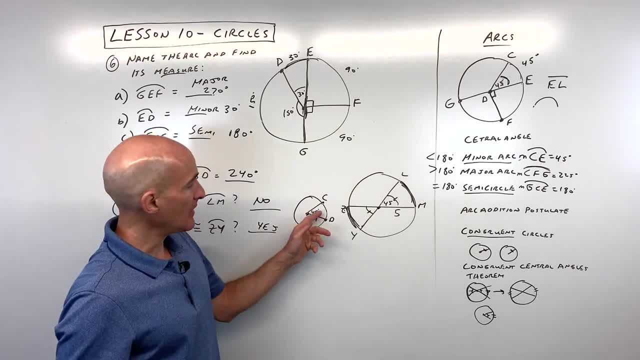 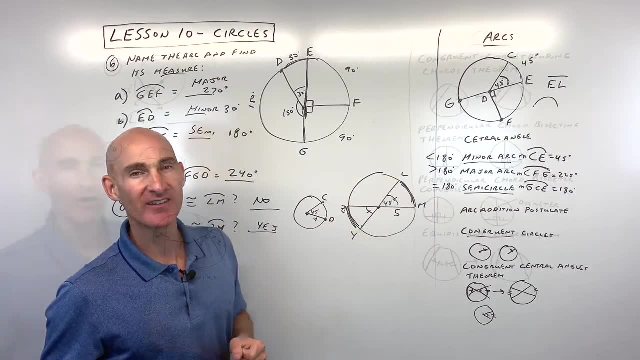 So, again, it works. whether the circles are congruent, you know, and they have the same central angle, Or within a given circle, then if they have the same central angle, the arcs that they intercept are going to be congruent. Okay, 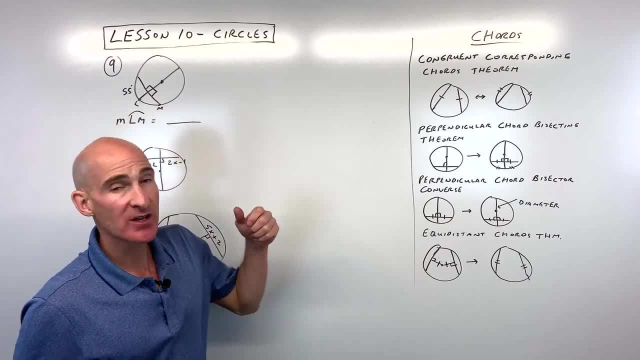 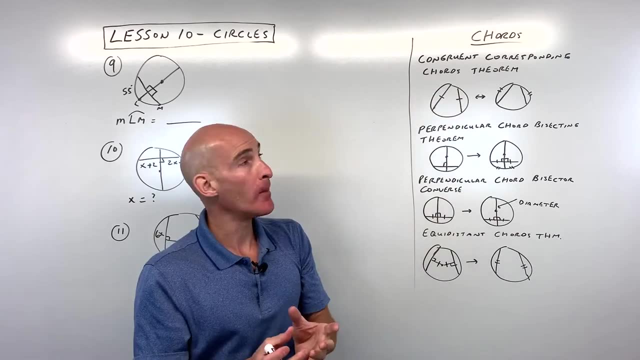 Let's talk about some theorems related to chords. We talked about what a chord was earlier in the lesson. here It's a segment that connects two end points that lie on the circle. But first let's talk about the congruent corresponding chords theorem. 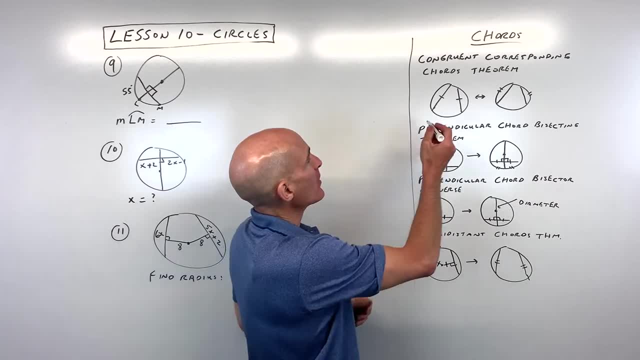 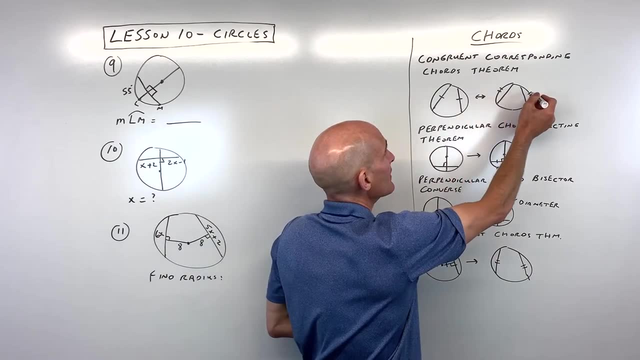 Okay. So that's a lot to say there, but what it means is that if you have two chords that are congruent, they're the same length, Okay, And then we know that the arcs that they cut off or intercept are also going to be. 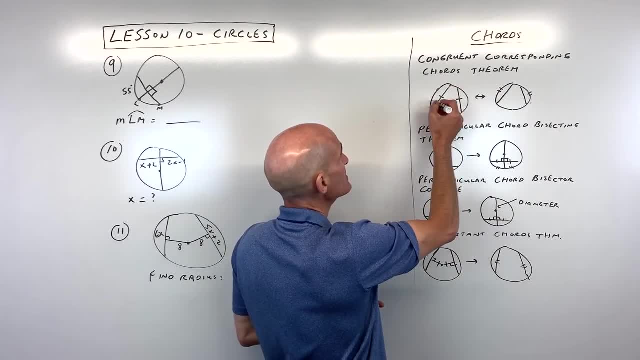 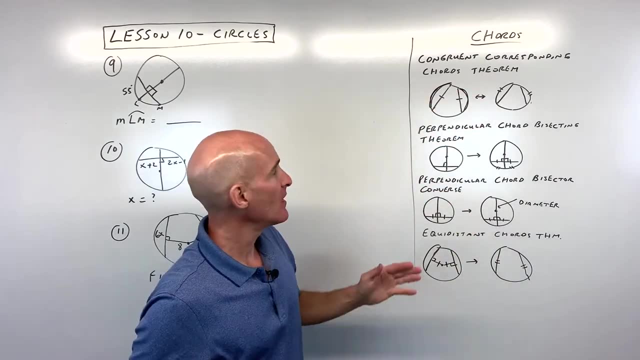 congruent. So does that make sense? So if this chord and this chord are the same, then these arcs here are going to be congruent. They're going to be the same. If you cut one out, match up with the other one, it's going to be an exact match. 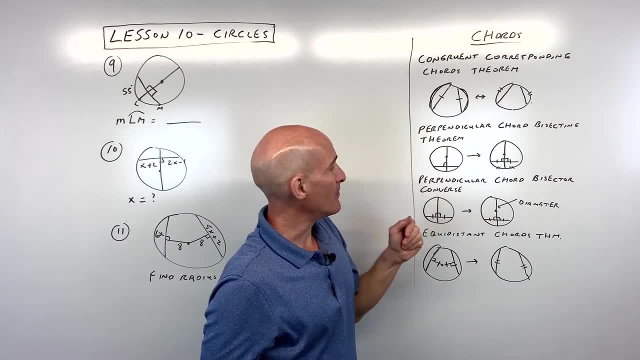 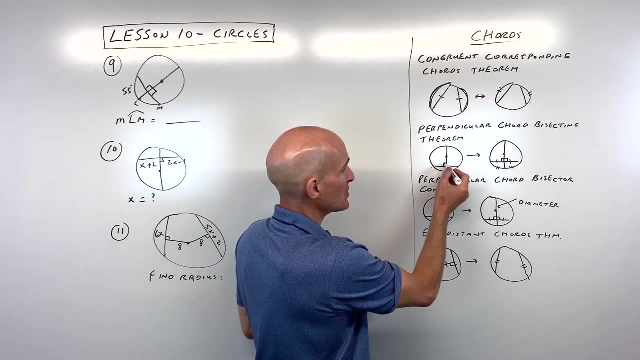 Okay, The perpendicular chord bisecting theorem. Okay, So what this is telling us is that if you have a diameter- okay, and it's perpendicular, that meaning 90 degrees to a chord, it will bisect the chord, It'll cut it in half. 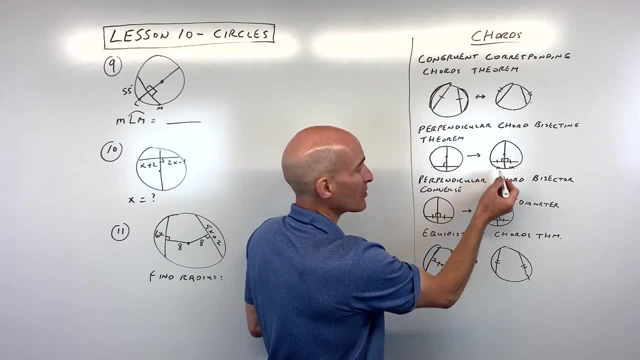 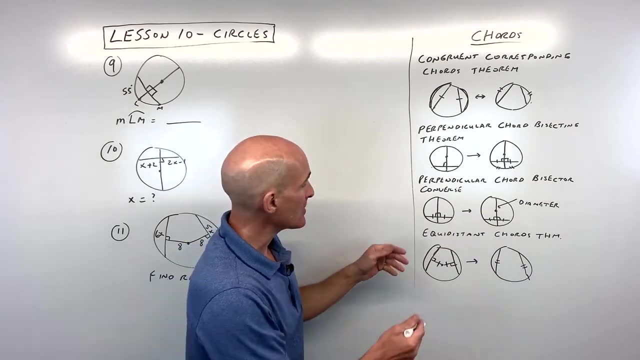 It'll cut it in half as well as it will bisect the arc. It'll cut that arc in half. And then the perpendicular chord bisector converse. of course the converse means you're saying it in reverse: If you have a chord and it's perpendicular to another chord and it bisects that chord. 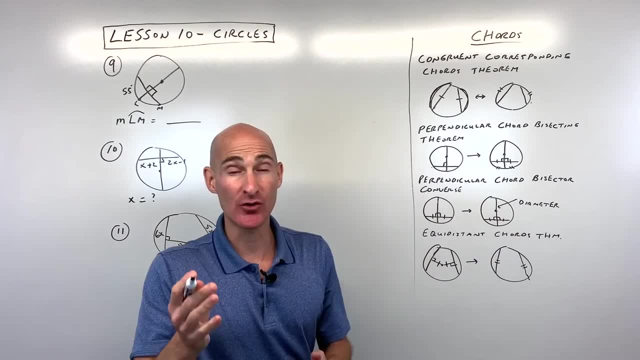 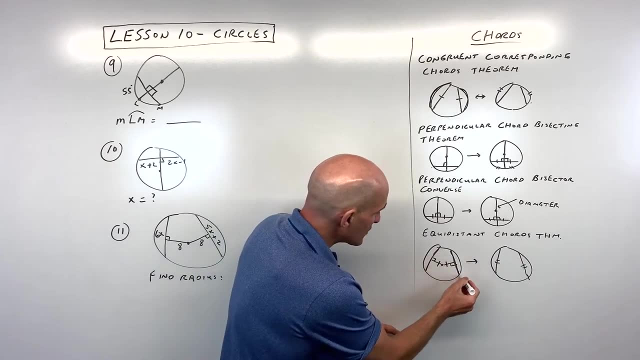 what do you know about this chord here? Well, it must be a diameter, meaning it goes to the center of the circle. And then the last one, equidistant chords theorem. See, if you look at these two chords here and if they're the same distance from the 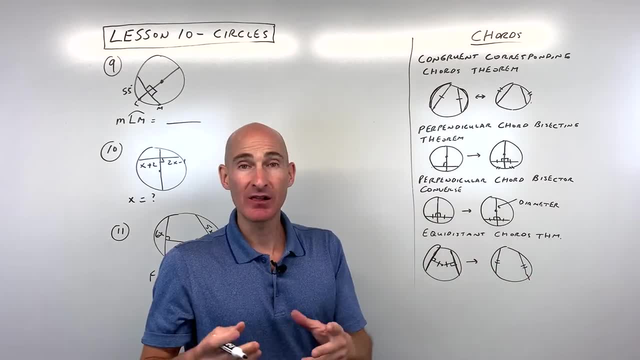 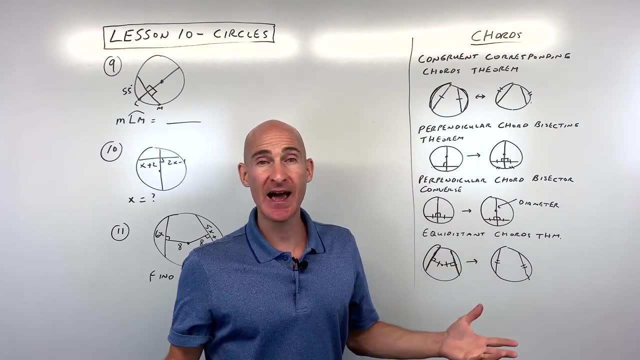 center, then you know that those chords have to be the same length. See, the closer you get to the center of the circle, the chords are going to get longer, longer, longer, until the longest one, which is the diameter, goes right through the center. 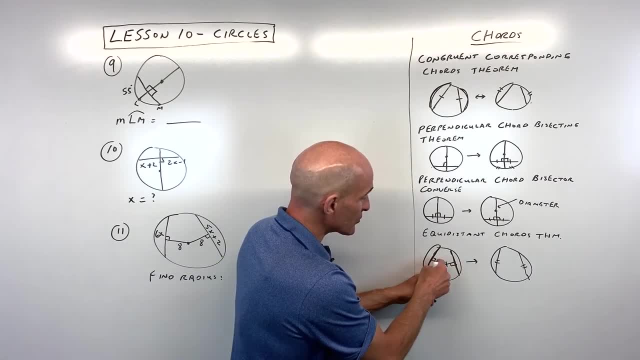 of the circle. But if they're the same distance from the center of the circle, then the chords are going to be the same length. Remember, when you measure the distance from a point to a line, you always want to measure that perpendicular distance, that 90 degree or right angle distance. 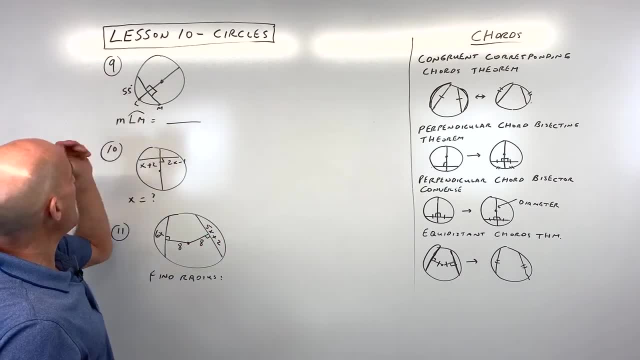 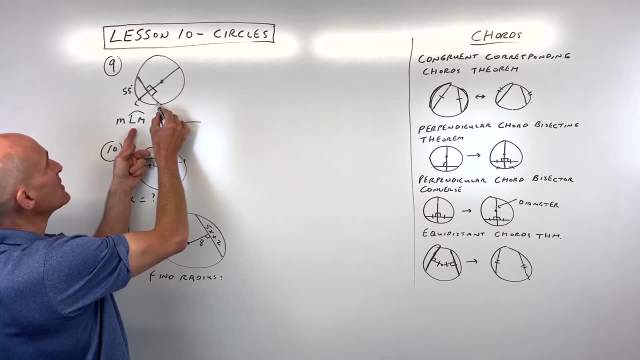 That's going to be the distance. So let's do a few examples For number nine. here You can see we have a diameter goes right through the center of the circle. It's perpendicular to this chord here. So what do we know? 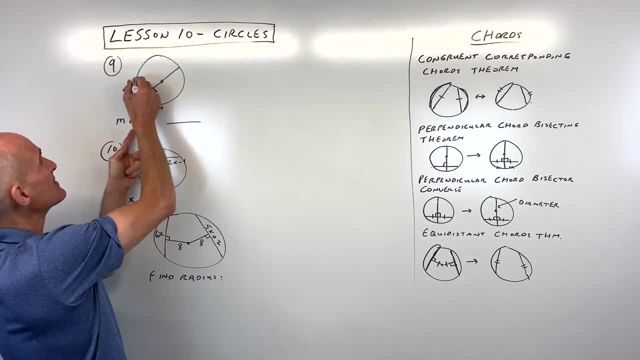 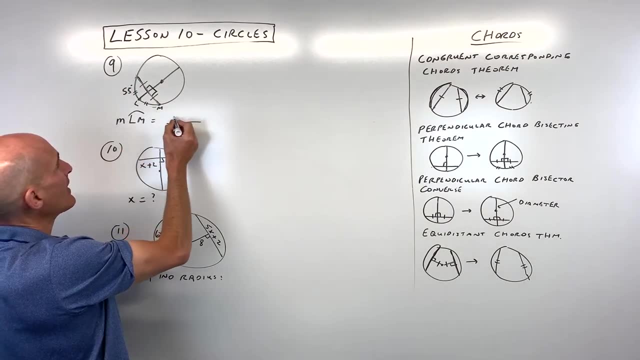 We know it bisects the chord. It also bisects this arc, meaning it cuts the arc in half. So what's the measure of arc LM? Well, if we know that this arc here is 55, LM will also be 55 degrees. 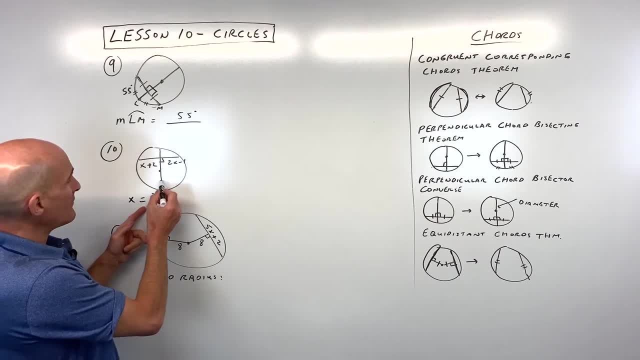 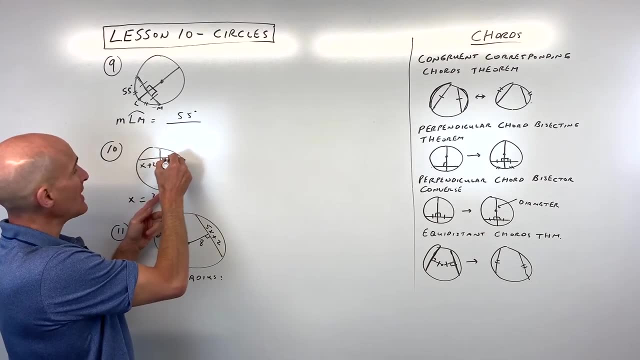 Okay, let's do number 10.. So this one we have is we have a diameter. see, it goes right through the center of the circle. It's perpendicular to the chord. What do we know? It's perpendicular to a chord. It's going to bisect the chord. of course, it will also bisect this arc. 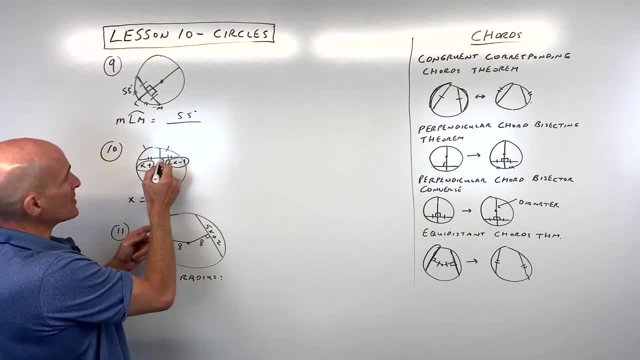 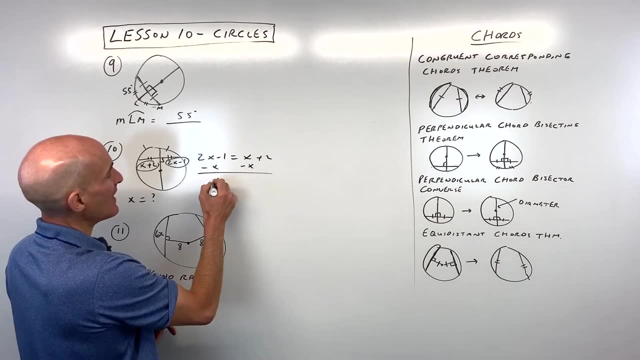 But we know that these lengths, these chords, are going to be congruent, or I should say these segments are going to be congruent. So we have 2x minus 1 equals x plus 2.. Let's subtract x from both sides, add 1 to both sides and you can see x equals 3.. 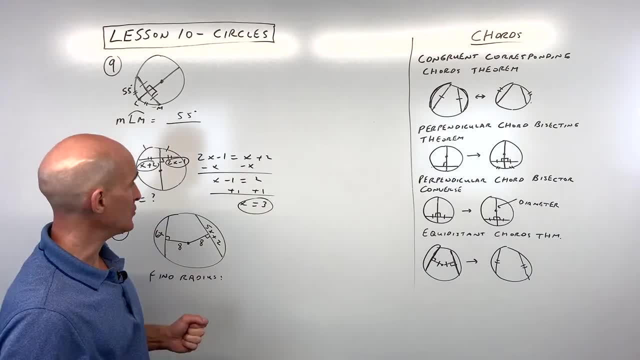 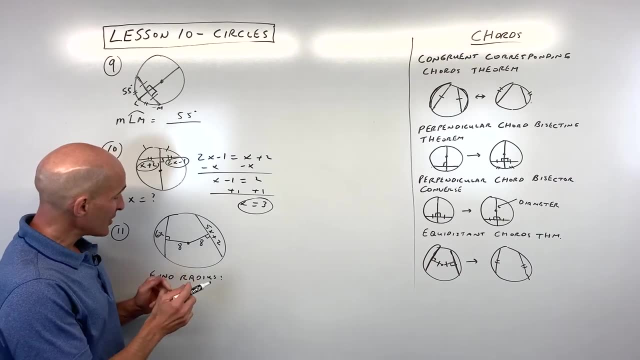 Now if you put 3 back in, you know you can figure out the length of that chord if you need to. For number 11, it says: find the radius of the circle. Now this one's a little bit more challenging, But let's look at the clues. 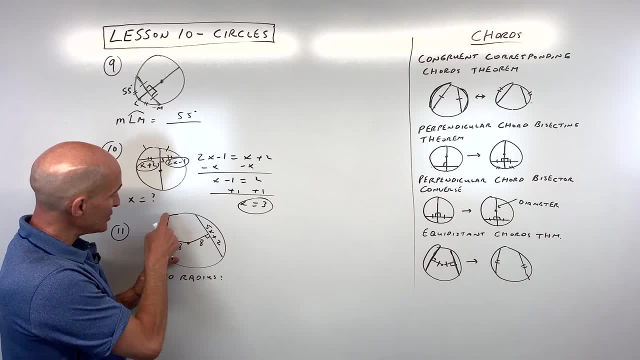 So notice that the distance from the center of the circle to each of these chords is 8 units. Well, if the chords are equidistant, meaning the same distance from the center, what do you know about their lengths? They must be equal. 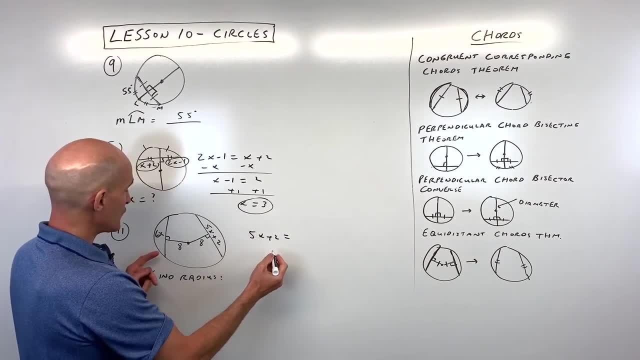 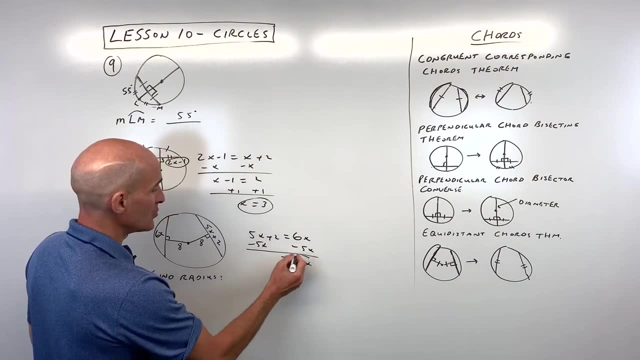 So let's go ahead and figure out what the lengths of these chords are. So 5x plus 2 must equal 6x. If we subtract 5x from both sides, you can see that x is equal to 2.. But now, if we put 2 back in, that's going to be 10 plus 2 is 2.. 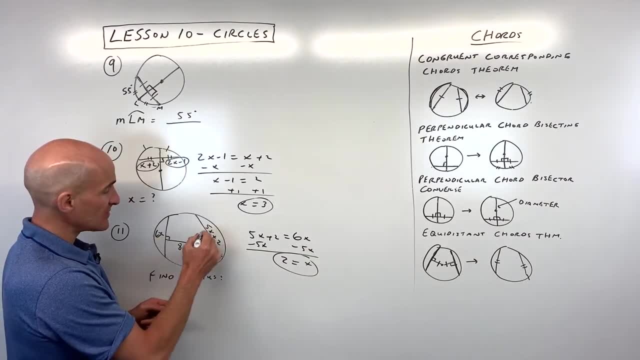 So that's going to be 10 plus 2 is 2.. 6 times 2 is 12.. 6 times 2 is 12.. So we know the lengths of these chords are going to be 12 units If we draw an auxiliary line like a radius here from the center to, let's say this point: 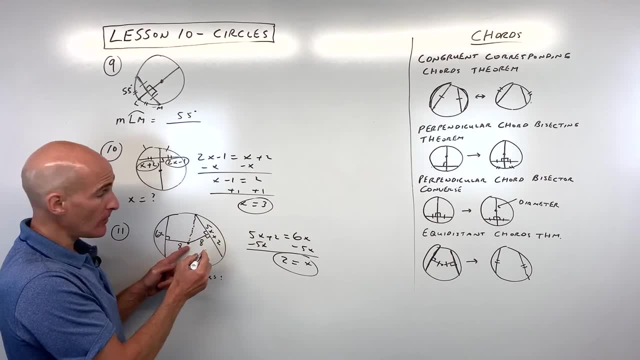 And the reason I'm doing that is to make like a triangle, specifically a right triangle. See, remember how this we figured out. this was 12?. But when you draw a line from the center perpendicular to the chord, it bisects that chord. 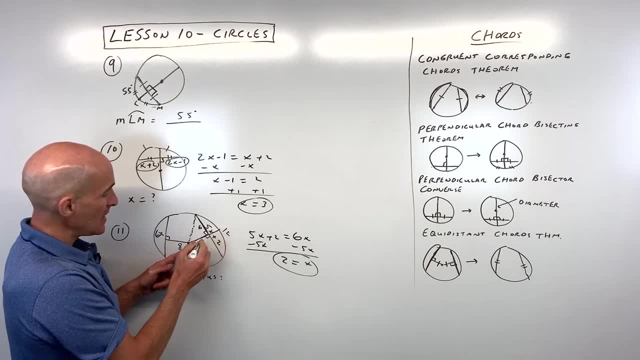 So that means that this length right here must be half of 12,, which is 6.. And now what we have is we have a 6x, We have a 6,, 8,, 10, Pythagorean triple. Or you could do the Pythagorean theorem: a squared plus b squared equals c squared. 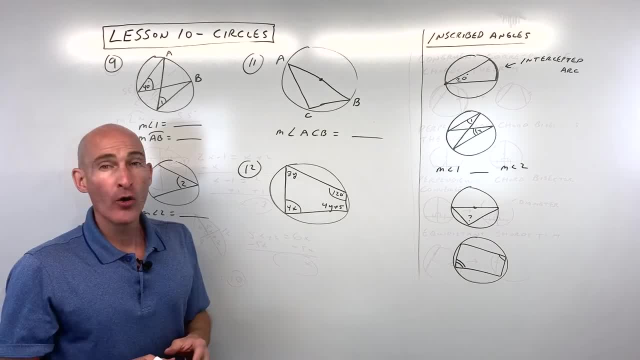 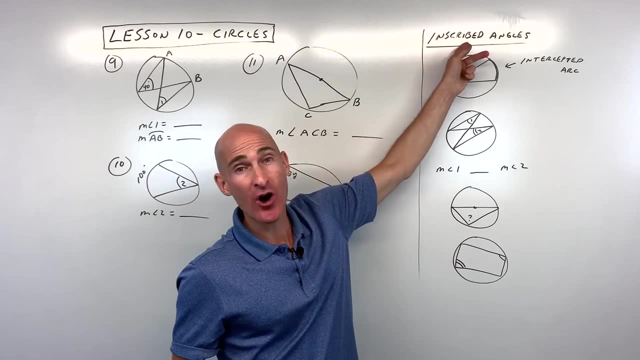 Now we know the radius is going to be 10 units. Okay, let's talk about inscribed angles now. So what is an inscribed angle? Well, scribe means to draw or write In, means it's on the inside, okay, of the circle. 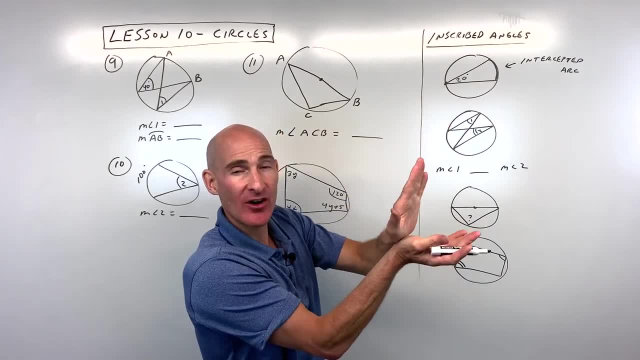 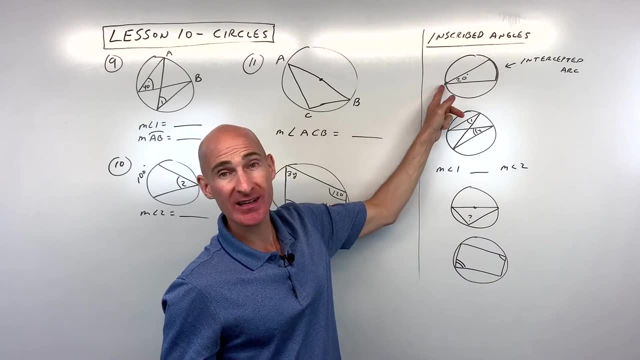 But specifically the vertex or that hinge of the angle lies right on the circle. Now, remember central angles. The vertex was at the center of the circle. Inscribe: the vertex is on the circle. Now, if you follow the sides of the angle, it's going to cross the circle at two points. 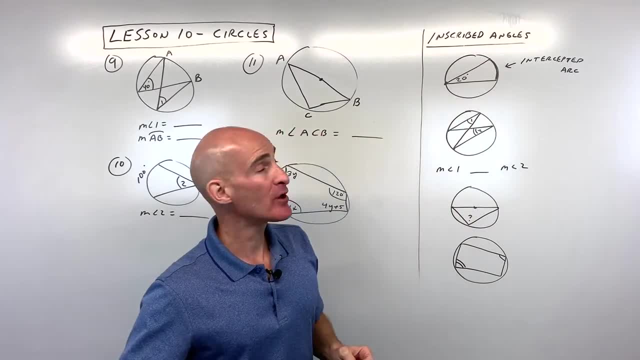 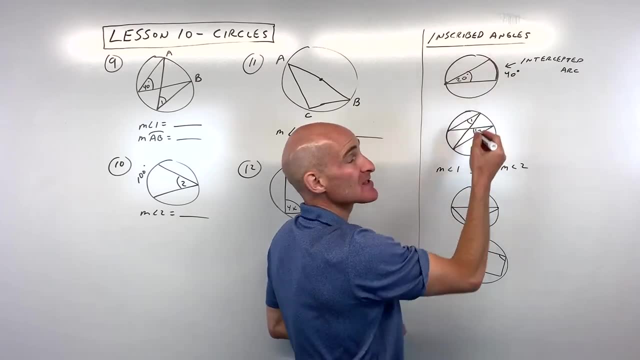 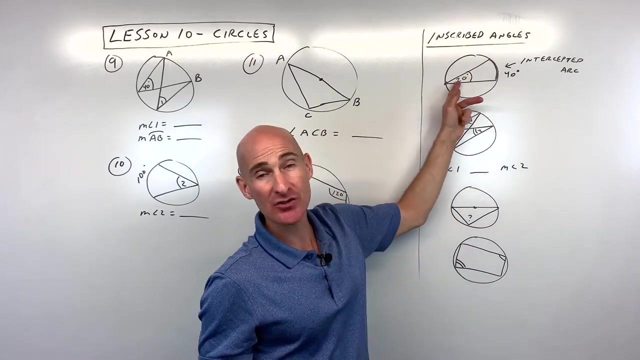 This is called our intercepted arc, And an important thing to remember here is that whatever the measure of the inscribed angle is, the intercepted arc is going to be twice as much. It's going to be 40 degrees, Or you could say the intercepted arc. if you divide that by 2, you get the measure of the. 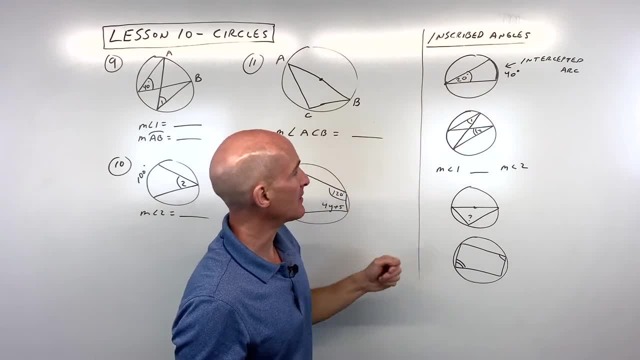 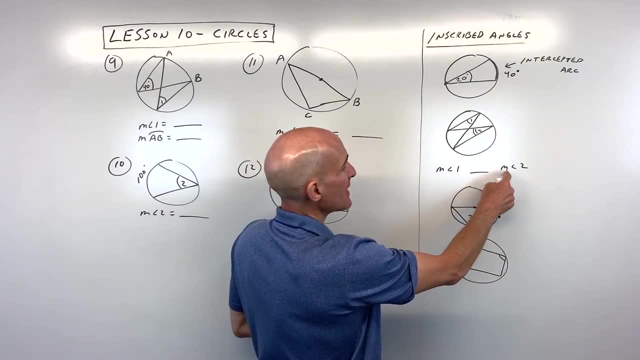 inscribed angle Double or half, however you want to think of that. Now, for this example here, it's kind of interesting: Do you think the measure of angle 1, this angle right here, is greater than, less than or equal to the measure of angle 2?? 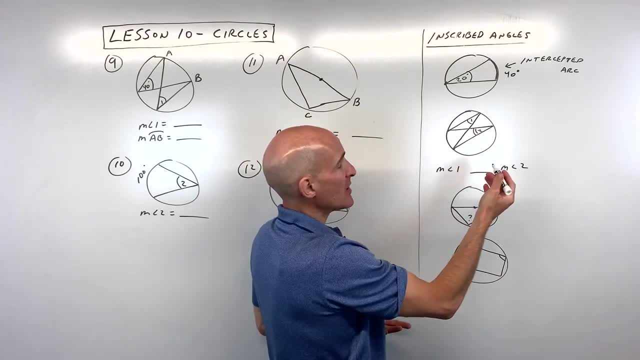 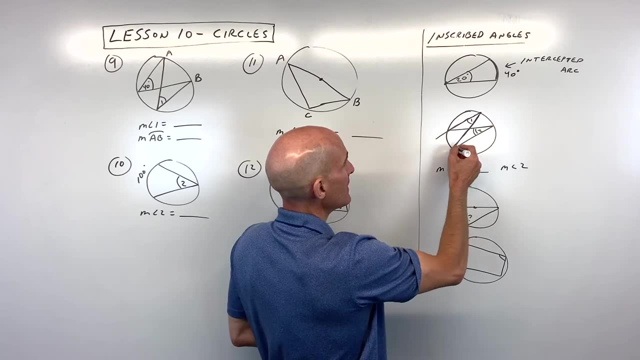 Well, we don't know any measurements here, any degree measurements, but you can see if you look at angle 1, if I follow the sides of angle 1 like this right, it's intercepting or cutting off this part of the circle. 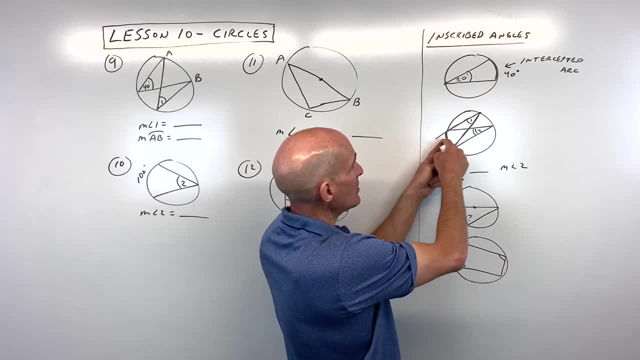 That's our intercepted arc. Whatever this is, Say it's 100. This would be 50. If this was 60,, this would be 30. So the angle's going to be half of this arc. If we look at angle 2, and if we follow the sides of angle 2 to where it crosses the circle, 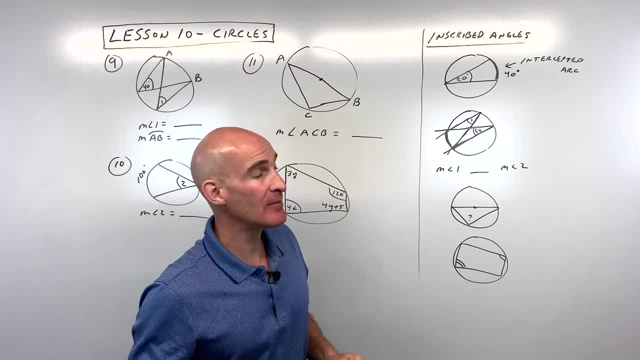 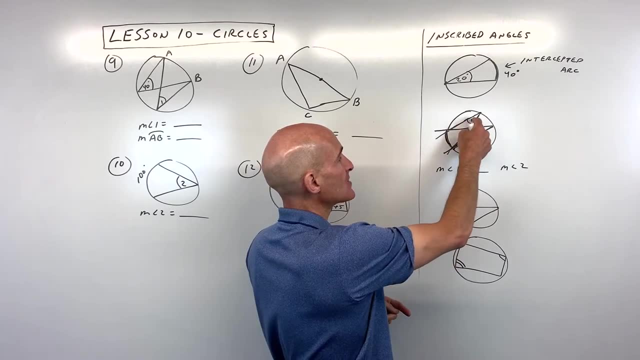 oh look, it's intercepting the same part of the circle. It has the same intercepted arc. So if this was 100, this would be 50.. If this was 60, this would be 30. So because both inscribed angles are intercepting the same arc, their angles are going to be. 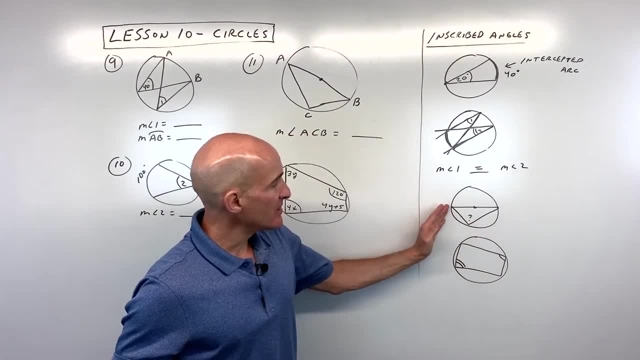 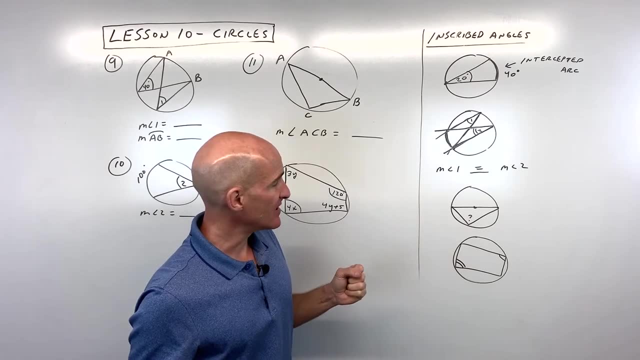 congruent, They're going to be equal. okay, For this diagram here. what do you think this is? What do you think the measure of this angle is right here? Well again, there's not any numbers on this diagram here, but you can see that this chord. 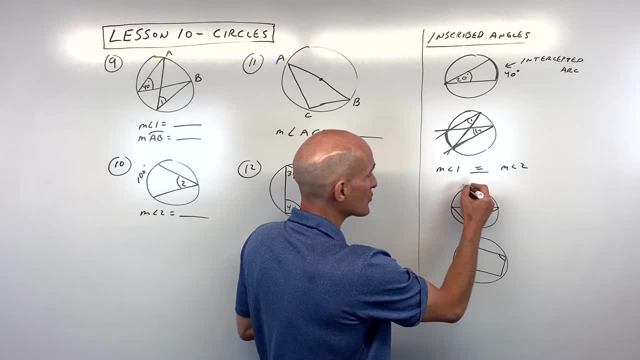 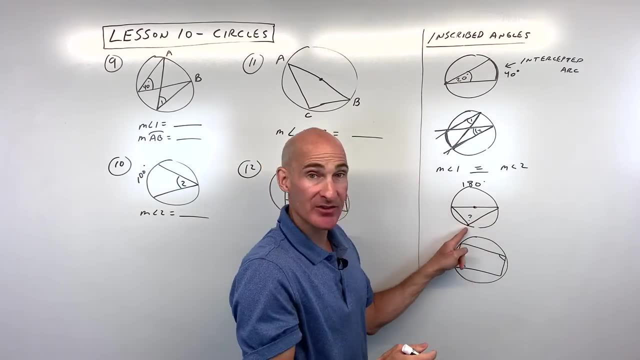 here goes through the center of the circle. It's a diameter. That means this is a semicircle, That means it's 180 degrees. We can see that this is an inscribed angle because the vertex is right on the circle and if you follow the sides of that inscribed angle to where it intercepts the circle, see 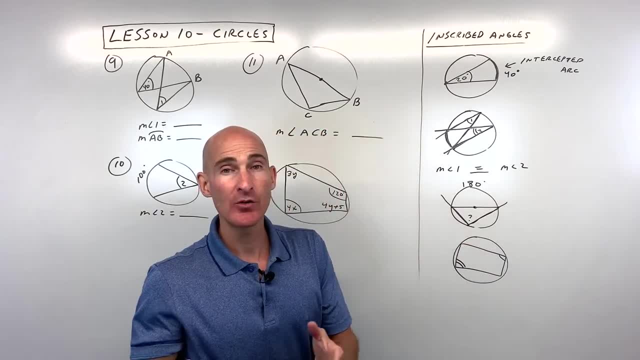 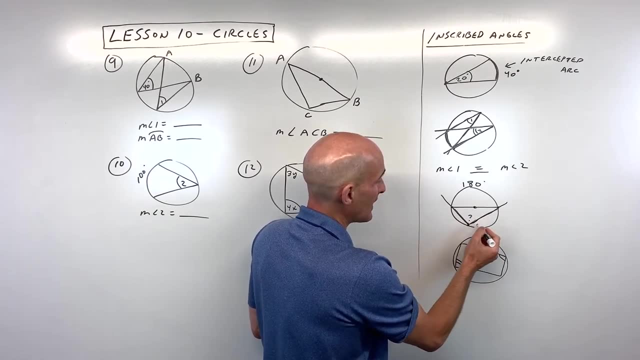 how it's 180?? This is going to be half of 180, which is 90 degrees. Okay, So whenever you see an angle that's inscribed inside of a semicircle, like half a circle, you always know it's going to be a right angle. 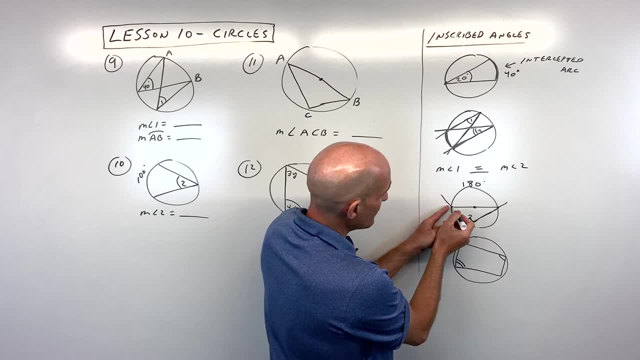 This is kind of a fun exercise here. if you want to play around with it, See, go ahead and go like this. See how I have the ends of the angle- they lie along the diameter here where the diameter intersects the circle- And notice how that forms a right angle. 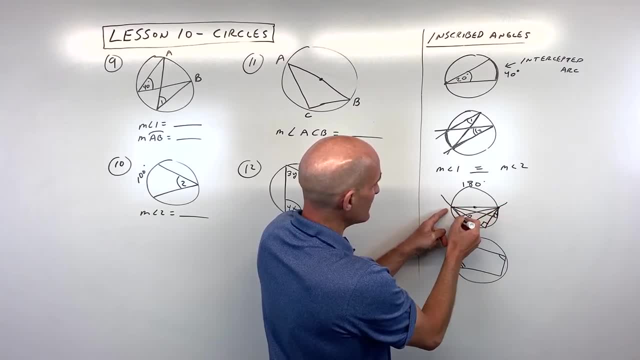 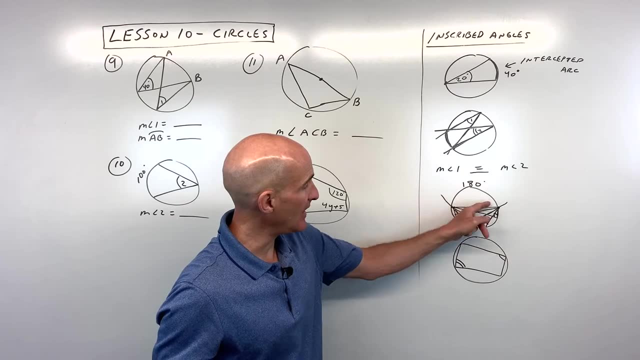 If I go like this, see again another right angle. If I go like this, another right angle. And again, that's because this is 180.. This is an inscribed angle. the vertex is on the circle. it's always half of that 180. 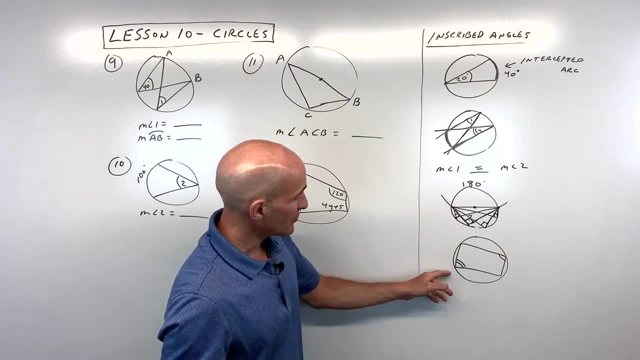 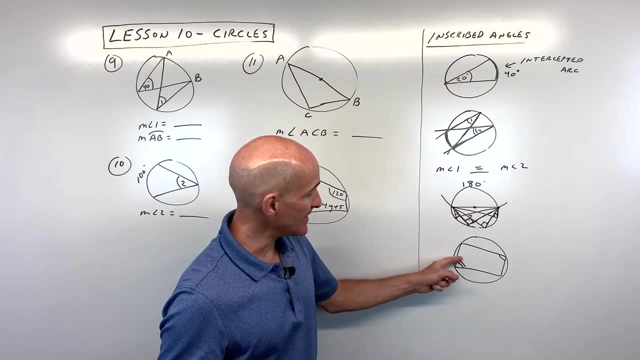 or 90.. Okay, and then for the last introductory example here. this is what we call an inscribed quadrilateral. Again, scribe is to draw in, is on the inside. Notice: the vertices of the quadrilateral lie right on the circle. okay, 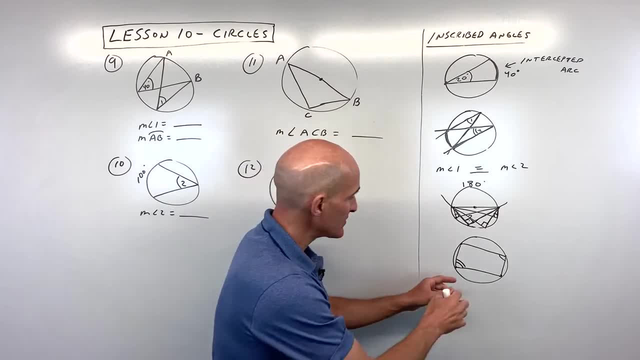 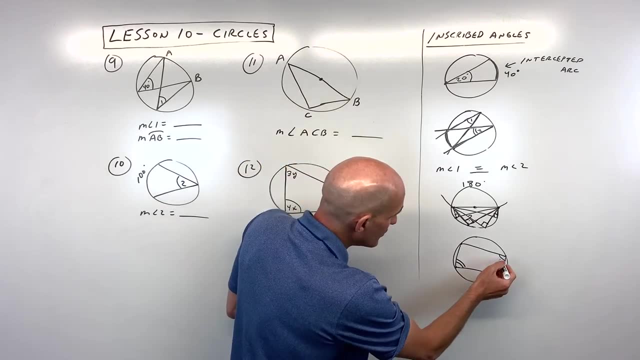 And the interesting property here is that the opposite angles, the ones that are across from each other, these are always going to be supplementary. Now you might be saying, Mario, why are they supplementary? Well, take a look at angle one right here. 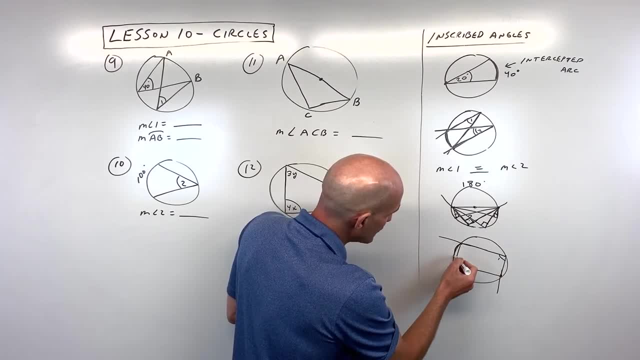 If I extend the sides of that angle, see how it's intercepting or cutting off this part of the circle right here. Now let's call this angle two. If I take the sides of angle two and kind of extend those, see how it's cutting off. 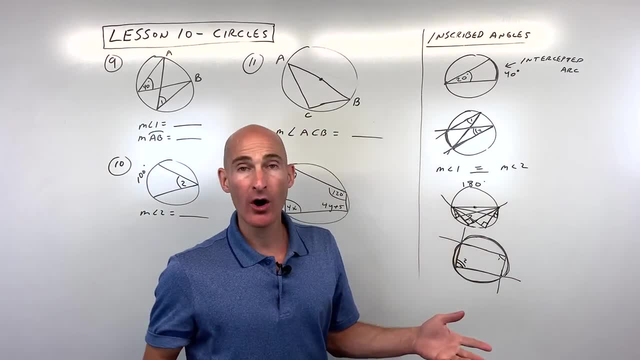 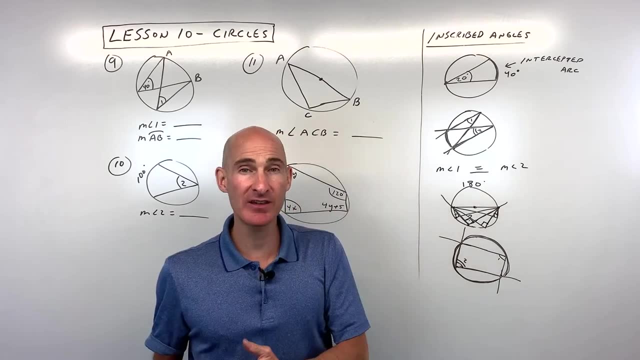 the rest of the circle. And we know, in a circle the arcs all add up to 360 degrees. So this arc plus this arc is 360, but we know the inscribed angles are half of the intercepted arcs. That's why they're going to add up to 180.. 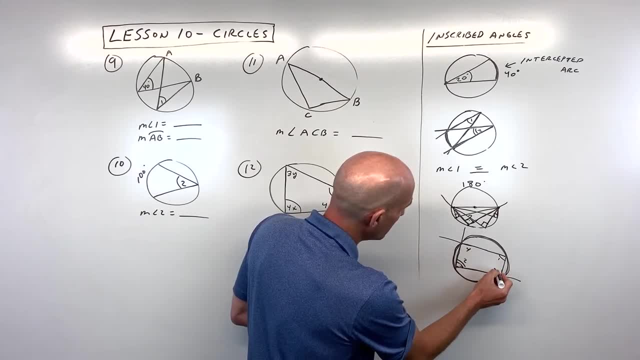 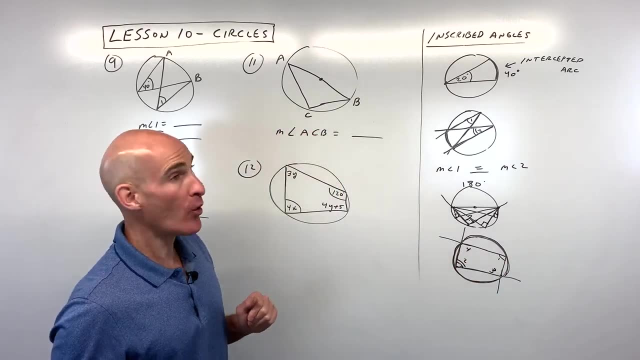 And it's the same thing for angle three and angle four. These two angles are going to be supplementary or they add up to 180.. So opposite angles are supplementary in an inscribed quadrilateral. So let's see if we can do some examples here. 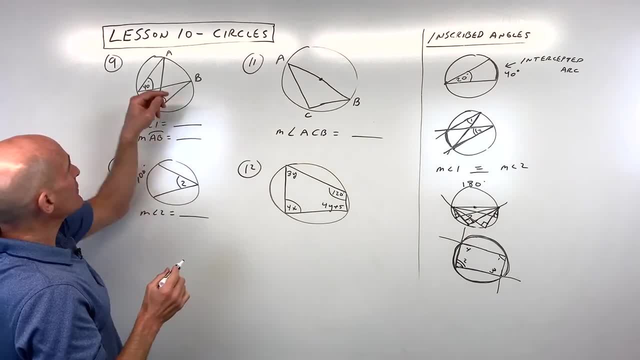 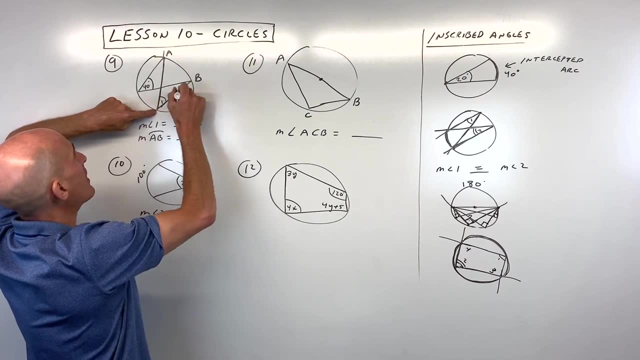 Number nine. it says what's the measure of angle one. So what do you think for this one? It's an inscribed angle. What do you think? Well, notice that angle one intercepts arc AB Over here, this 40-degree angle. 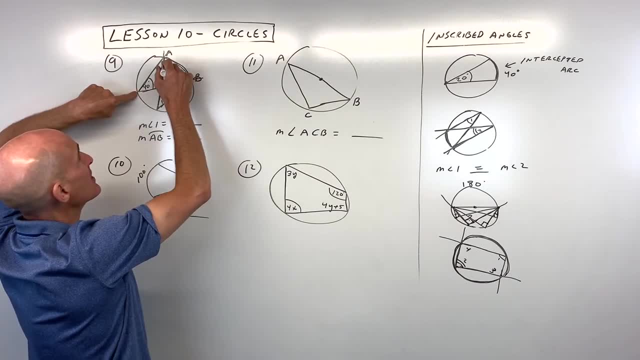 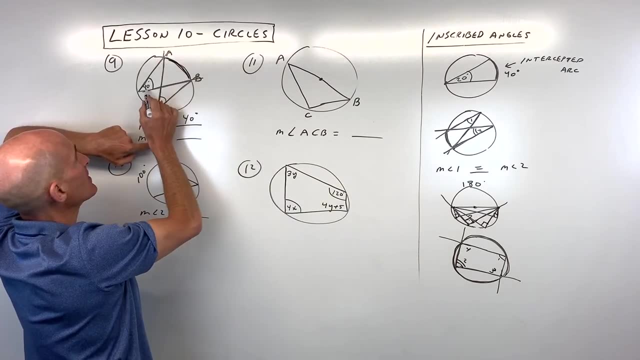 Also intercepts arc AB. Because they're intercepting the same arc, they must be congruent. Now here it says: what's the measure of arc AB? How many degrees? Well, because this is an inscribed angle 40, the intercepted arc is going to be double. 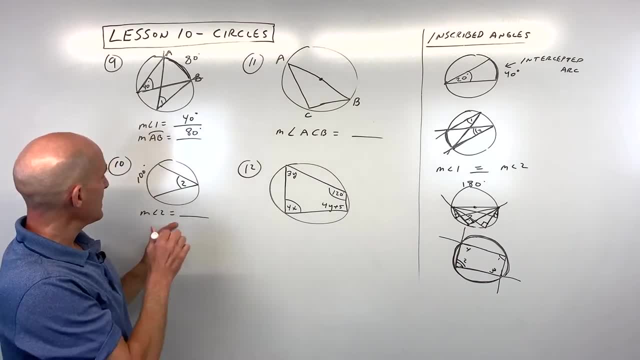 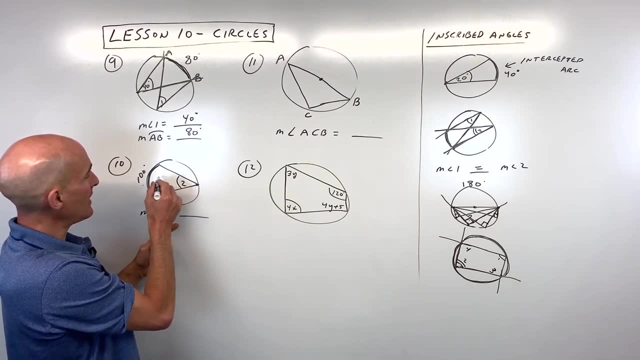 80 degrees. Okay, how about for number 10?? Here they give us the measure of this intercepted arc. It's 100 degrees And you can see angle two is an inscribed angle. It's going to be half of the intercepted arc. 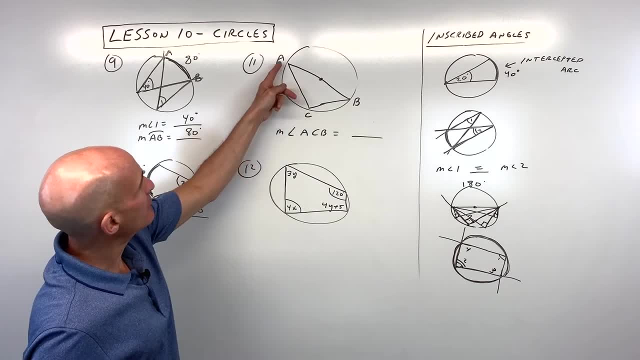 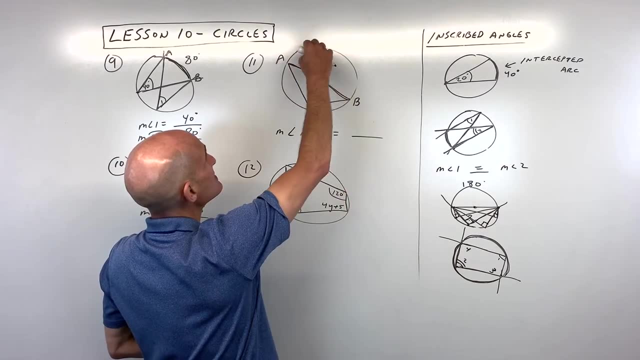 So it would be 50 degrees For number 11,. what do you think for angle ACB? Well, notice that this is a diameter, which means that this is a semicircle, Or you can think of this angle as being inscribed inside of a semicircle. 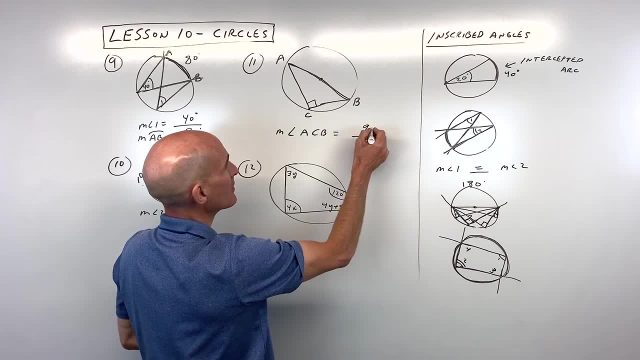 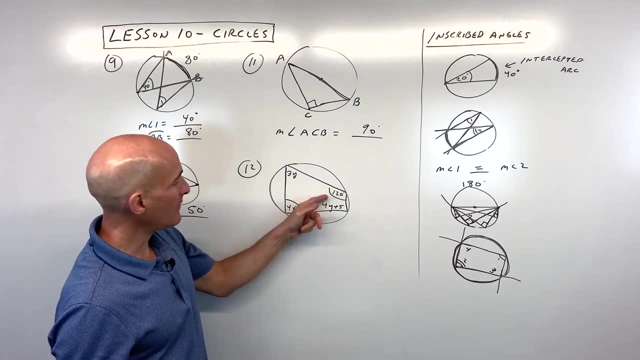 This is going to be a right angle, like we were talking about in this diagram here. So 90 degrees And then for number 12, you can see we have an inscribed quadrilateral. What do we know about the angles that are across from another or opposite angles? 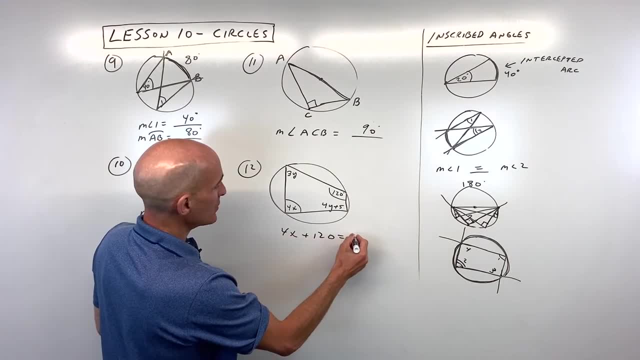 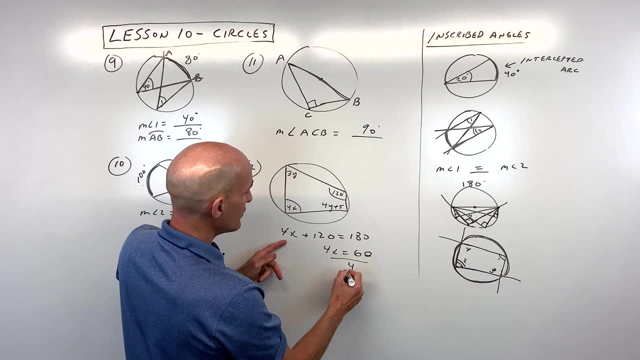 We know that they're supplementary. So 4x plus 120 equals 180.. If we subtract 120 from both sides and divide by 4, you can see that x is equal to 15.. Okay, so that would make this: 60 plus 120 is 180.. 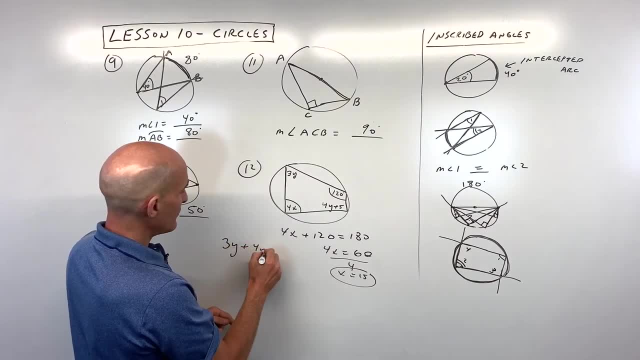 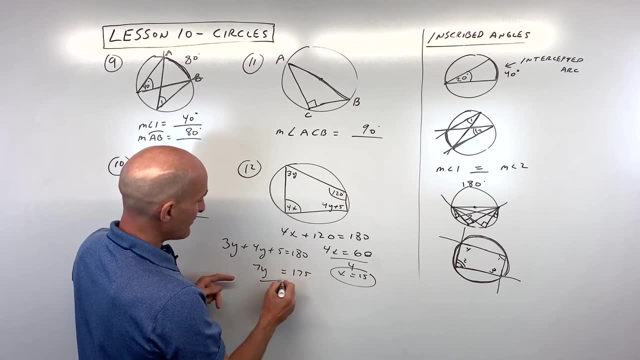 And these opposite angles also have to be supplementary. They have to add up to 180.. So here we've got 7y. subtract 5 from both sides and divide both sides by 7, you can see that y is going to be 180. 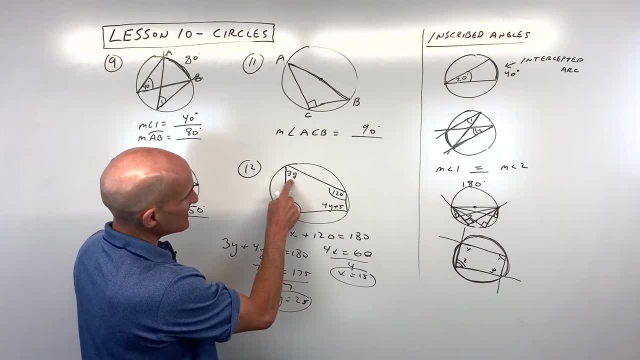 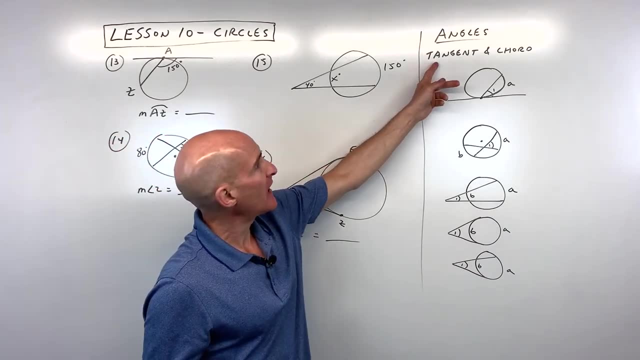 y is coming out to 25, and we can check that that's 75,, that's 105, those add up to 180.. Okay, let's talk a little bit more about angles. The first thing we want to look at here is when we have a tangent and a chord. 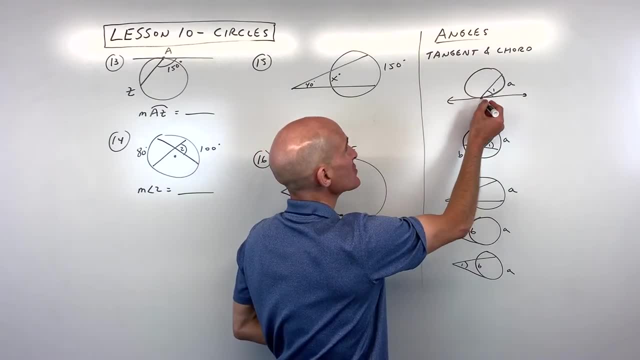 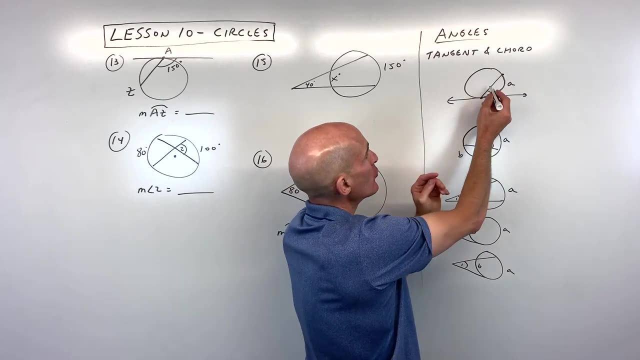 So remember, a tangent is like a line or a segment that just barely touches a circle at one point, And a chord is a segment where both endpoints lie on the circle. But notice what happens here: between this chord and this tangent there's an angle here. 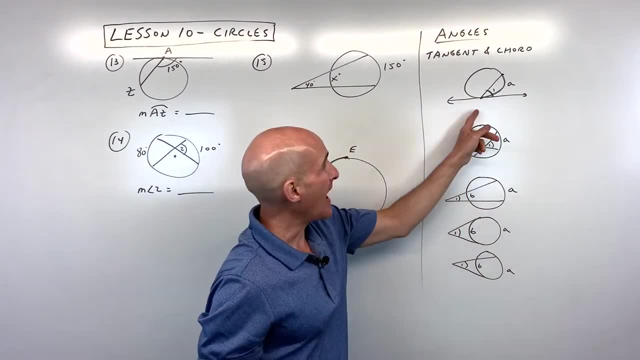 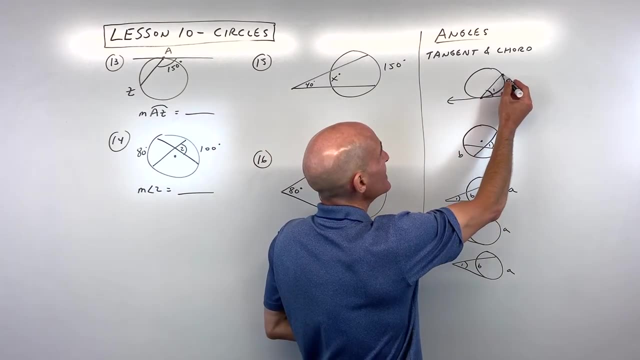 that's formed And that angle. notice the vertex is on the circle, very similar to an inscribed angle that we talked about just recently here, And notice angle 1: here it's intercepting or cutting off this part of the circle. 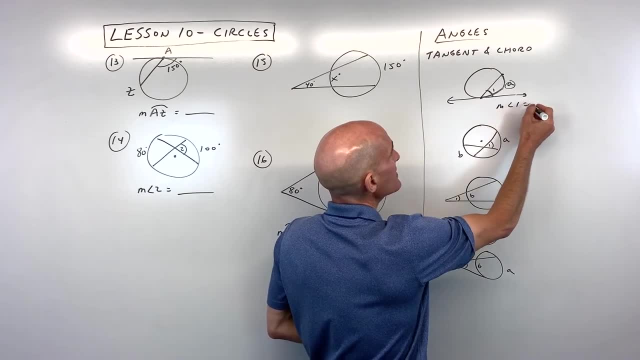 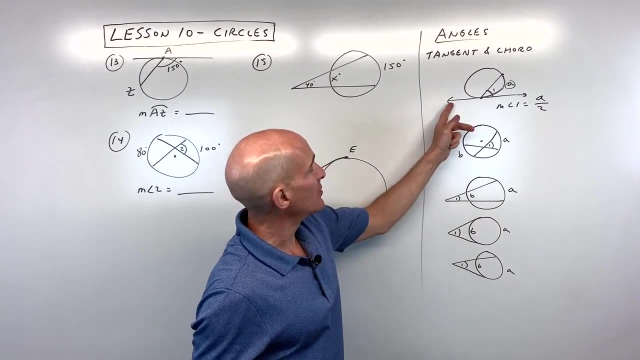 I'm just going to call this a. here The measure of angle 1 is going to be equal to a divided by 2.. It's the arc divided by 2, just like in an inscribed angle. So that's a good formula to memorize there. 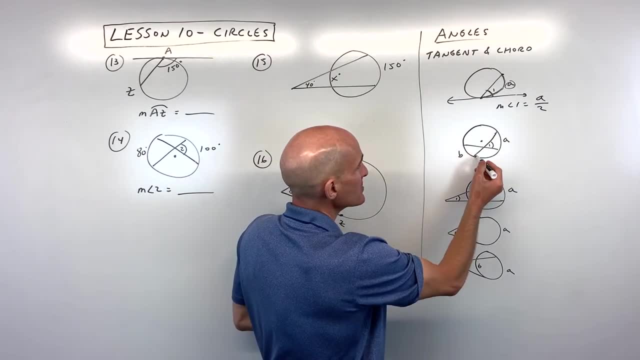 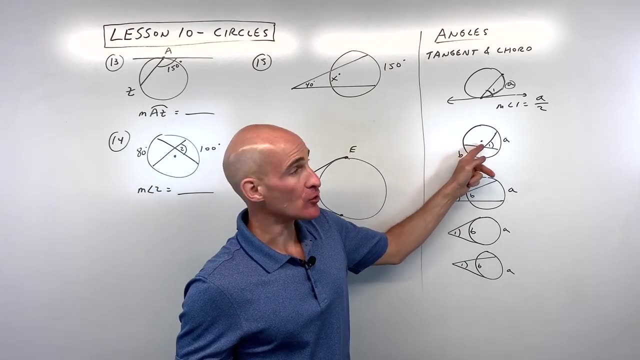 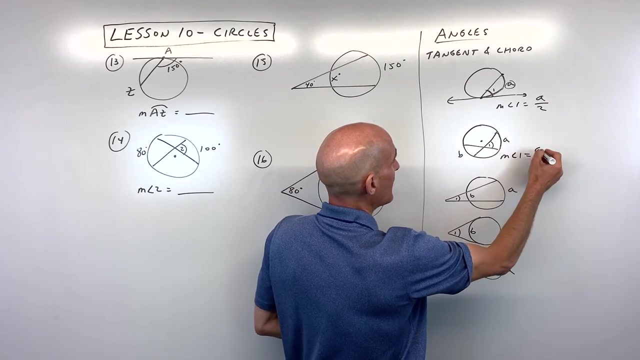 Now, here what we have is two chords that are intersecting. They're intersecting inside of the circle, But notice that where they intersect it's not at the center of the circle, So this is not a central angle. But the measure of angle 1 is equal to this arc A plus this arc B, divided by 2.. 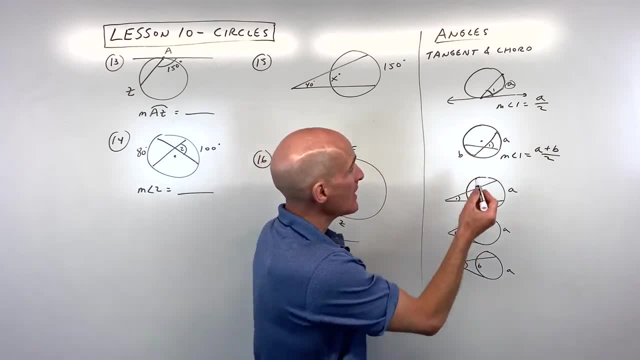 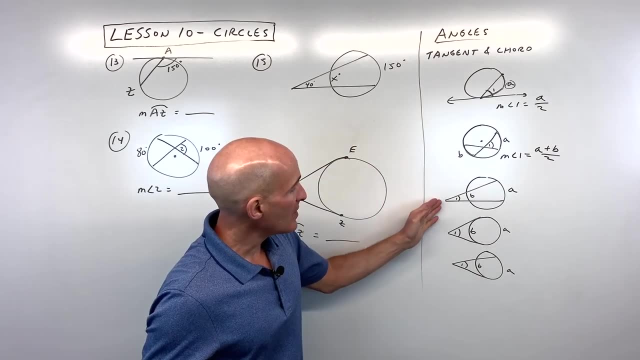 So it's like an average. You're adding up the two intercepted arcs divided by 2.. Now, if you wanted to find this angle here, once you know this angle, you can subtract from 180, because they form a linear pair Over here. now notice what we have. 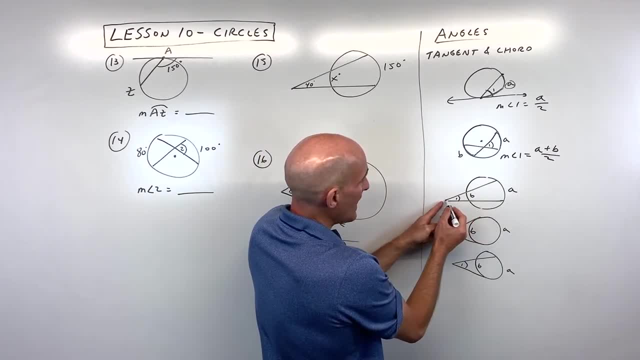 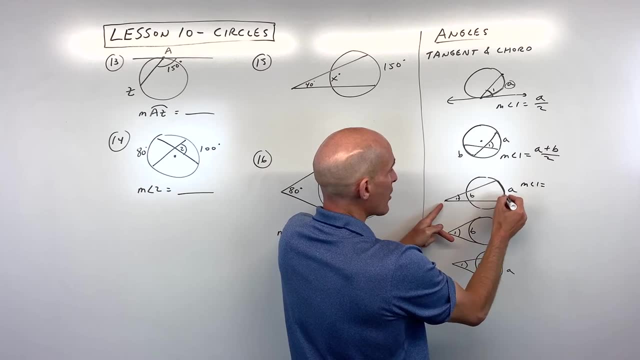 We have 2.. We have 2 secants, But notice the angle that's formed. It's on the outside of the circle. So if we want to find the measure of angle 1, what we do is we take this larger arc A. 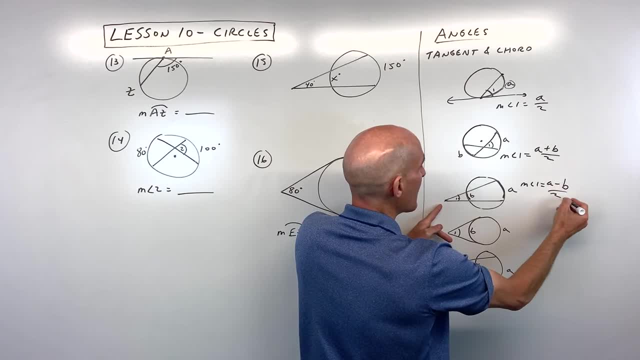 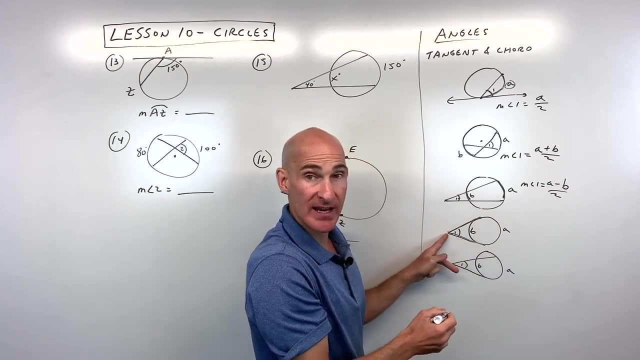 minus this smaller arc here, B, and we divide by 2.. Same thing for this one. here We have 2 tangents. Again, notice the angle that's formed. It's on the outside of the circle. We take this larger arc A minus the smaller arc B, divided by 2.. 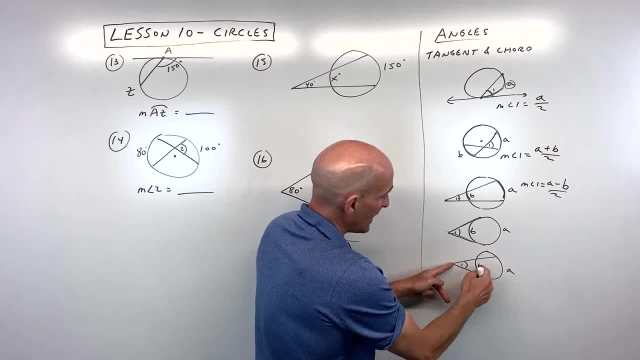 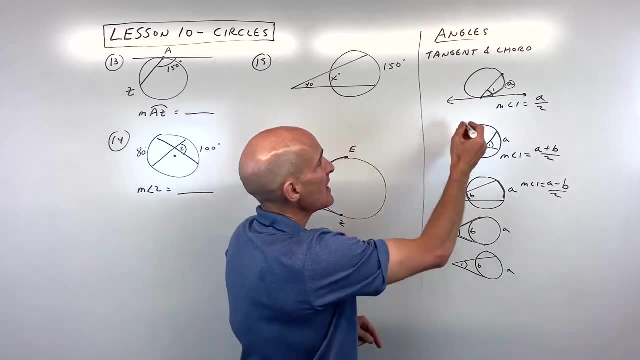 And here we have a secant and a tangent. We take this arc A Minus this arc B, divided by 2. Now it's a lot of formulas, but an easy way to remember it is: look at where the vertex of the angle is. 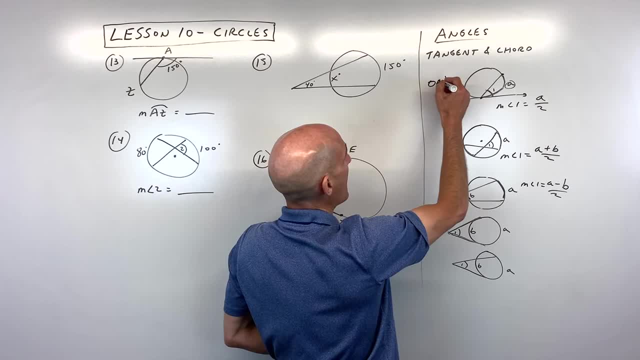 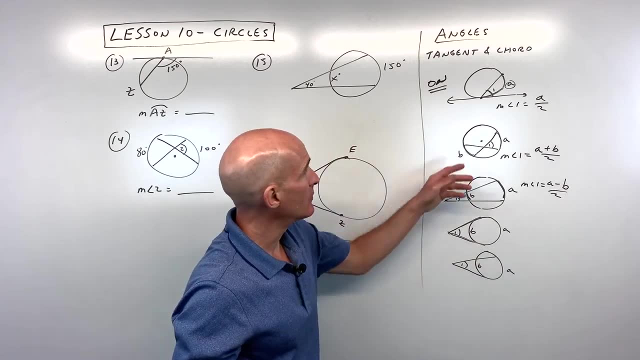 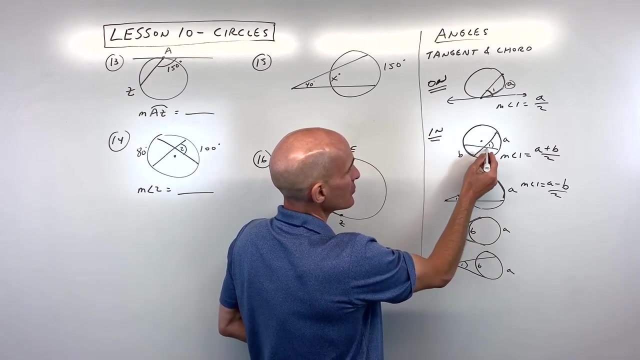 If the vertex is on the circle, so I'm just going to write over here on- then it's just the arc that it intercepts divided by 2, just like an inscribed angle. The vertex is on the circle Here. notice that the vertex of the angle is inside the circle. 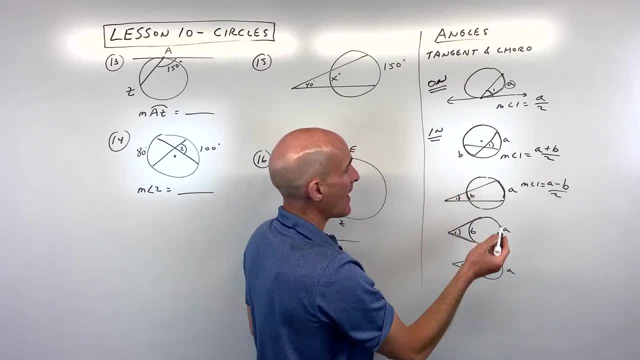 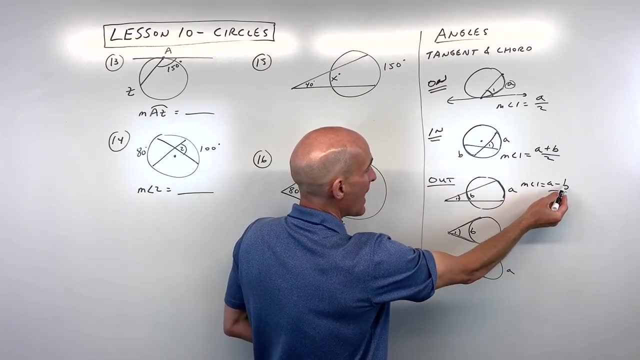 So we add up the two intercepted arcs and we divide it by 2, like an average, And over here notice the angle. the vertex of the angle is on the outside of the circle And what we do is we subtract the intercepted arcs and divide by 2.. 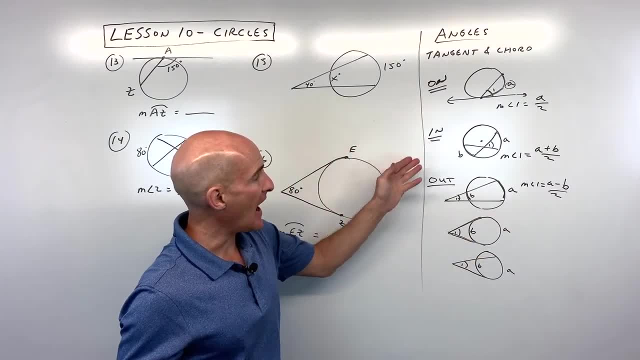 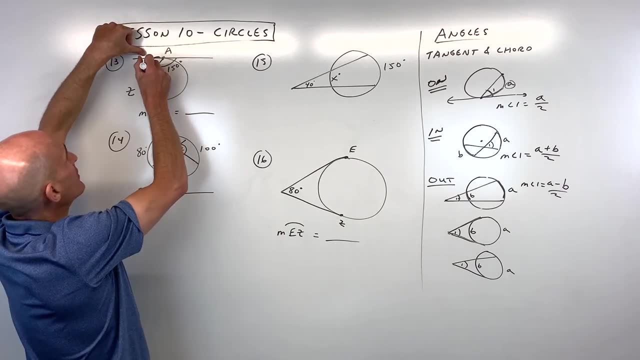 So you really only need to memorize those three formulas and just ask yourself: is it on, in or out? Okay, so let's go over to some examples. So say number 13, we want to find the measure of this arc, AZ, right here. 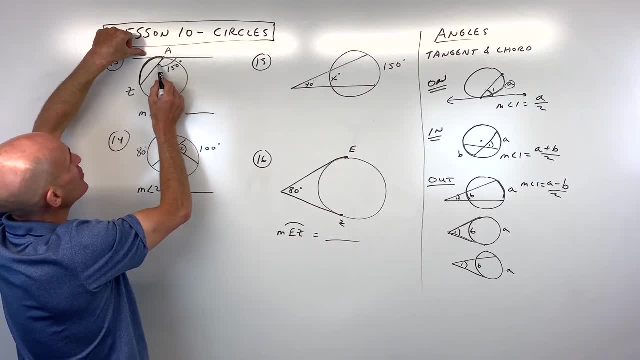 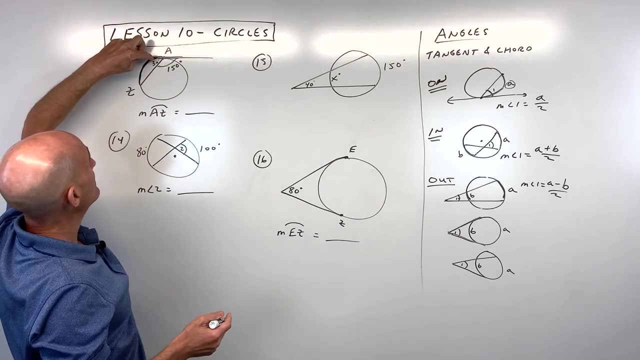 Well, there's a couple different ways we can do this. but if this angle here is 150, then we know that this angle here is 30, because they form a linear pair, A straight line. If this is 30,, the intercepted arc is double. 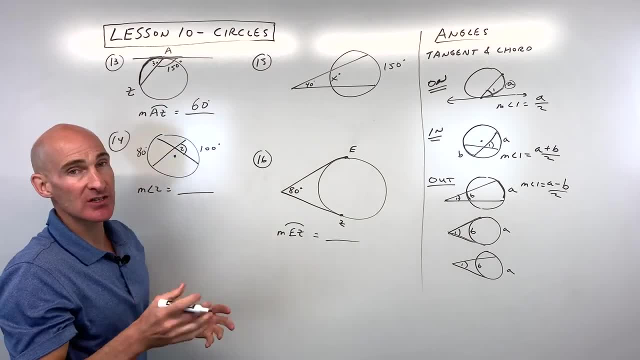 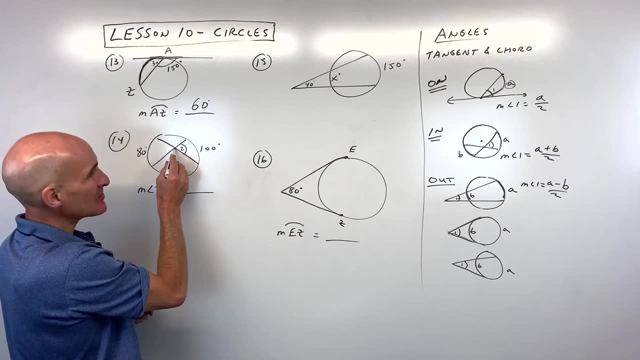 It's going to be 60. Or if this was 60,, half of 60 is 30. So either way For number 14, what do you think for this one? We've got two chords that intersect inside the circle. 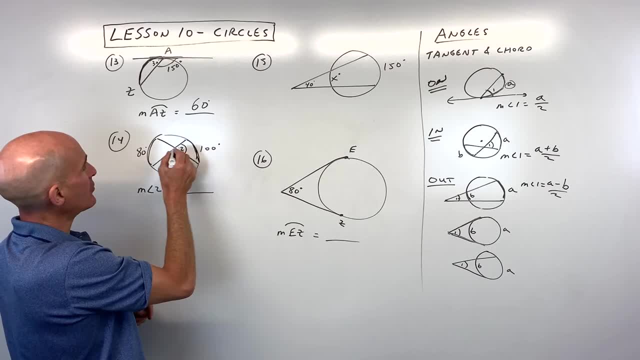 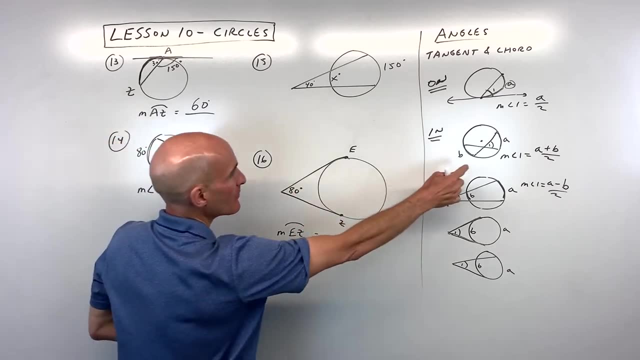 They're chords here. they're going to intercept these two arcs. 180, right. 100 plus 80 is 180, divided by 2 is 90. Remember, it's an average. You're adding up the two arcs and dividing by 2.. 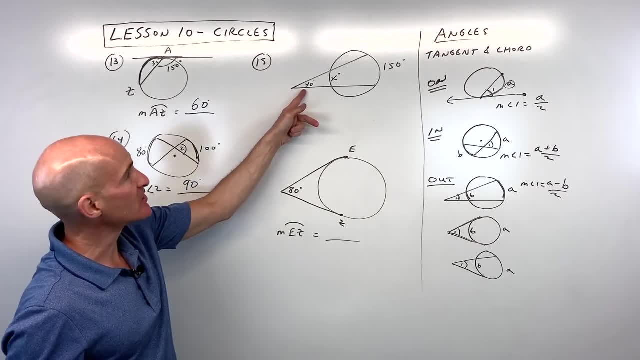 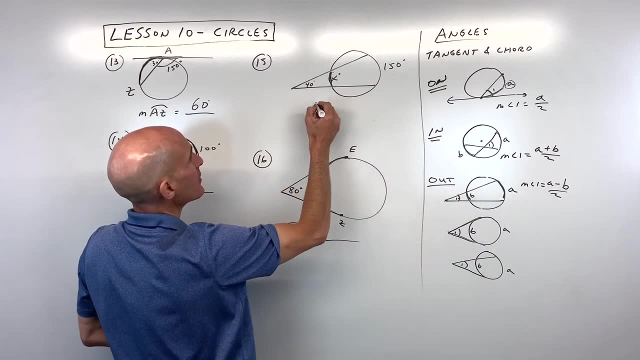 For number 15, notice this angle is on the outside of the circle, but we're trying to solve for this arc now. So what we can do is we can use our formula when it's on the outside. we can say: take the larger arc minus the smaller arc divided by 2, and that equals the measure of the angle. 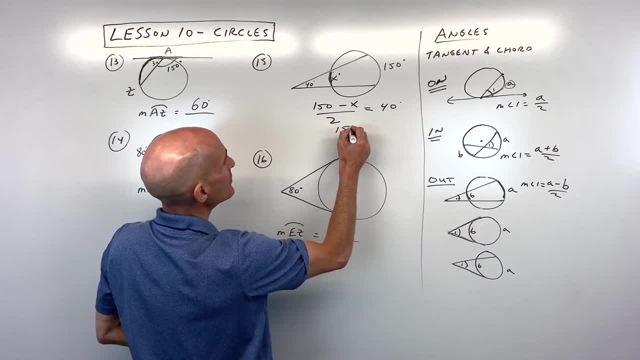 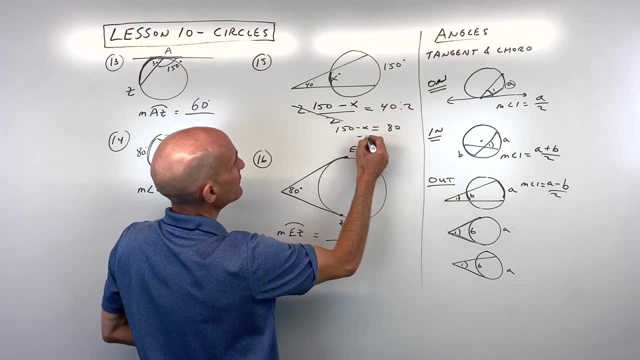 on the outside of the circle. If we multiply both sides by 2, we get 150 minus x equals 80.. If I subtract 150 from both sides, I get negative 70.. And if I divide both sides by 2, I get negative 70. 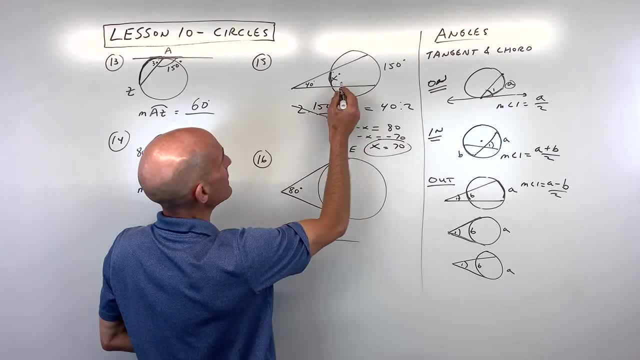 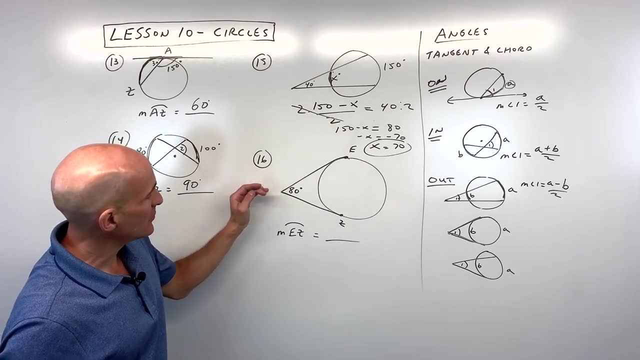 And if I divide both sides by negative 1, I get: x is equal to 70.. You can check your work: 150 minus 70 is 80, 80 divided by 2 is 40.. And for number 16, this one's a little bit tougher. 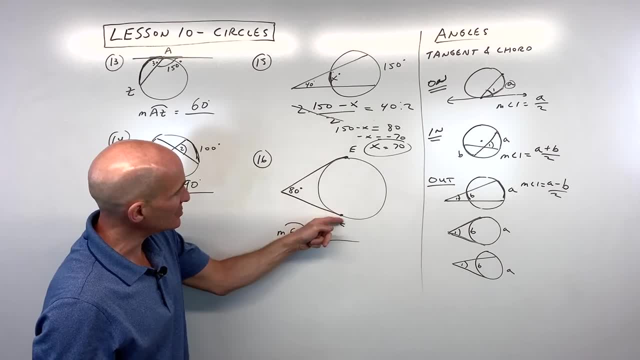 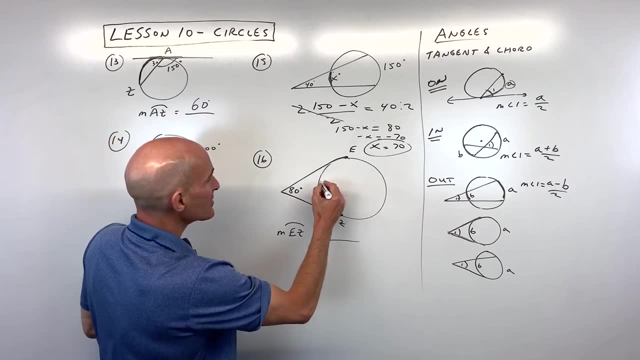 Here they give us the angle on the outside of the circle. These are two tangents. We want to find the measure of this arc right here. ez okay, ez right. So let's just call this arc x. How much do you think this arc would be over here? 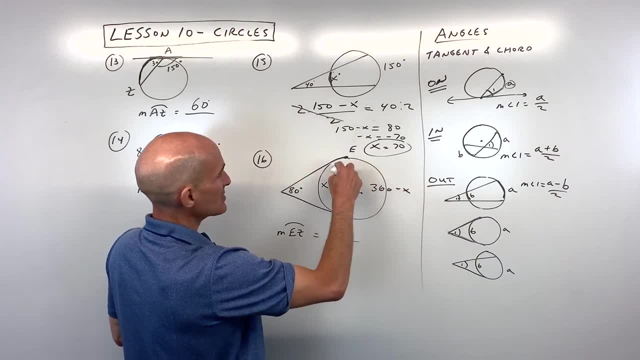 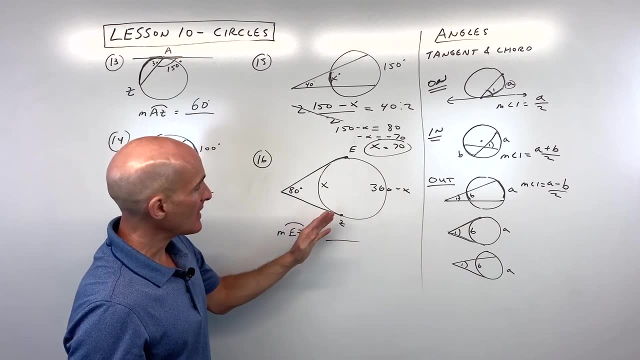 Well, this is going to be 360 minus x. Two arcs have to add up to 360.. If this was 100, this would be 260, right, It's 360 minus 100.. Okay now, because this angle's on the outside of the circle, we want to use this formula. 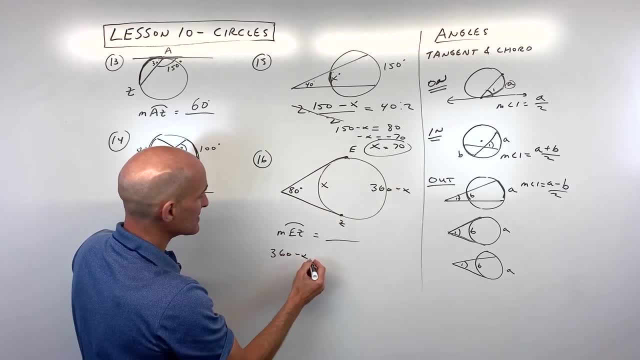 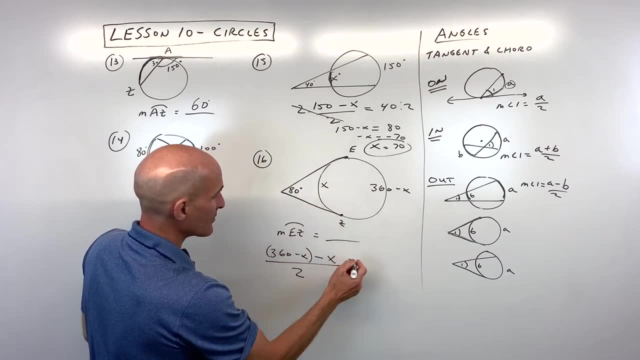 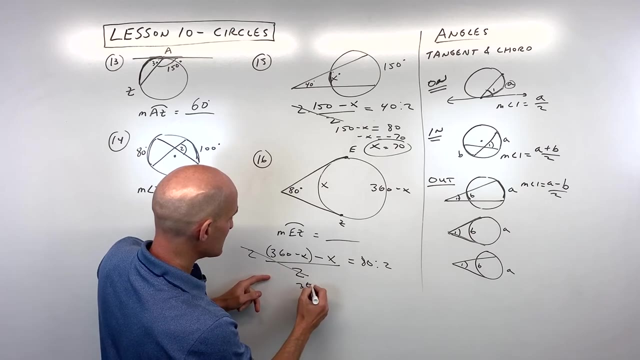 here We're going to take the larger arc, which is 360 minus x, minus the smaller arc, which is x, divided by 2, equals the angle on the outside of the circle here, 80 degrees. If we multiply both sides by 2, to get rid of the fraction here, we get 360 minus x. 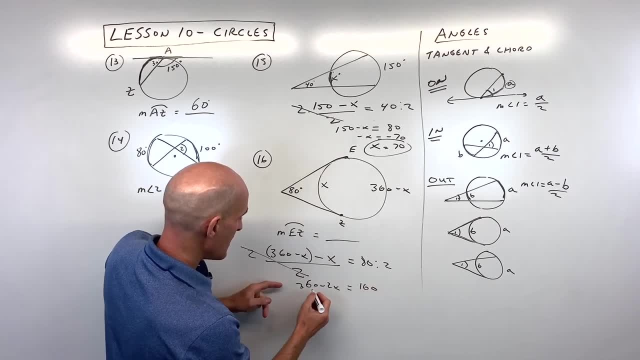 minus x, that's minus 2x equals 160.. If we subtract 360 from both sides, we get negative 200.. If we divide by negative 2, we get x is equal to 100.. So ez, the measure of our ez, is 100 degrees. 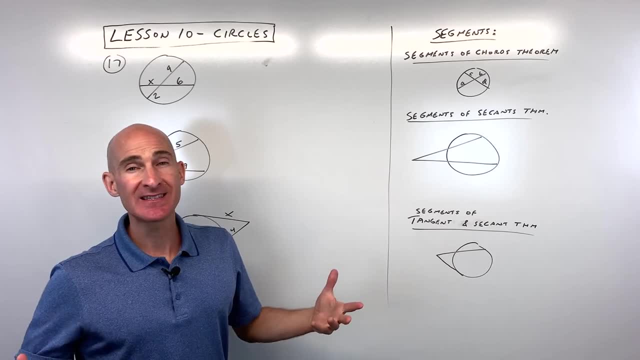 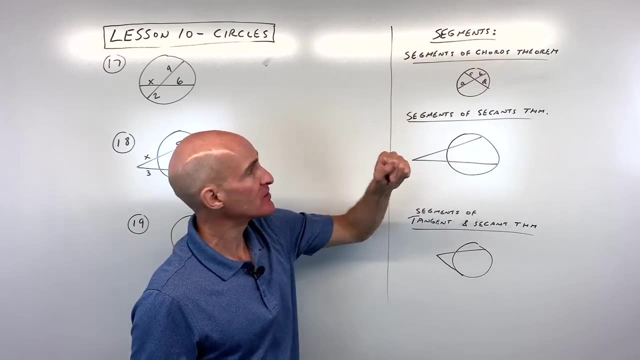 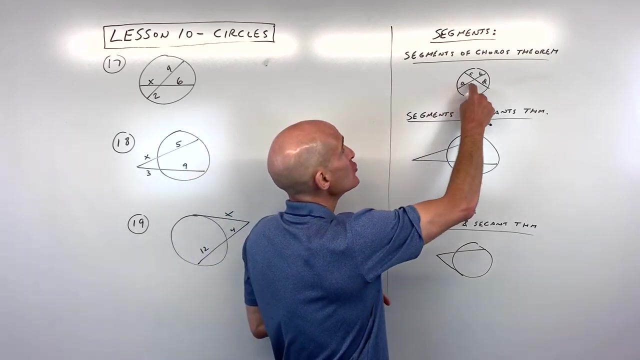 Okay, now let's talk about some theorems involving the segment lengths in circles. So the first one is the segments of chords theorem, and so the way this works is say you have two chords, Okay, They intersect one another, They cut each other into two pieces or two segments, and they don't necessarily have 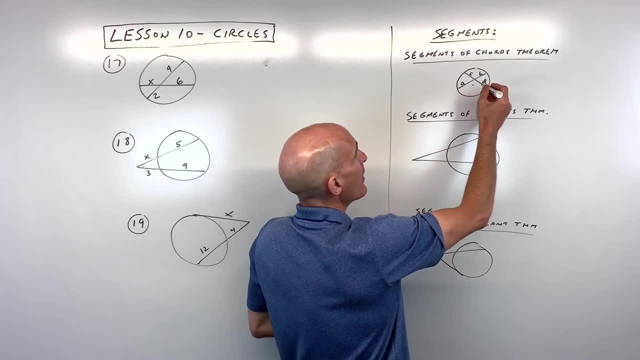 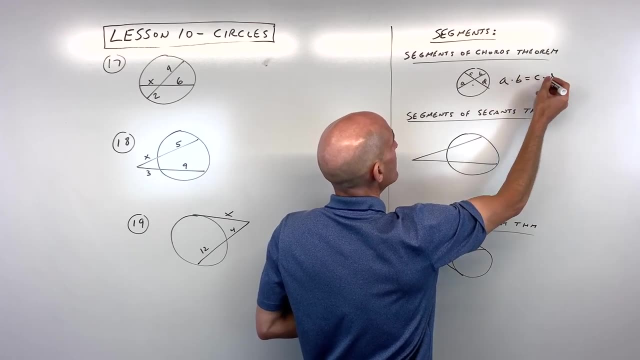 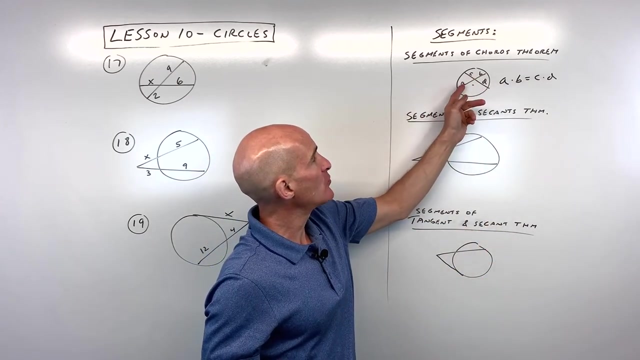 to cross at the center, Like, for example, here. the center could be here. but what happens when they cross and intersect one another, divide each other into two segments. the product of a times b equals c times d, So very easy to remember. they just break each other up into two parts. you multiply. 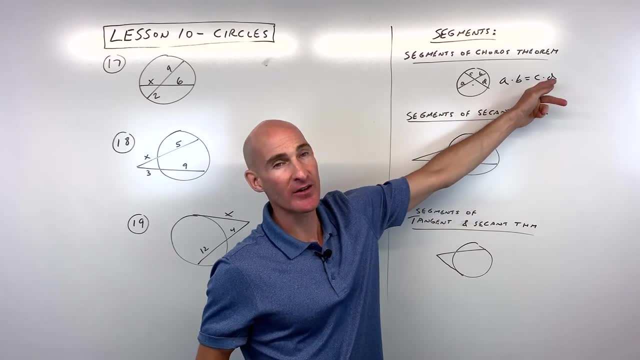 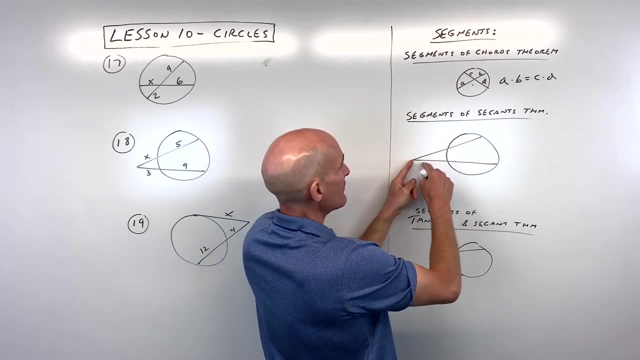 the two parts together, it equals the product of the other two parts multiplied together. Okay, So how about the segments of secants theorem? Okay, so, this one's a little bit interesting. you've got a secant, you have another secant. 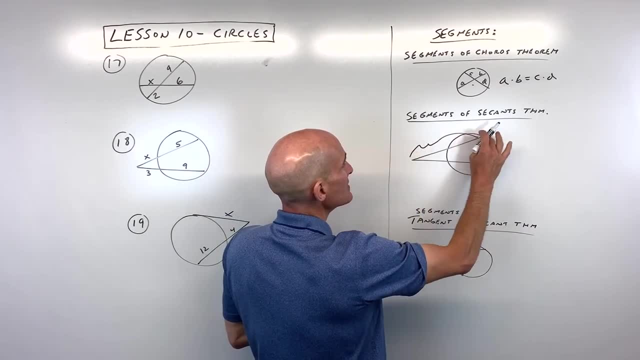 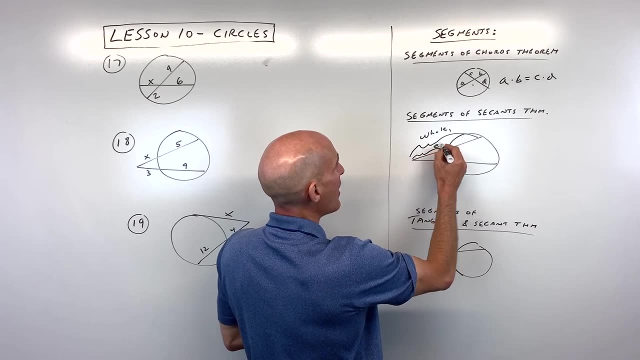 What's the relationship here? Well, if you take this whole secant length- I'm just going to call it whole 1, and you multiply it by the part of the secant that's on the outside of the circle I'm going to 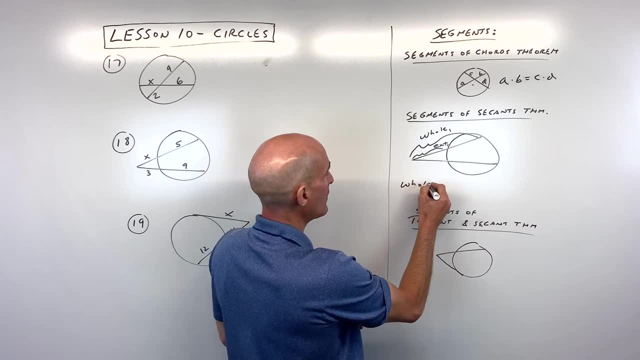 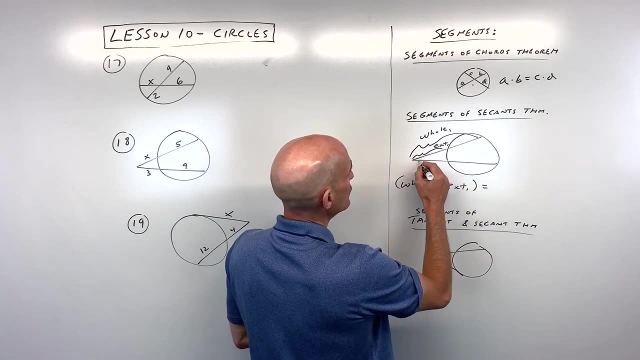 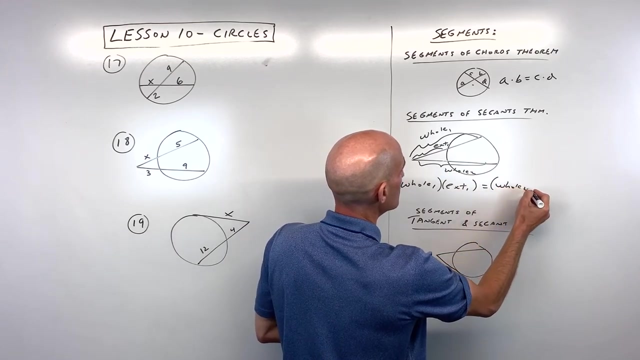 call that exterior 1.. Okay, so we have the whole length of secant 1 times the part exterior to the circle. I'll call it exterior 1.. Okay, So the product is equal to the whole length of secant number 2 times the exterior part. 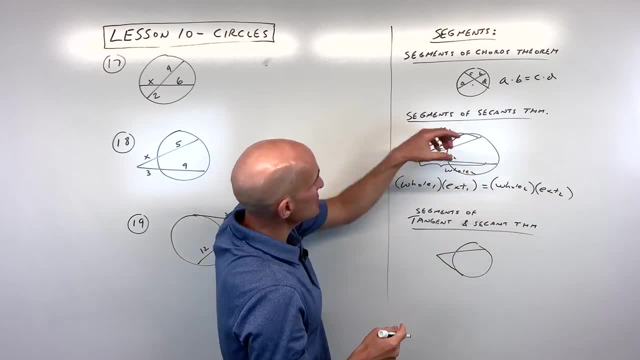 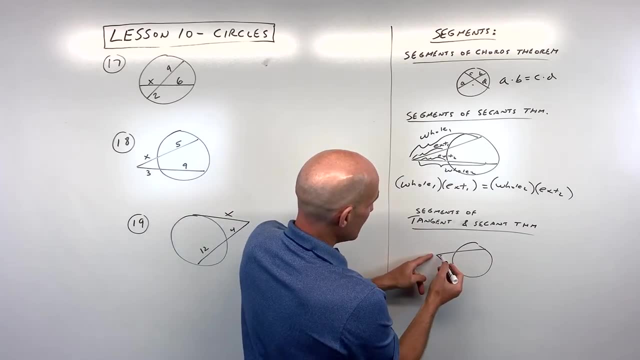 of secant number 2.. So pretty easy. just whole times exterior equals whole times exterior. Now what happens if you have a secant and a tangent? so this is called the segments of tangent and secant theorem. Well, what you do? it's very similar to this one. 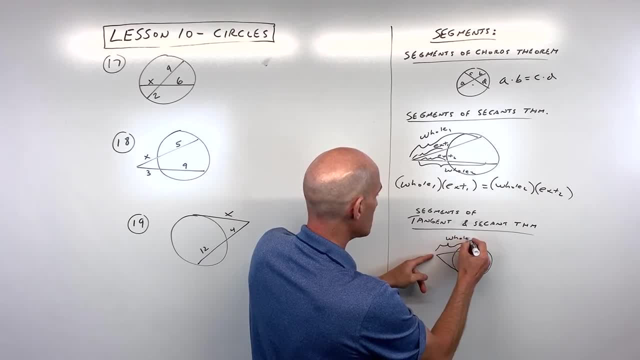 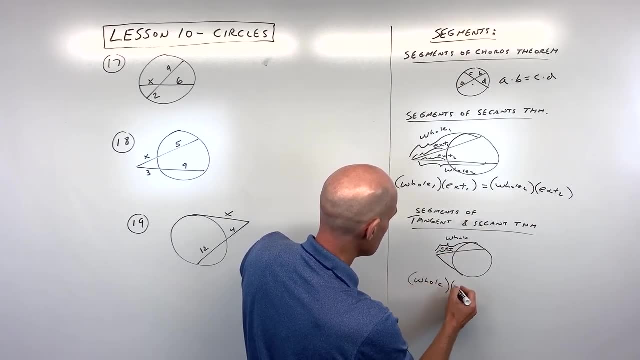 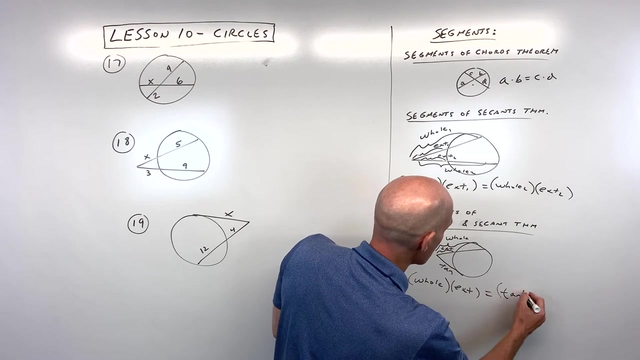 You take the whole secant length. I'm just going to write whole the part that's outside the circle. we'll call that exterior. so we have whole secant length times the exterior part of the secant equals the tangent. okay, this tangent length squared. 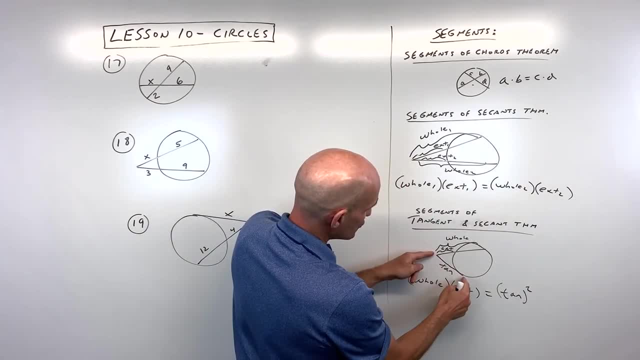 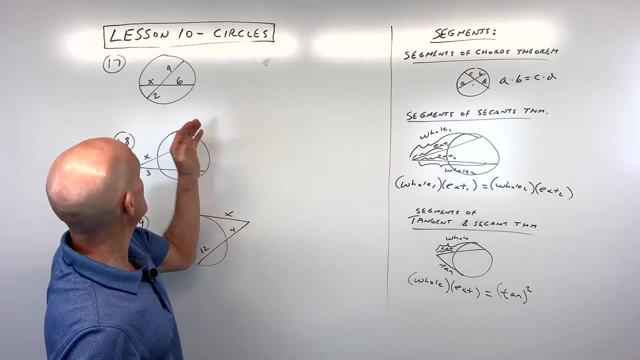 So you can kind of think of it as like the whole length and the external part they're the same, so it's like whole times. external is really like tangent times tangent or tangent squared. So let's look at a few examples here. Number 17, you can see we have a circle, we have two chords that intersect, and how 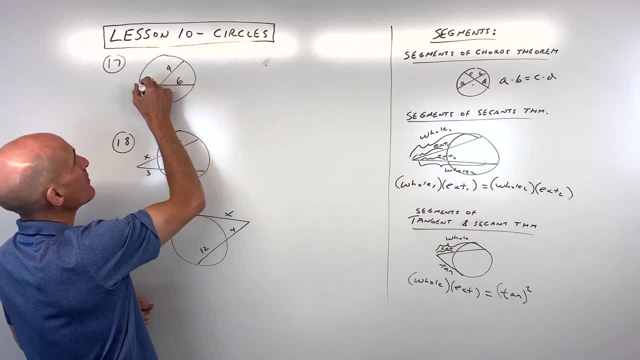 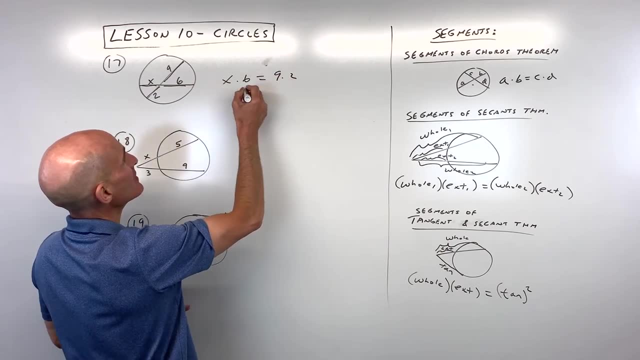 do we solve for this missing segment length here? x? Well, remember, x times 6 is equal to 9 times 2.. So pretty easy, right? So we have: 6x equals 18, divide both sides by 6,, x is equal to 3.. 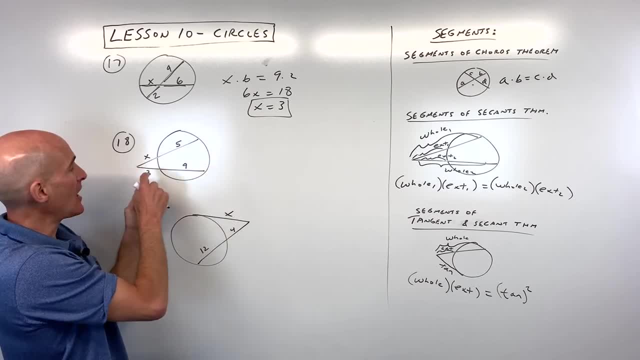 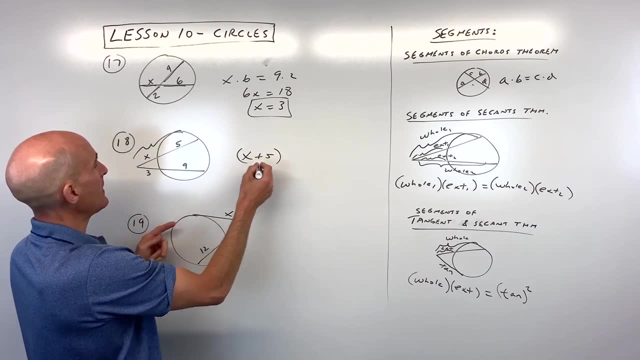 For number 18, you can see we have two secants. okay, so how do we find this exterior part here? x? Well, remember, it's this whole length. sometimes people make a little bit of a mistake with this. they say you know 5 times x, or 5, or x, you really have to add these together. 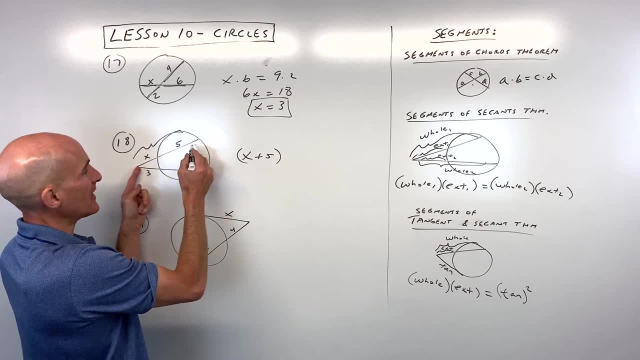 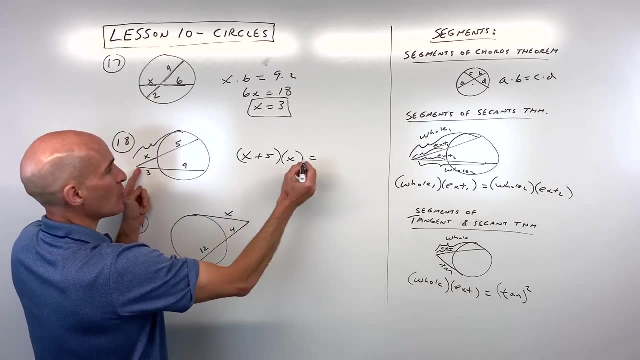 to get the whole length, x plus 5,, so that's the whole secant length times the exterior portion, which is x, equals this whole length. so 3 plus 9,, which is 12, times the exterior part of this secant, which is 3.. 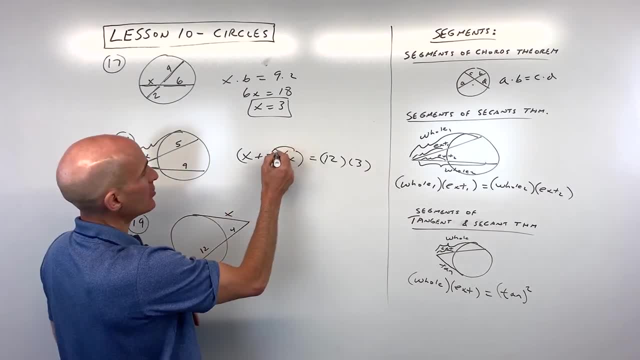 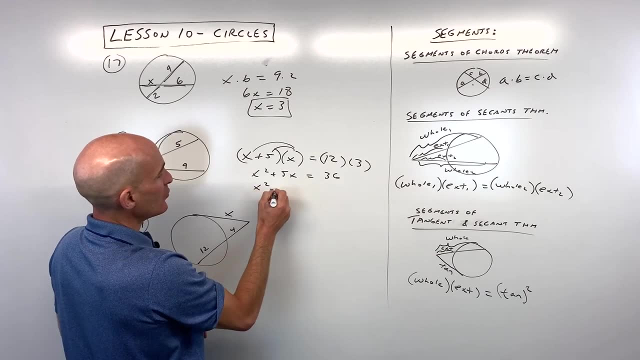 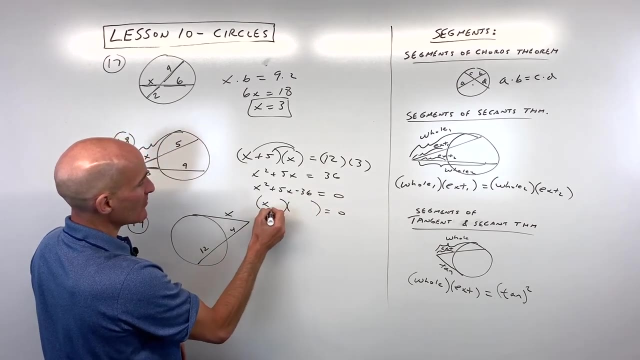 So just remember: whole times external equals whole times external. if we distribute, we have x squared. So we have x squared plus 5x equals 36, subtract 36 from both sides, so now it's equal to 0, and we can factor this. so this is kind of from algebra, right? so remember your algebra. 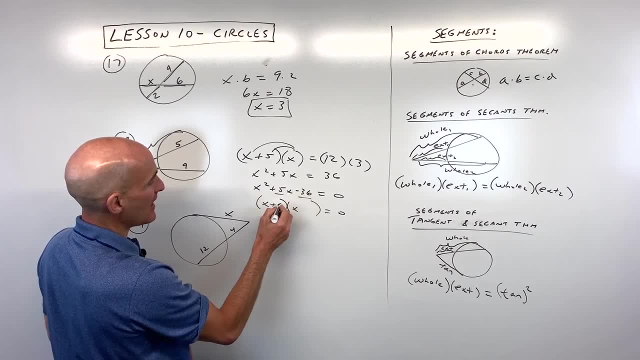 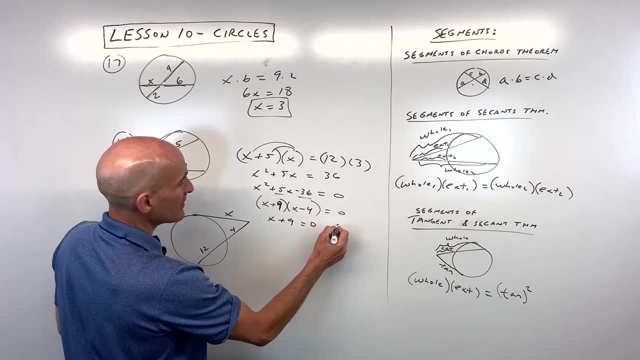 skills. what multiplies to negative 36 but adds to positive 5? That's going to be positive 9 and negative 4.. So if we set each of these factors equal to 0, that's our 0 product property- we get x. 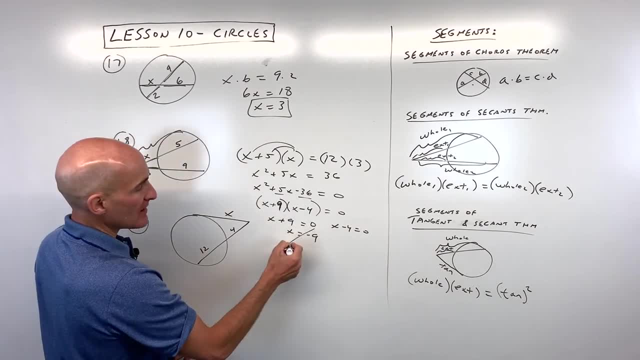 equals negative 9,. can x be a negative length? No, That doesn't matter, that's 12 plus 4, that makes sense. If we add 4 to both sides, x equals 4, yeah, that makes a little bit more sense. 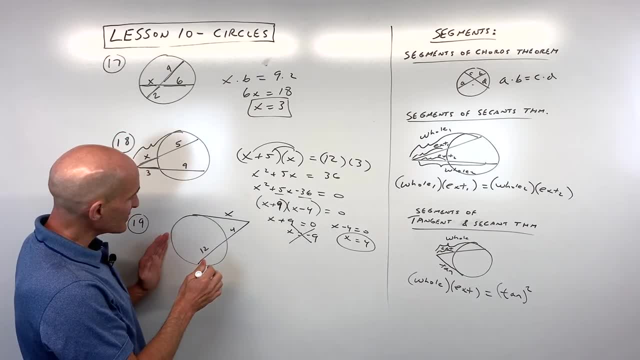 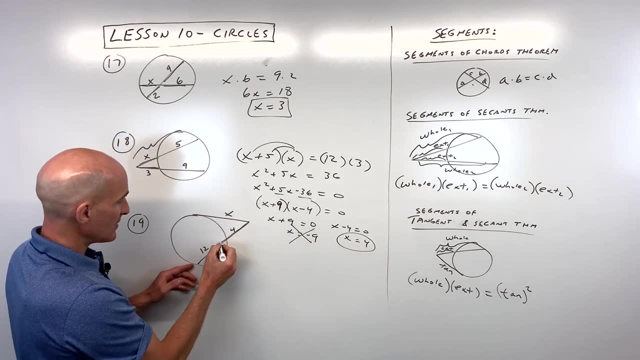 Okay, and then the last one, number 19. here, for this part, we've got a secant and we have a tangent. So what do we do when we have a secant and a tangent? Well, we take that whole secant length, which is 12 plus 4, that's 16, times the exterior. 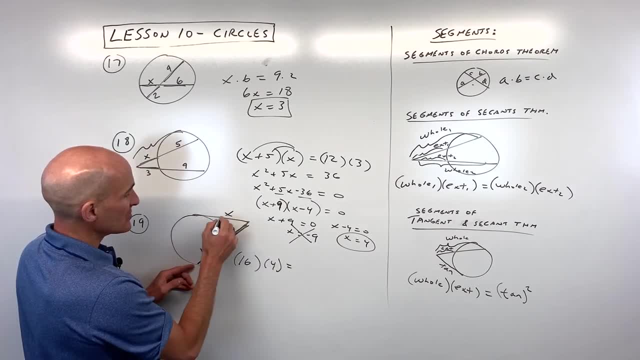 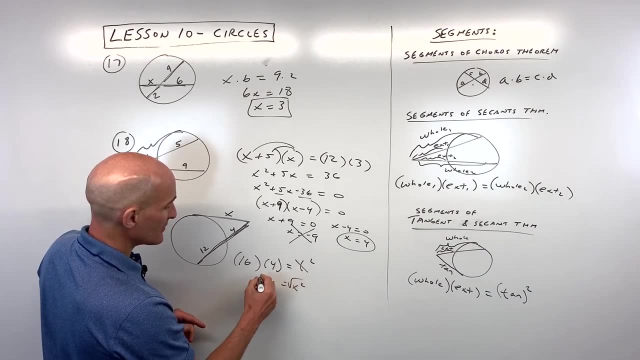 part. that's 4, equals the tangent squared, so that's x squared. So this comes out to 64, equals x squared. If we take that to the right, that makes sense. If we take the square root of both sides, you can see that x is coming out to 8, and 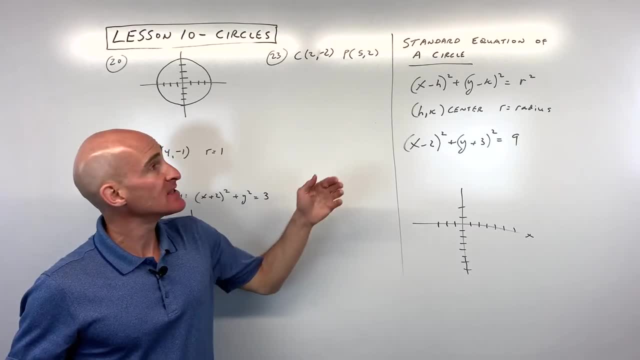 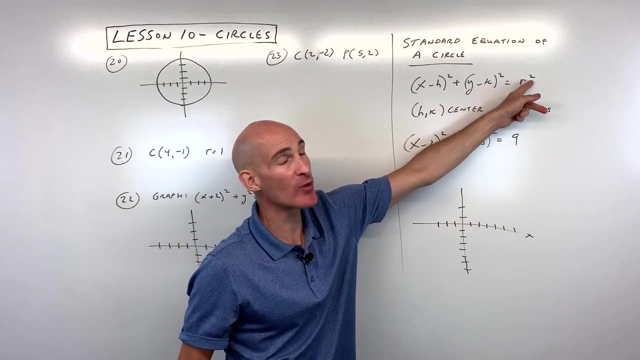 you got it, Okay. the last thing that we want to talk about in this lesson is the standard equation of a circle, and it's this here: x minus h, the quantity squared plus y minus k. the quantity squared equals the radius. 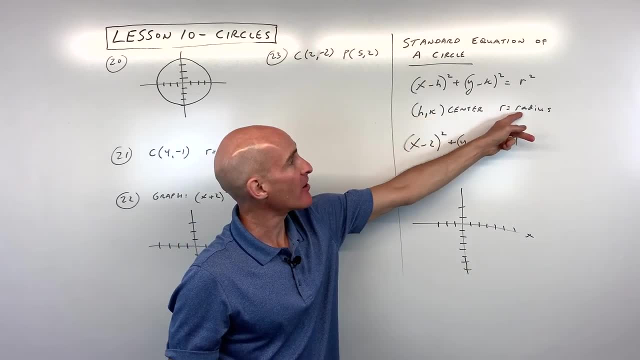 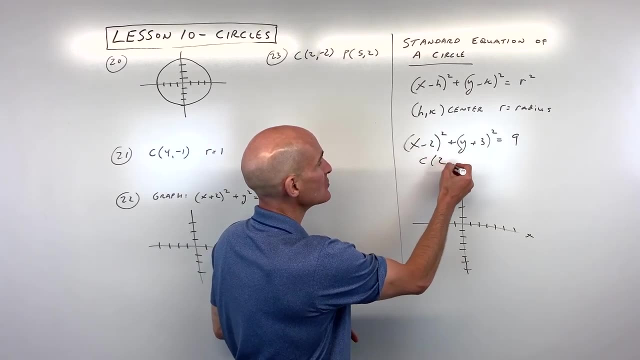 squared where h comma k is the center and r is the radius. So a quick example: if we're given this equation here, you can see that the center is going to be at positive 2, negative 3, it's going to be the opposite, see x minus h. so it's: 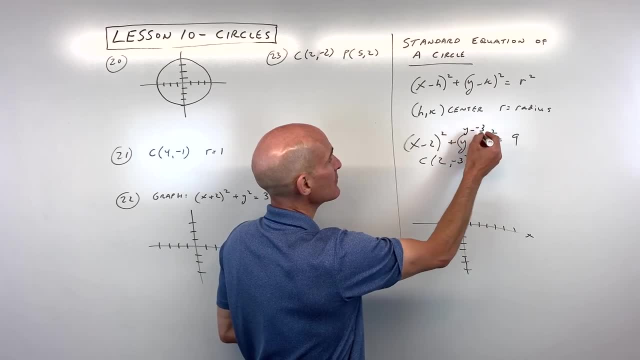 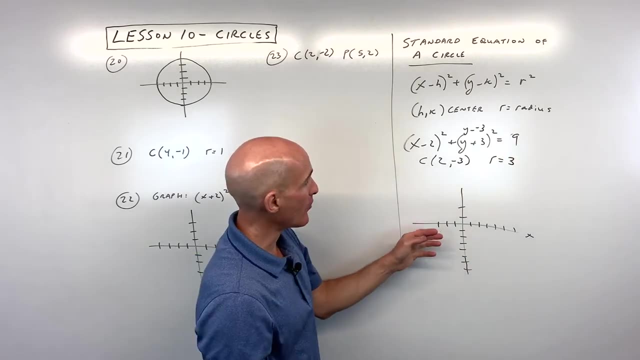 actually positive 2.. This is really like y minus negative 3, so they're always the opposite. And this because it's the radius squared is 9, if we take the square root, the radius is 3.. Now, if we graph it, the center is going to be at 2, negative 3.. 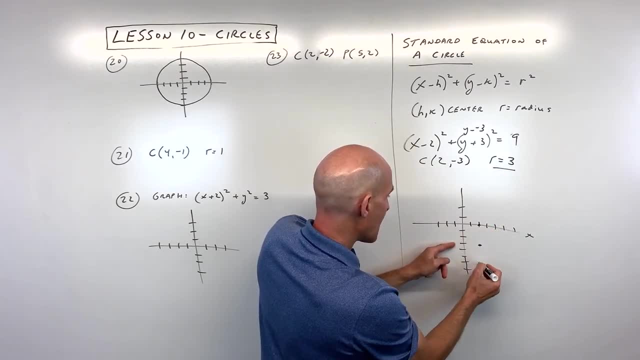 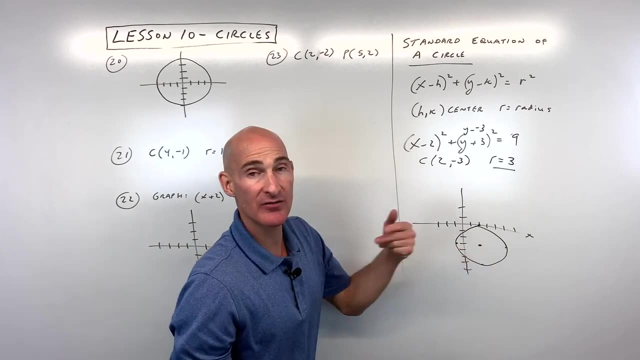 Because the radius is 3, we can go up 3, down 3, right 3, and left 3.. That kind of gives us some easy points on our circle, The graph, and you've got your circle. So for number 20, now they're giving us the circle. we want to find the equation. 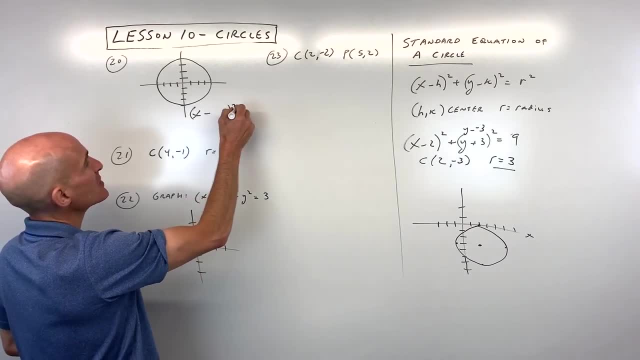 So if we start off with our equation of our circle, x minus h squared plus y minus k squared equals the radius squared. here you can see the center is right at the origin, so it's 0, 0, and the radius is 4, so 4 squared is 16.. 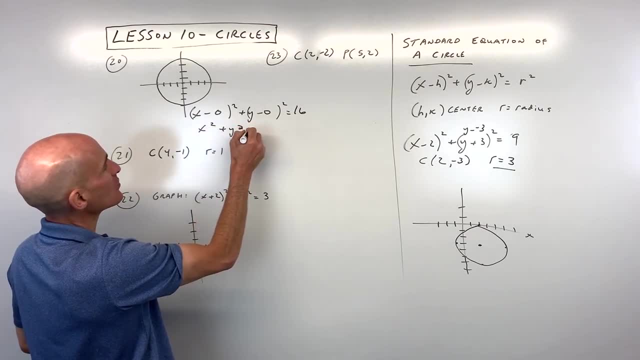 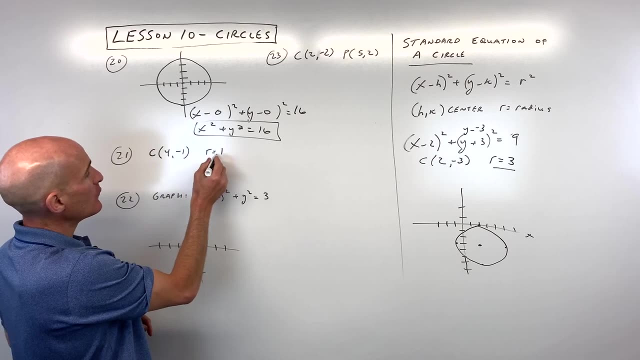 Of course you can simplify this just to: x squared plus y squared equals 16, and you got it For 21,. we want to write this. We want to write the equation of a circle with center at 4, negative 1, and radius 1.. 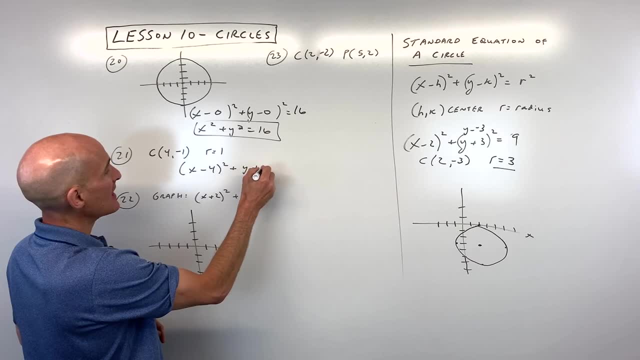 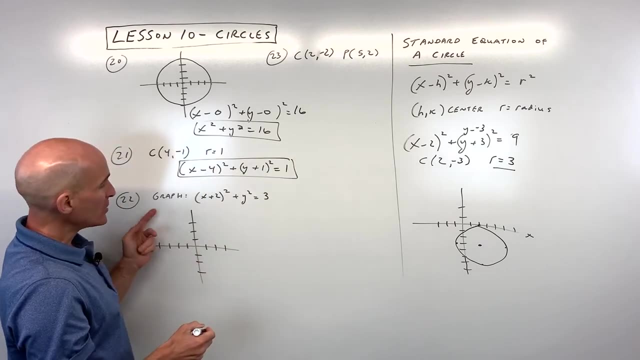 So it would be x minus 4 squared plus y minus negative 1, which is y plus 1 squared, and the radius 1 squared 1 times 1 is just 1.. For 22, we want to graph this circle. 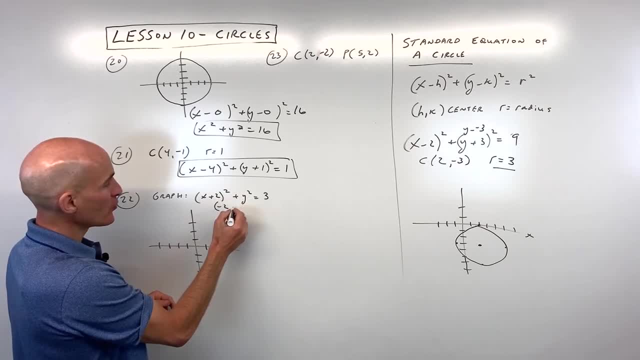 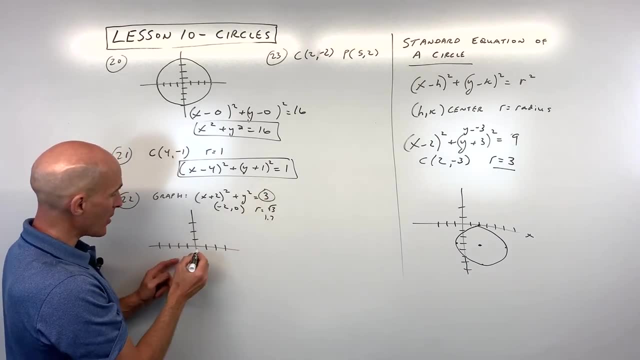 It looks like the center is at negative 2.. This one, there's nothing grouped with y, that's just going to be 0, and the radius is actually the square root of 3, which is about 1.7.. Remember, this is r squared. 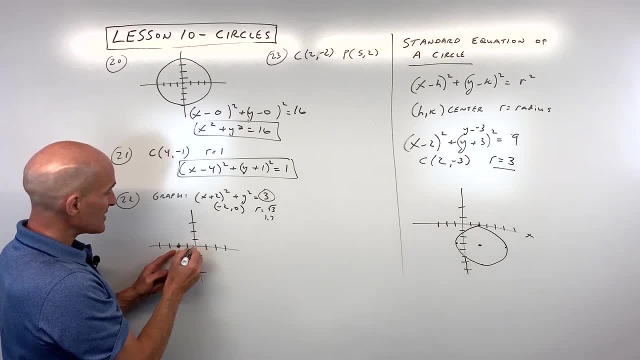 So negative 2, 0.. We're going to go right- 1.7, left, 1.7, up 1.7, down 1.7, approximately, to get a good sketch of our circle. And the last one, the center of the circle, is at 2, negative 2, and it passes through. 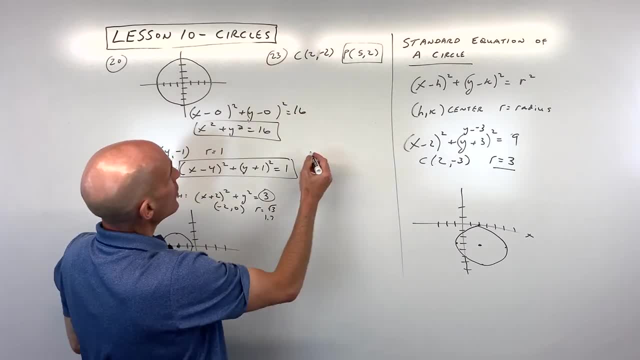 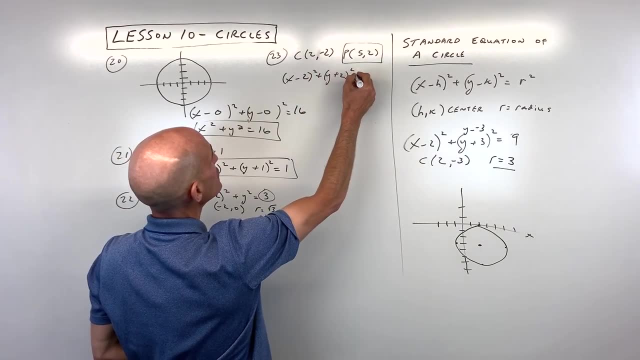 this point, 5, 2.. What's the equation of the circle? Well, let's see. We've got x minus 2, the quantity squared plus y plus 2, the quantity squared equals r squared. We don't know the radius.